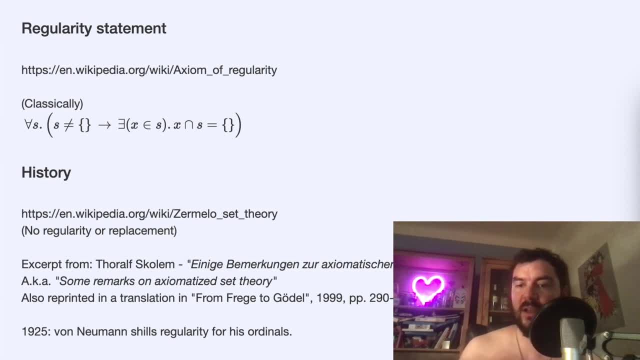 So I will restrict myself to the spicy topic of weak arithmetics- And If you are just here for the formal explanations, then you can now skip ahead for probably about five minutes or so. but I will want to give some, some context and some explanation to to what extent this is like philosophically also interesting, and not just the math. 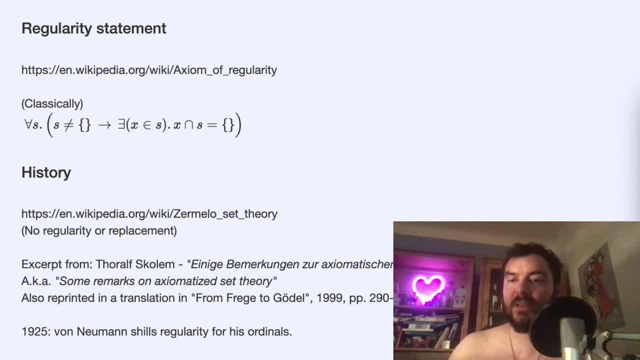 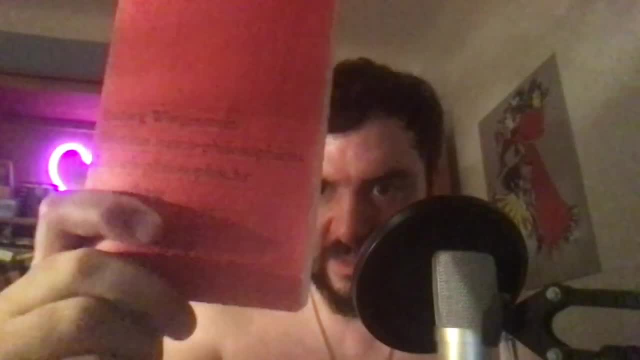 So there are timestamps below. You can jump ahead. Otherwise I'm quickly going to talk about Tony coming out. And anyway, thank you for watching and have a great weekend. Bye, Bye. See you at nice, nice, nice, like like. bye, bye. Bye, bye. J B C, D Z, M, J B, A, C, C E, A, J S, A, P, C, D S, S A E W. 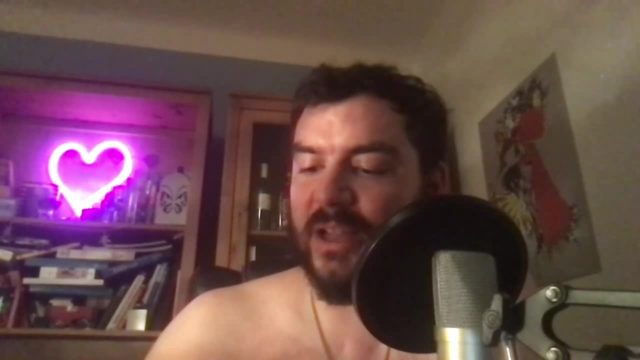 J M R S B. That's all because I want to show how you can use that concept as a way to� the The young Wittgenstein working with and J Russell and good colleagues with Ramsey. he had this perspective, that, only that. 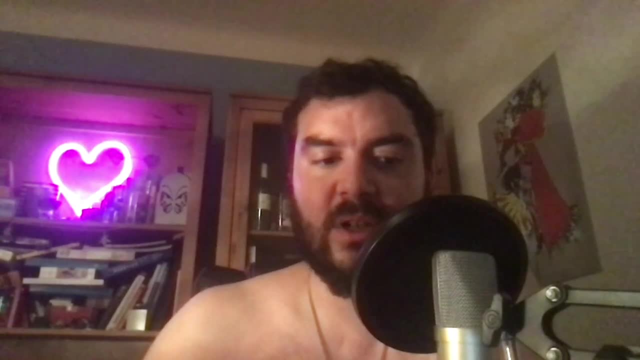 which can be really properly formalized in a consistent fashion. yes, it's really like it's really possible to make sensible statements about it, and the sentence I just quoted is basically saying: you know, everything else is you know. this is just really gibberish and every philosophy before that talking. 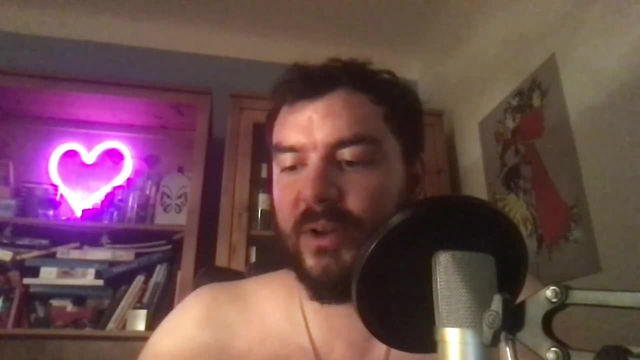 about God in the world. they must have had it wrong because they didn't have the formal tools, that they were not rigorous enough. so naturally, this, the time in which this is written, is about the same time as these formalizations of set theory comes up. and this is not an accident, because a few years prior, the 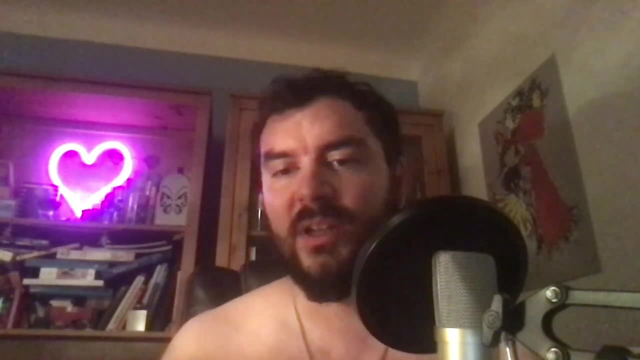 whole, you know, logic season project was started. they had then their takes on science and the world in general, and in particular the world of science and the world of science and the world of science and the world in general, and in particular, mathematics and turning mathematics into logics, arguing and arguing for the. 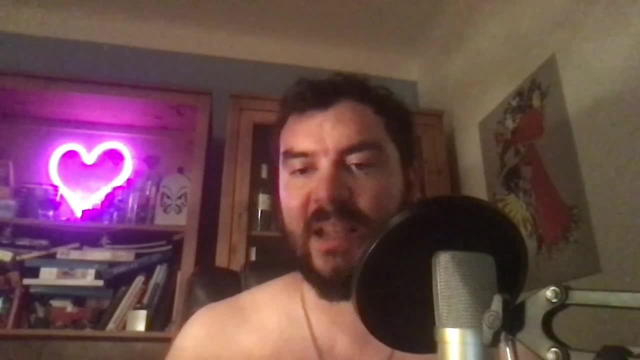 idea that mathematics is really just logics. I mean, this gets a little bit fussy on where you want to draw the line and how you want to use the words, but the the connection to regularity here is that, if you and I'm going to be brief, 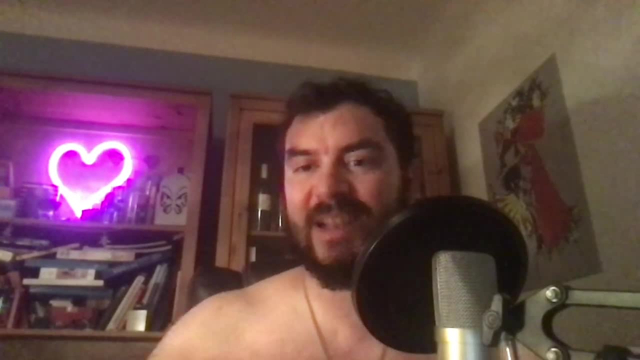 here to have enough time to discuss actually the, the set theory in in some mathematical detail. but the connection there is that you can view set theory, whatever set theory, whatever axioms you adopt, as a higher order logic in the sense that there is a correspondence between classes and predicates and sets. 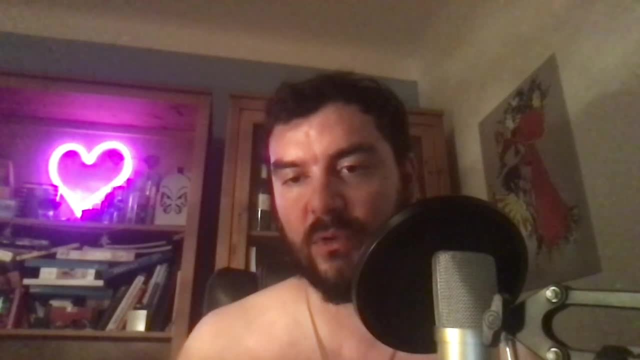 as a special case of classes, are therefore also predicates, and if you have, you know, an element hood of sets, then you're expressing properties. so the simplest example is: you know, you have the set of natural numbers and test the property in the natural numbers of being a multiple. 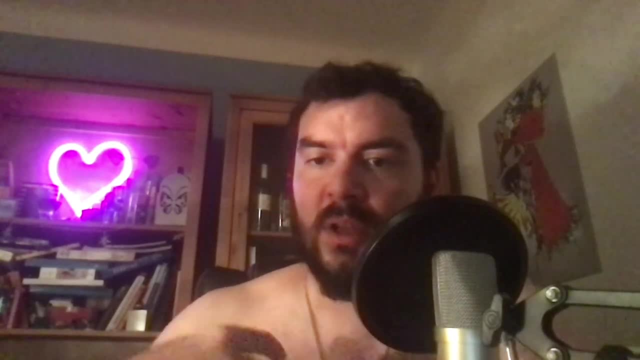 of seven. so, for example, twenty one and twenty eight would have the probability of being multiples of seven, whereas thirty does not. and you have this property that are just expressed and at the same time you characterize some subset, in this case an infinite subsets of the natural numbers, and that is a. 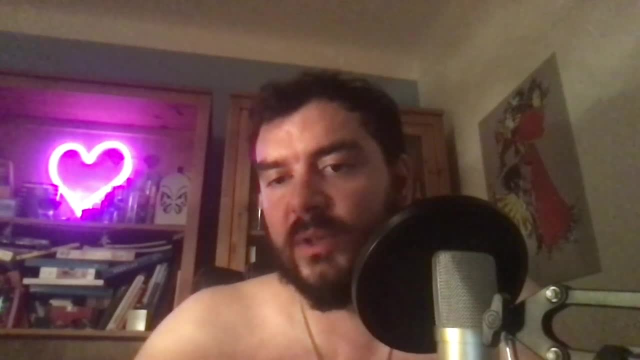 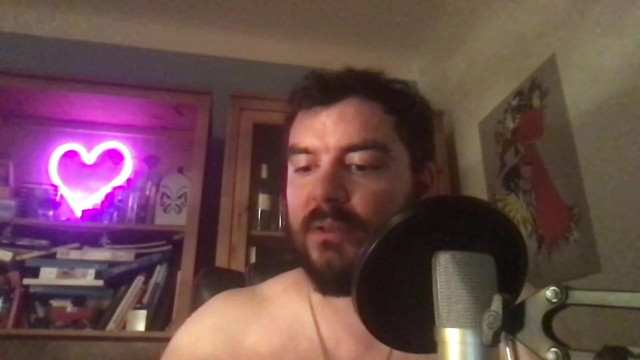 set and your, your set theory has quantifiers over sets and so it has quantifiers over predicates. in that sense and in that way, you have the capability about talking about, you know, existence of predicates, and the one complicated thing in logic is always, you know, reflexivity, things talking. 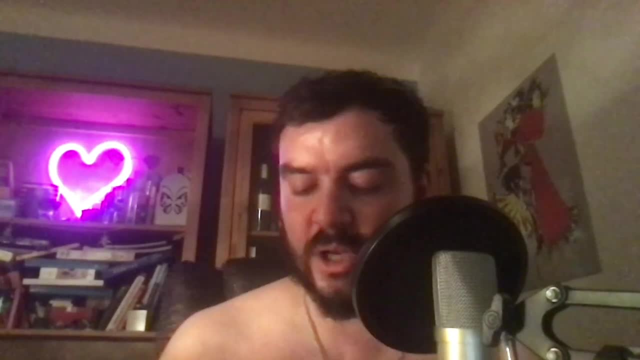 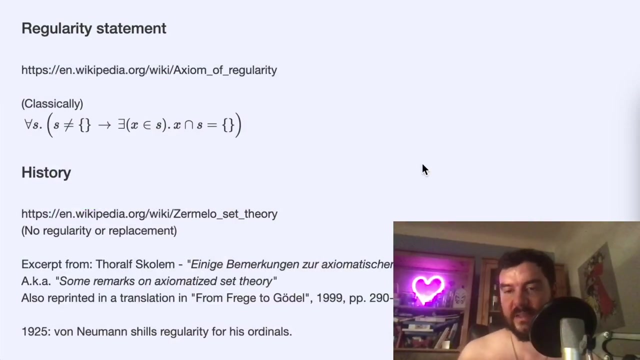 about themselves, and this is also the, the scenario in which in Kurt's interview that that came up- regularity is interesting insofar as it is that axiom which was adopted to rule out the, the possibility of having sets which contain themselves and in in in this, in the sense that 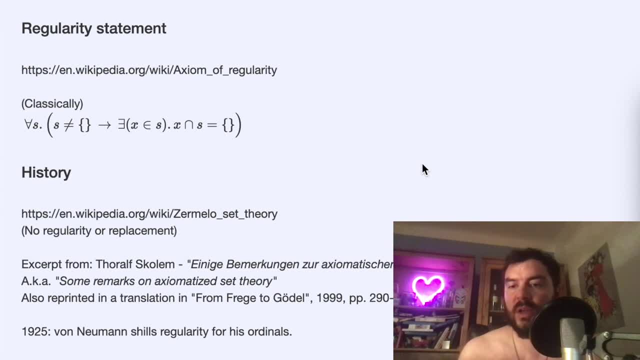 I just described this. this means talking about properties which exhibit the property that they are themselves right. so you have a property and it it might have some properties and it had might have itself as property and and so on. so on the property side it might get confusing quickly and 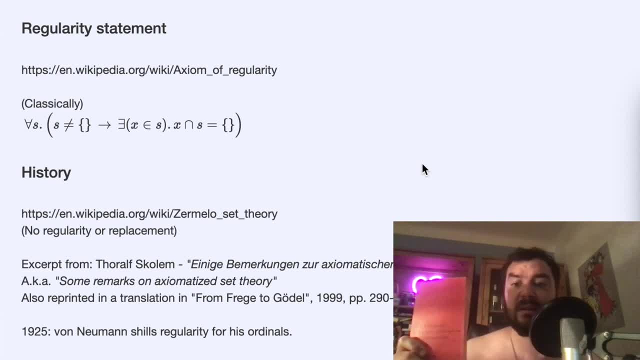 indeed, when people were developing, developing this stuff a hundred years ago, it was like pretty confusing. now the funny thing is, if you retract artists now and you're familiar with some introductory textbook on predicate logic, then you will have to feeling that this guy is, you know, spending a lot of pages for things which are relatively simple because he has 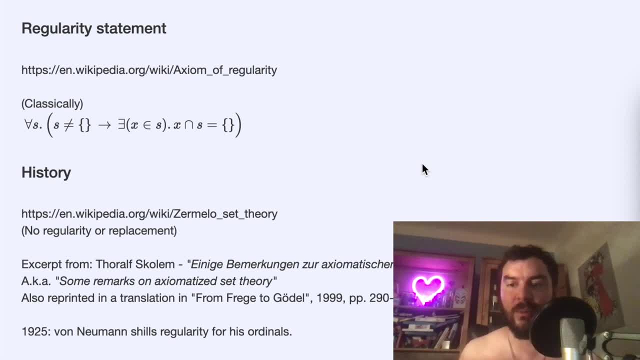 to explain. you know. he really explains what the tautology is and how predicate logic works and he surprises the reader um 100 years ago with with some of this formal logic things, and then he has his spin on how it relates to ontology. truly coming to it today is 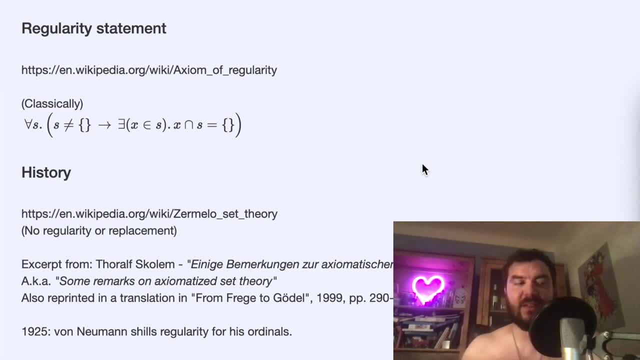 like it's. it's funny to see how, how things progress, how things like become the, the common knowledge, the common language, and and how. then it appears that this is like wasting a lot of time on things, that you could just read a math book first and then say everything much quicker. I actually got this book when I moved. 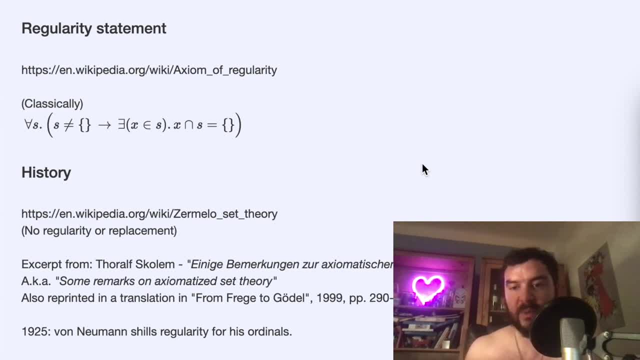 to Germany. you know, I moved to Germany um to the German Aerospace Center to do my PhD and there was Adrian, a physics student who was also studying philosophy and you know I was interested in in Wittgenstein. back then I discussed this with him a little bit and then he, when I, when I, when I went away out of 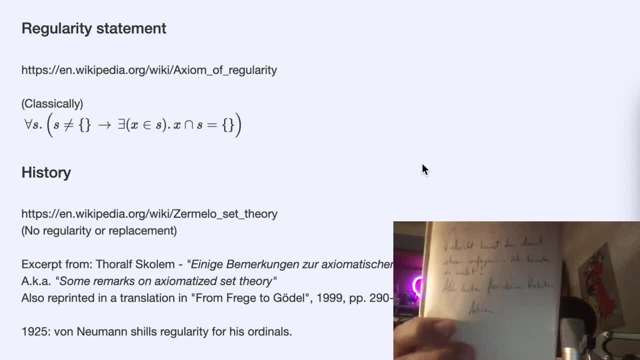 Vienna. he gave me this book as a farewell present, with this cute inscription. he says: maybe you can make something out of it. I couldn't. good luck with your rockets, um. so he had to read- read that for his courses, but obviously he found it weird and had not much fun with it. but I didn't read it. I actually. 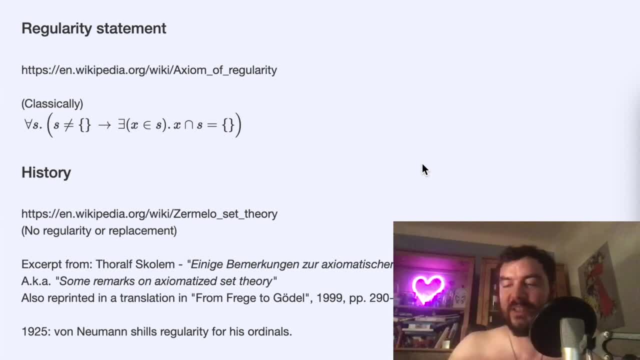 read it in front of the house that Wittgenstein built. you know he was. he was in Vienna and it was quite influential, not because I agreed with with the text, but just to see how things developed. right, this was before I got really into formal logic and, um, you know all the math. I study, I study. 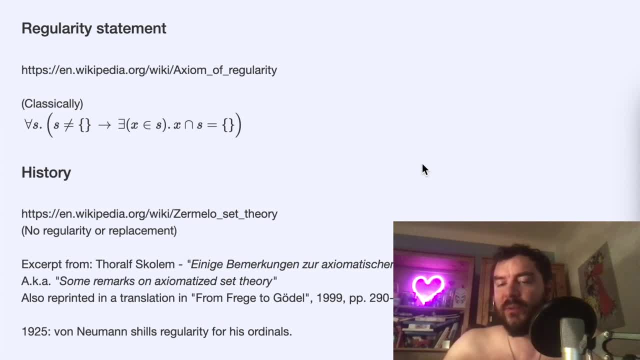 for doing physics. I'm a physicist but, um, if you would look at my- my- YouTube channel, you would think I'm just interested in logic. but it is for the purpose of doing proper physics, and this was before I really understood all these things, and it definitely influenced me in a way. 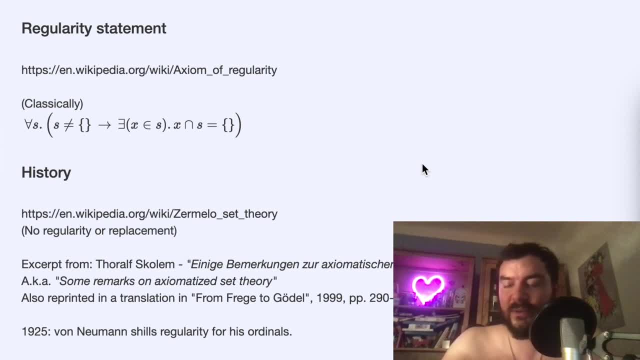 that when I finally came across people discussing physics, computation and all these things, I I was already hooked right. I was already saying, oh, there are some interesting things that I want to understand better. okay, so, um, uh, with that said, you know, I I discussed this quickly because my motivation is here to to show. 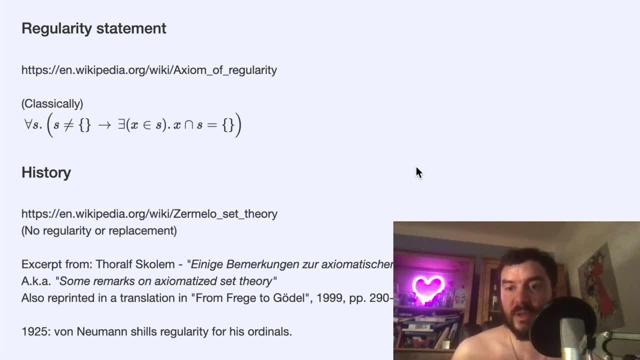 that if you talk about um, uh, sets, including themselves, there's always also the mirror image where you can say: this is about predicates speaking about themselves and and uh, and you don't have to force this sort of reading on it, but it's worth uh, keeping in mind and reflecting on it. 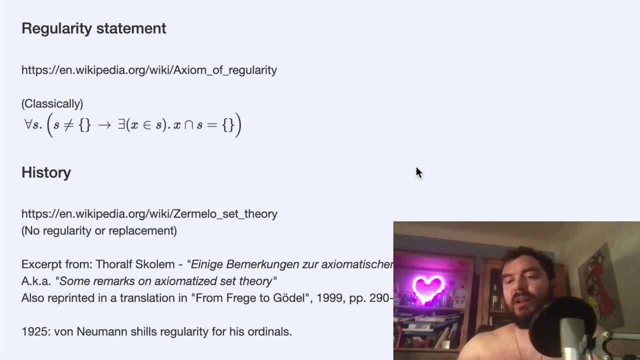 and the same goes um the same. you know the same Wittgenstein sort of relationship between, or you know, idea of relationship between formal languages and, and what we have in our head or what we can think and express was, is of course always brought up, still today, and people make. 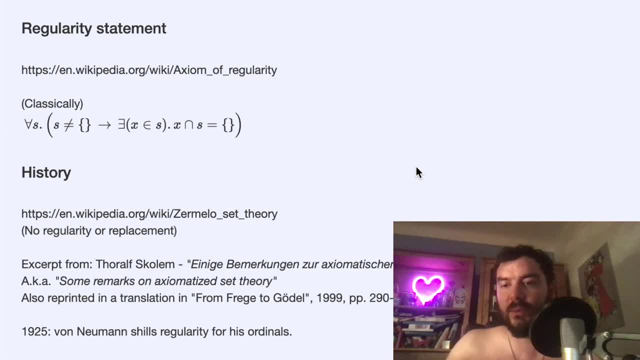 arguments in one or the other direction. I will not make a judgment on that in this video, but when we talk about um, first order logic, which is sort of the the nice logic, with completeness theorem and so on, then uh, there's always the capability of reflecting on it. what does it actually mean? 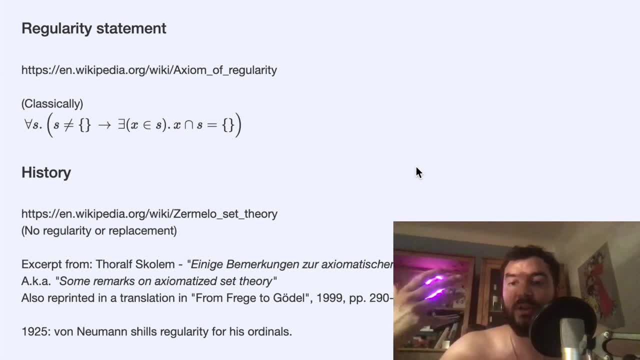 for a pessimological reasons, consequences that mathematical theorems that we're discussing have on us, or if they have or do not have that, and, in particular, when we talk about a theory being able to capture some models, categorically or not, as we would see in this video what that really means, okay, so, with that said, 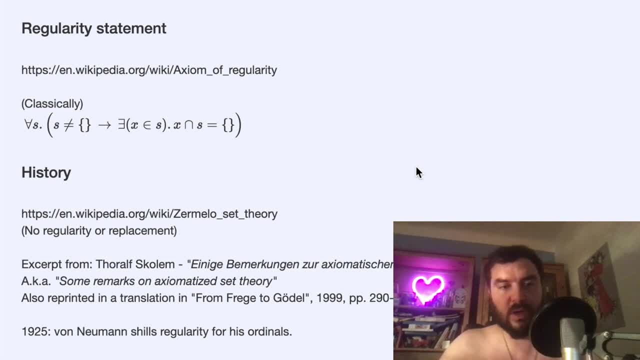 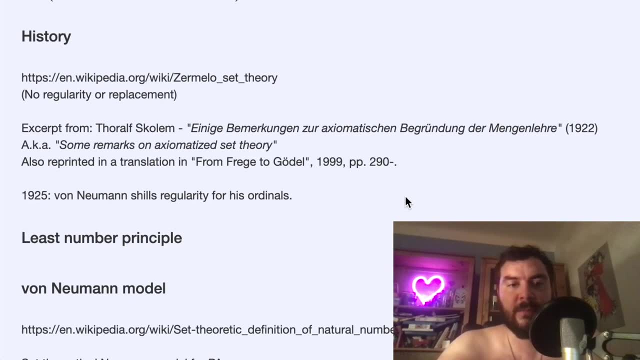 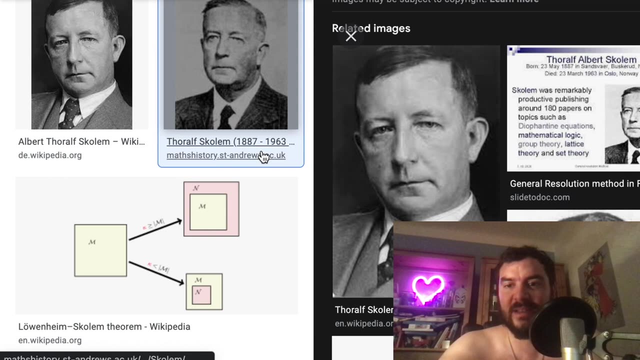 um, let's jump into the video. uh, proper, so I have here for you, um, that might be interesting to read if you want to know some history, and I have a screen kept um an excerpt. so there is this guy's golem I have to page here. is this very um happy looking fella? um, he uh was reflecting on. 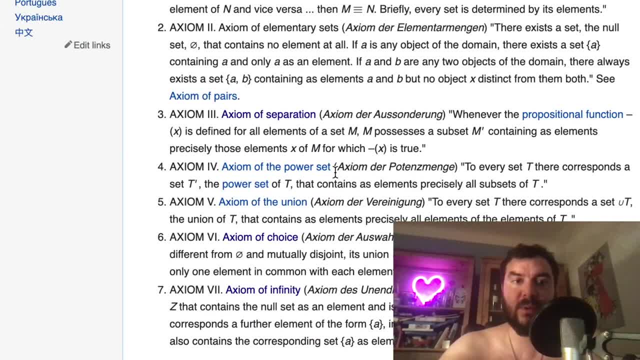 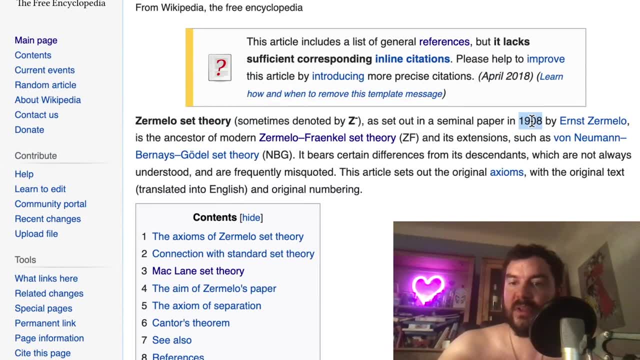 cemelo's Fury. so cemelos Fury. I have the Wikipedia page. here is um the set Fury of that dated here which is before cemelofrenkel set theory, right not to be confused with the cemelofrenkel of cemelofrenkel choice set Fury. that is the standard set Fury in academics. if 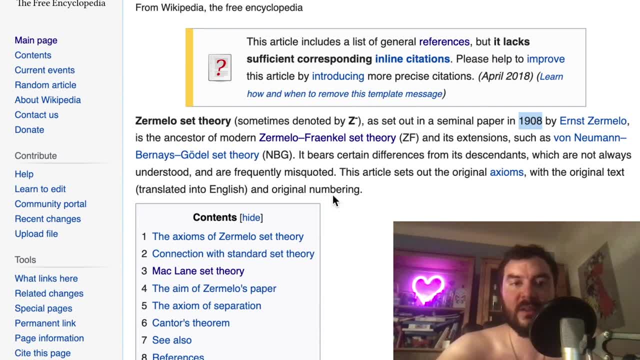 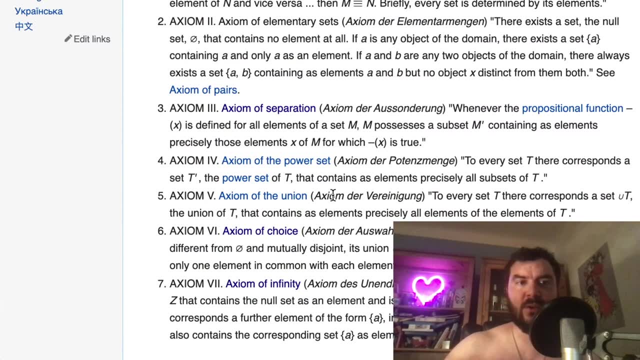 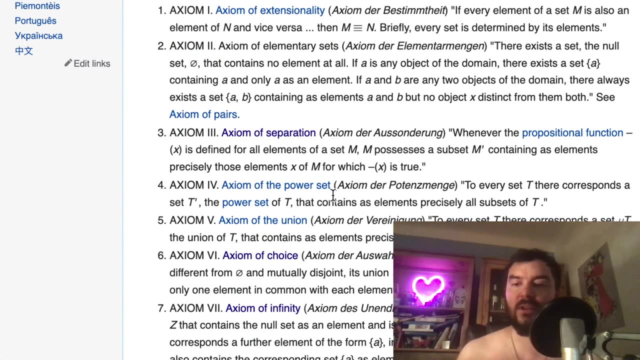 you. you can say that like that today. this was sort of the precursor and, uh, cemelo wrote down a bunch of axioms. these are now here on the screen and notably: um, they don't contain the axiom of regularity, right, so he did not have have that here yet. um, and it also does not contain the axiom of replacement, which is very 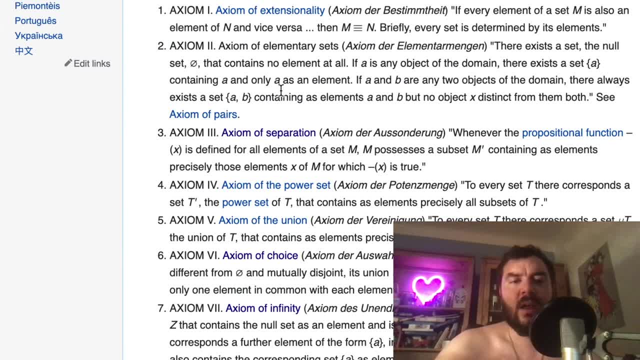 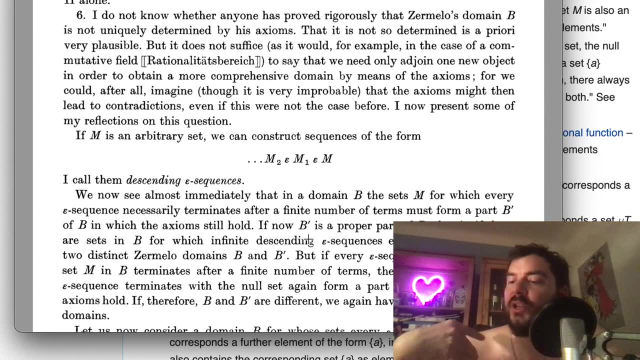 interesting but we'll not discuss in this video. so, um, he published uh these axioms and then people like uh tomato came along and uh pointed out some, some features of that: that Fury, in particular, the degree to which it does not really um pinned on a particular 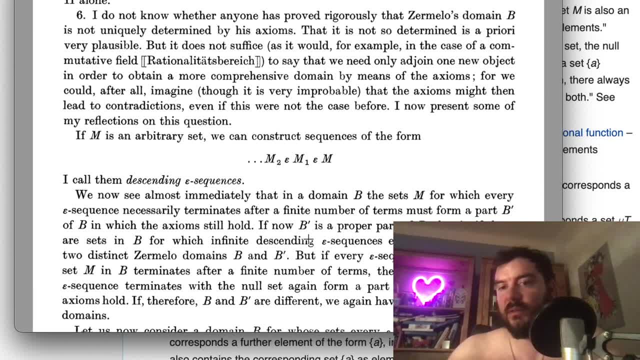 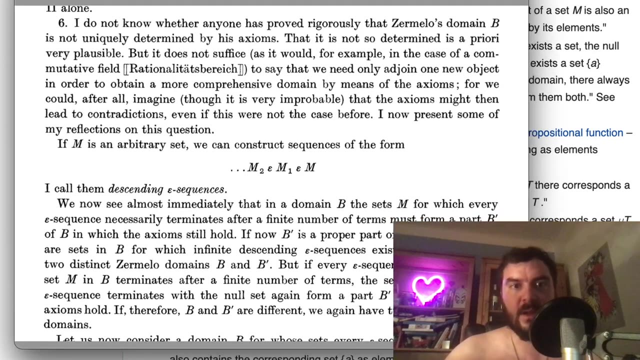 idea of sets. so if you want, you can press pause and read this uh little piece from his, from skolem's 1922 article um, where he uh like highlights how sadly my screen is there, let me actually make this smaller. he highlights doesn't really work. he highlights how, um, okay, sorry, I cannot put this on. 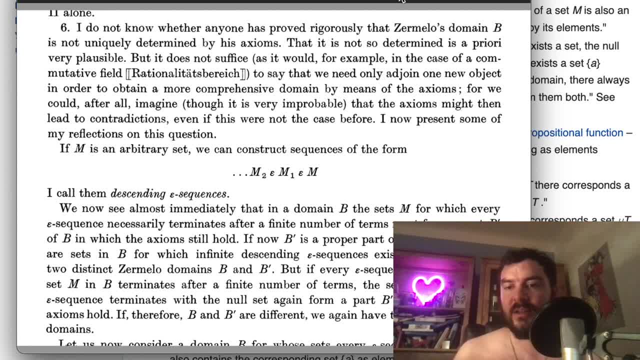 the wall um. he highlights how, uh, the, there is the possibility in similar theory for this infinite descending chains, for sets which contain themselves, and that the, the set um enables the interpretation for two domains, B and and P, prime, one with and one without these, this sort of um self-containing sets. 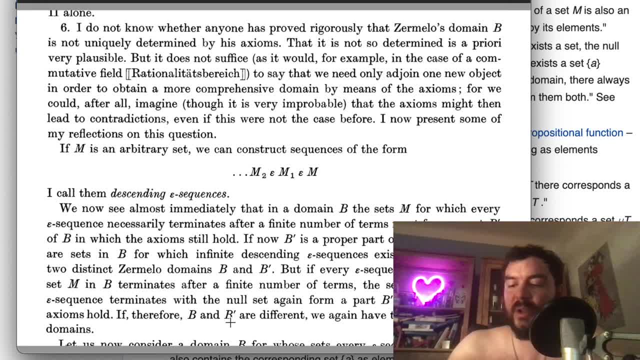 and so he reflects on that. and it is then, two years later, when von Neumann who came up with his ordinal Fury, ordinals modeled in in set Theory, where he wants to use um well-foundedness, property and induction, and then really advocates for, for adopting, uh, the axiom that rules out this um self-containing. 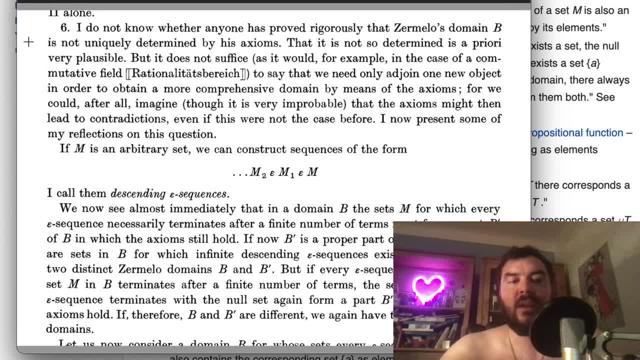 object. so this is sort of the history where we have it um. it is also equivalent then to induction principles which can be proven from it and um, this will be the topic of another video, for of mine I think I will make another one hour video on the topic of transparent induction. but to keep it short, 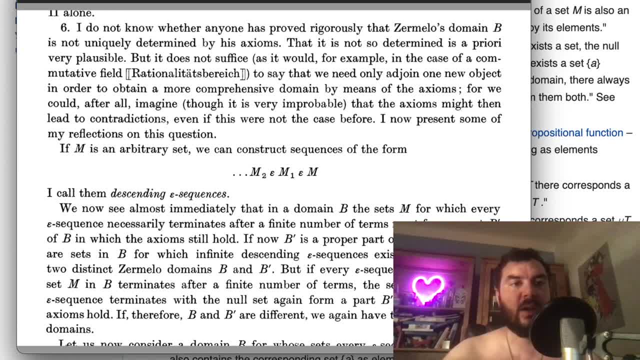 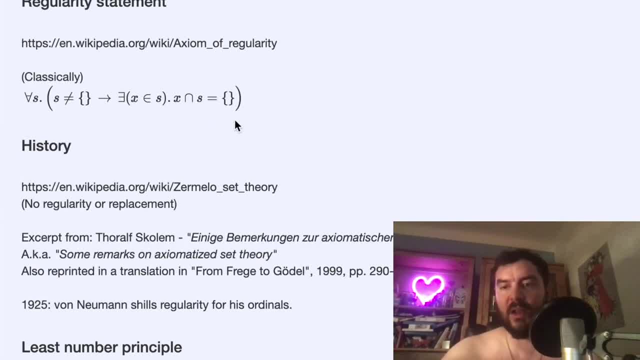 in this video. I will just talk about arithmetic. okay, so this is for a little bit context. um so, uh, let's actually like spell out what does the axiom of regularity say? so it says for all sets if these sets are not the empty set, ie if the sets are not empty, then there exists an element. 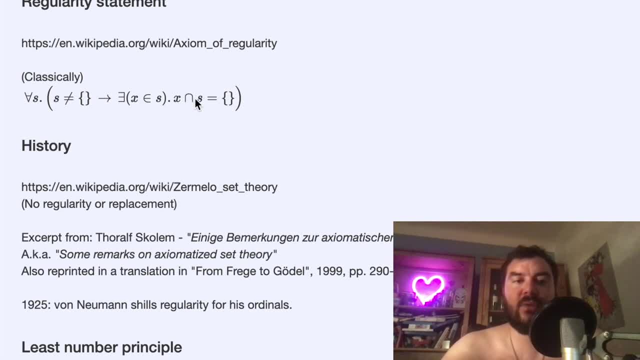 such that in S, such that the intersection of S and X is the empty set. so again, if you have a set which is not empty, ie classically, which contains some element, then there is also an element in S which is entirely different from S in the sense that they don't share. 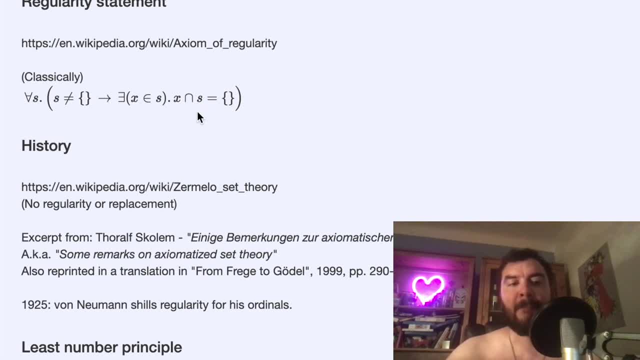 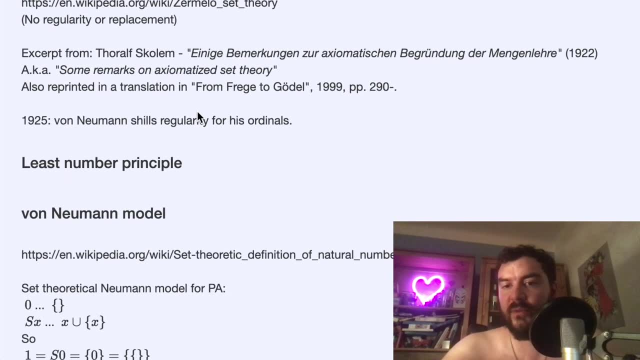 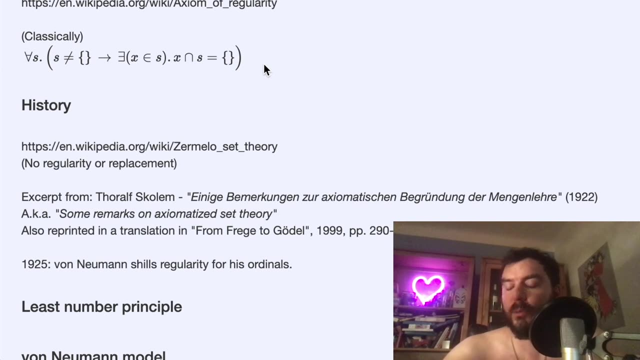 any elements. right, this is what the axiom says. um, we are going to uh discuss in the video the least number principle in arithmetic. so you know this is the form um it. people always say this is a little bit obscure um compared to other axioms, maybe similar set theory. um, the nice thing is we are. 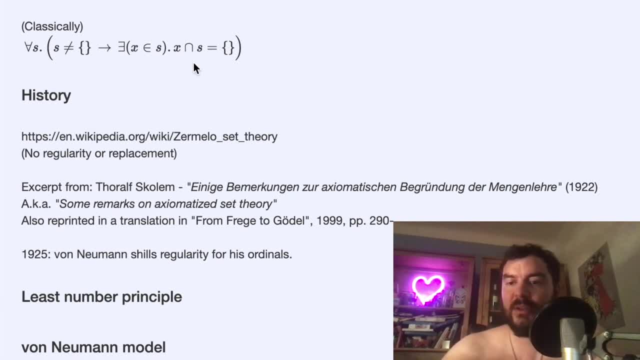 going to discuss the least number principle, which has basically the same form but which, because the natural numbers are only countable, um interpretation and it talks about minimality. and then you can take some of the intuition back to set theory, and people also like to usually express regularity as sort of the existence of. 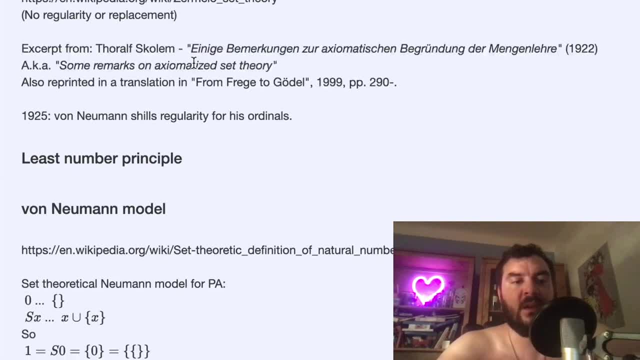 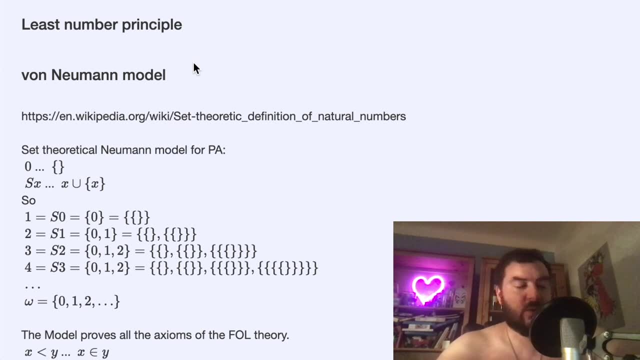 a minimal element and we are going to discuss what it means, so okay. so I want to talk about the least number principle and for that, um, I would have to say some words about the von Neumann model, because we wanted to discuss the minimal number principle also in. 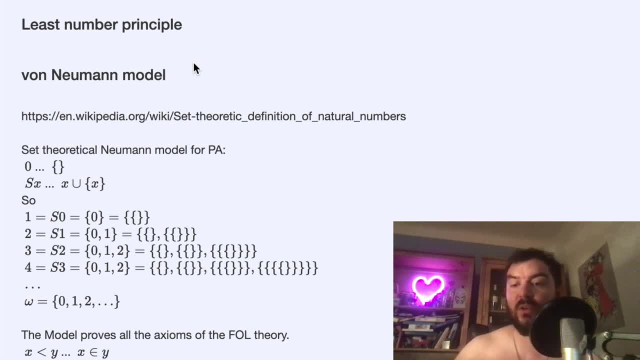 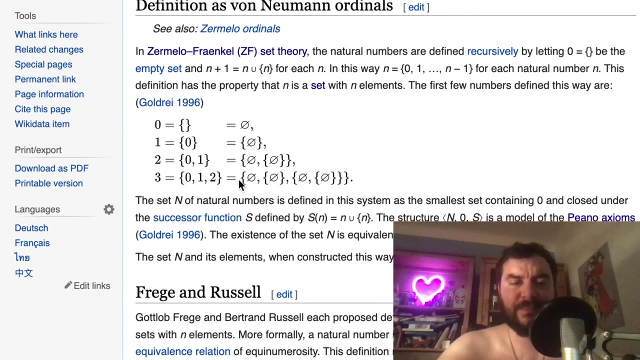 its incarnation of set theory where it looks most close to the regularity axiom. so, um, I mean, I have again here Wikipedia page open. I'm basically just show you this to to give you a reference and to show I'm not making things up. but the von Neumann model, uh, you know you can. if you don't know it. 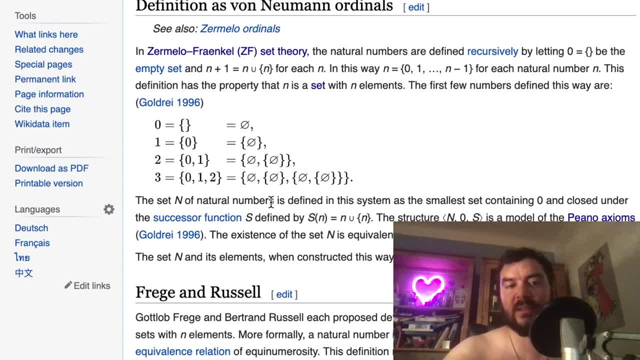 then you can look at the page if you know it. um, keep two minutes ahead, but it is the one way to encode the natural numbers in set theory. what you want to do is you want to find some set which contains objects such that, for the totality of it, 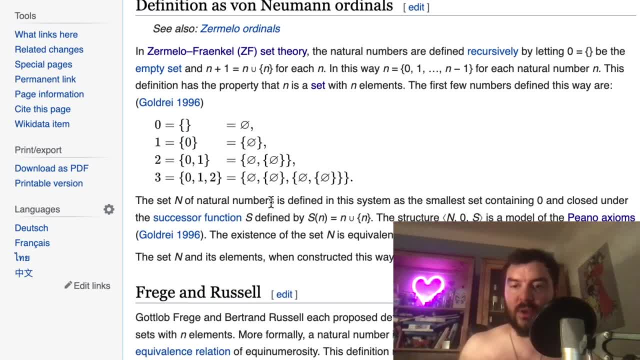 you can prove all the axioms of piano arithmetic in this case. but it really goes for any theory that you model. in your set theory you find objects and then you show that with the axioms of set theory, um, the um, all the axioms of the theory which you want to represent, which you want to model, are fully. 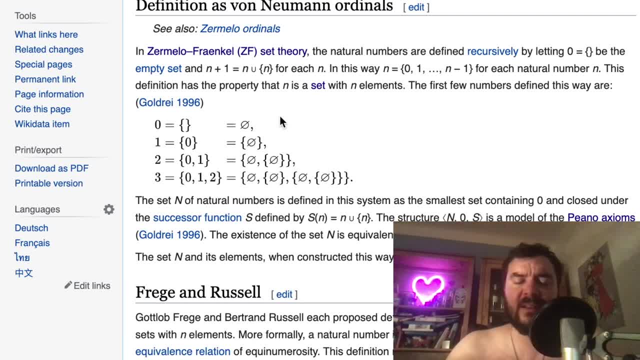 fulfilled. and what? what you do here is the axiom offset period, tell you there's some empty set and then you can do: uh, use, pair, uh, pair construction of sets to construct other elements. and in this way, what you do is you postulate: okay, the empty set is going to represent the number zero and 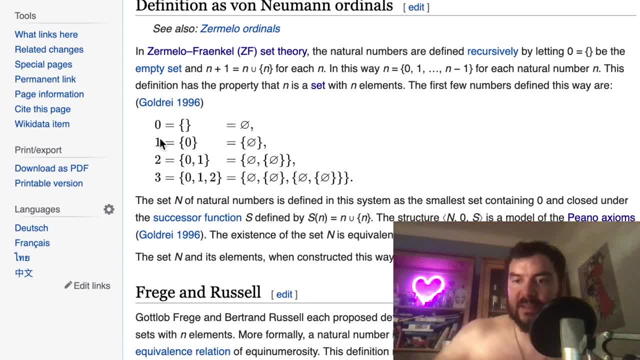 then every subsequent number is represented by um, a set which contains all numbers so far. so, for example, the number one is the set which contains just zero, the number two is the set which contains zero and one, the number three is the set which contains one, two, three and so on and so forth. so the number 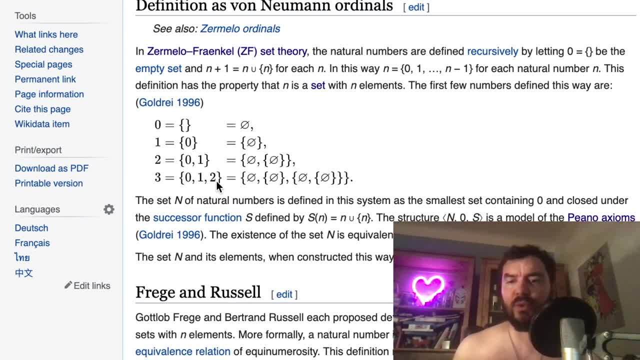 2000 will contain um 2000 sets. right, it will contain zero one, and so on, 299, um 1999.. um, and then, And then, if you want, you can of course then write it down what this means in terms of the empty set, and you'll find all these sets are sets next to each other and nested, and eventually you get down to the empty set. 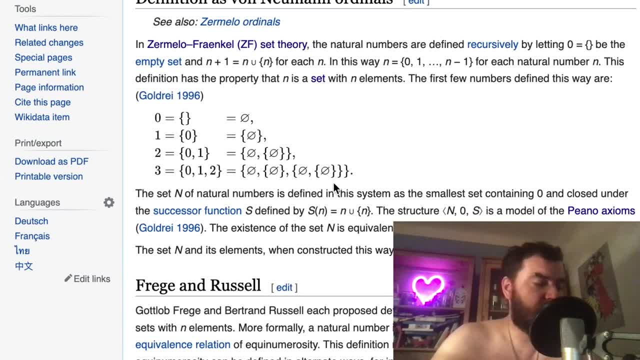 The theory of piano arithmetic. as we will later see, I will show you the axioms explicitly. but it has, as a primitive in general standards presentation, in its theory signature the successor operation right, which takes you from one number to the next, to the successor number. 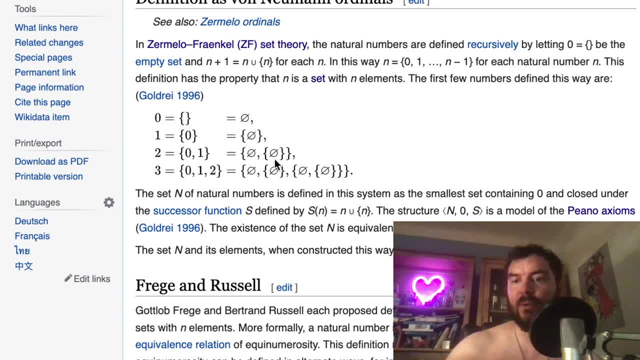 And conveniently for this particular model- you know it's not the only model of the natural numbers in set theory, but for this model you can represent the successor operation as it is shown here. you say: you take any set, in this case we will apply it to the natural numbers, and you build a union with the singleton set which contains n, and then this actually takes you from one set to the next. and if you want- you can, you know, test it yourself- you can take the 2 and apply this operation to the 2, then you get necessarily something which also has a 0 and 1 in it. 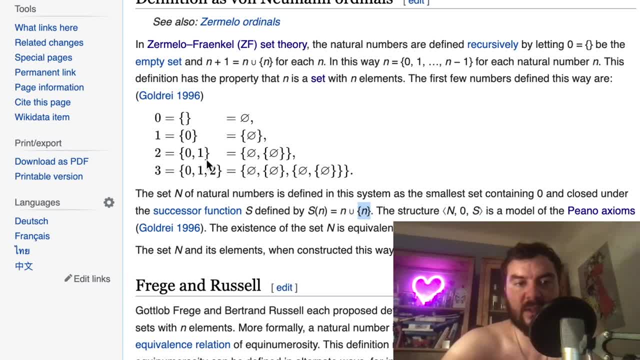 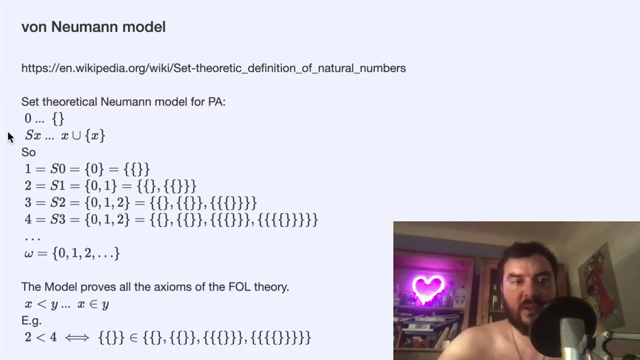 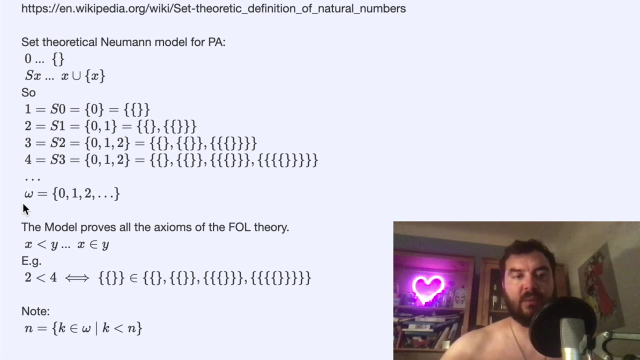 But also the singleton which contains this thing, and indeed, this is exactly then, this is exactly then this set, Yeah, okay, So okay, I've written this down here, the S I have constructed in set theory with the axiom of infinity, you also have an infinite set, which is the set which contains all of these numbers. 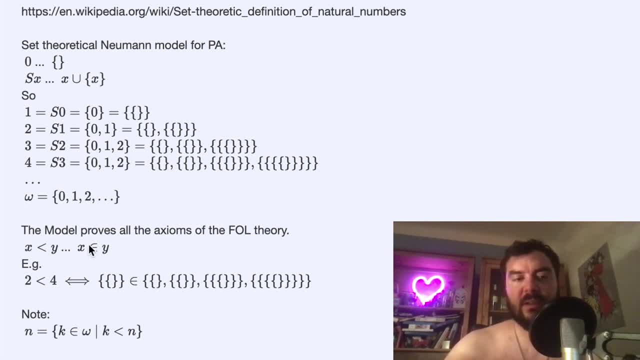 Also, one nice thing about this model is that the if, x and y are just natural numbers. in this sense, then the order relation, the strict order relation, is smaller than is represented exactly by the membership. so you see, for example, that the set 2 is inside of the set 4, basically by construction, and indeed 2 is also smaller than 4.. 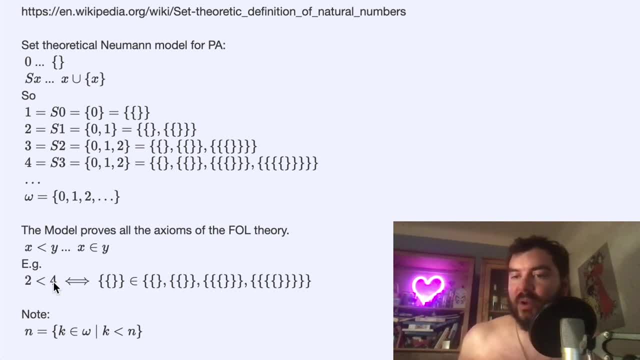 So small. the natural, smaller than relation that you have in mind is exactly represented also by membership. so this is how the order is implemented and indeed, you know, this does not actually just work for the natural numbers, it also works for ordinals, which come after it in the von Neumann construction, but we are not going to need it in this video. 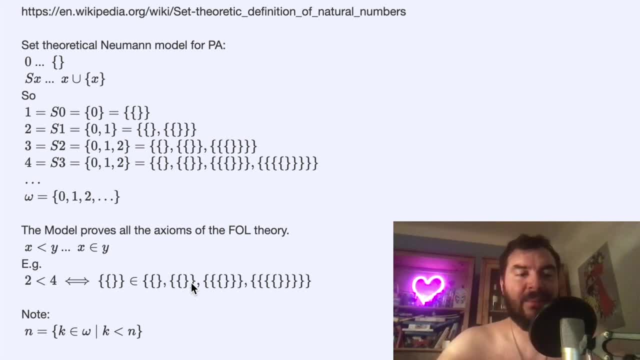 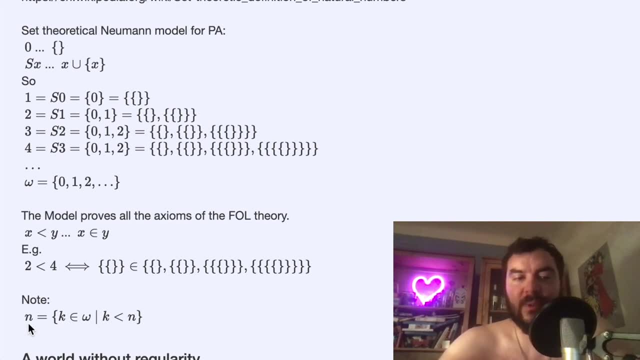 We are going to need it in the next video, Okay, and so, as you see, down here, there's also this equality relation where you know, Firstly, I have here- Sorry, There is of course a 3 missing there in the 4.. 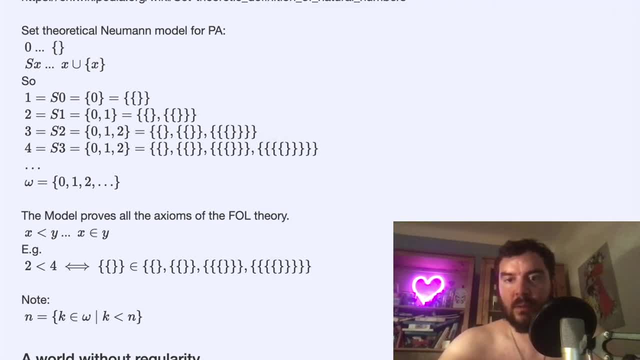 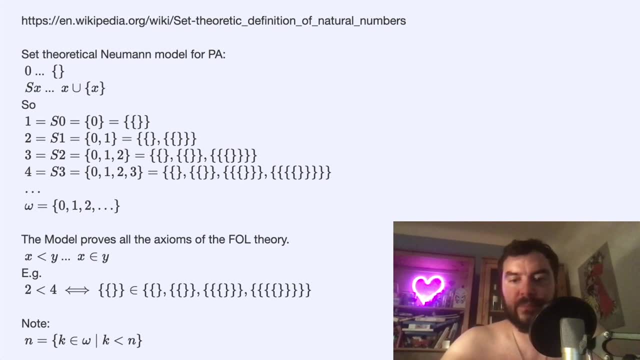 Let me actually fix that, Okay. So what I have here also is a statement that every natural number in this model has a property that is actually the set of all natural numbers smaller than it, again, you know, by construction. this is how i started the definition of them. 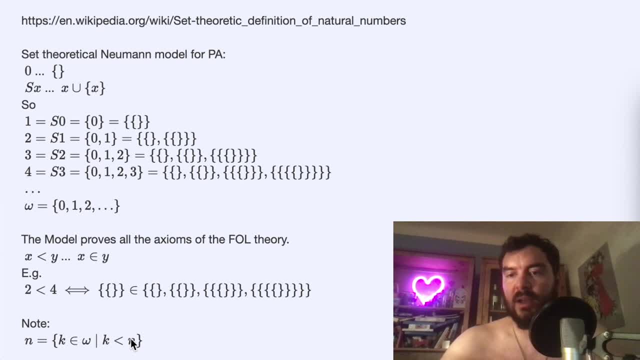 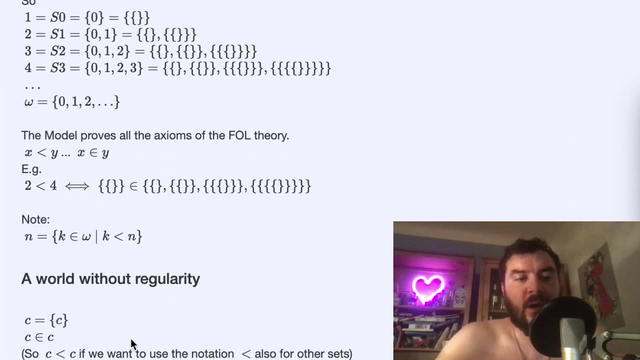 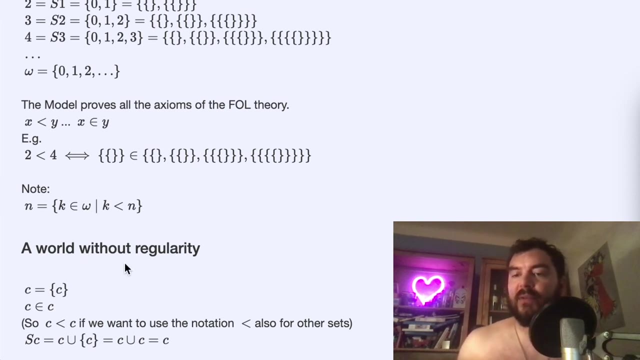 and this is a relation that's going to be relevant to formulate the least number principle in the set theoretical case. okay, um, here one note, right, if, uh, without more context, let's say for a moment that there exists a set c, for example, which contains itself. now, this is what's ruled out. 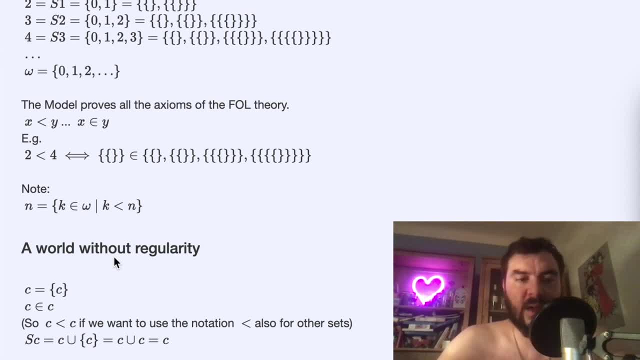 by regularity or by induction, but um, for the moment, let's um, let's allow this, you know, don't adopt similar fractal set theory, but actually allow this object. then, if you things are true, like now, by definition um c is a member of itself, right, and then so um. you know this order, relation i. 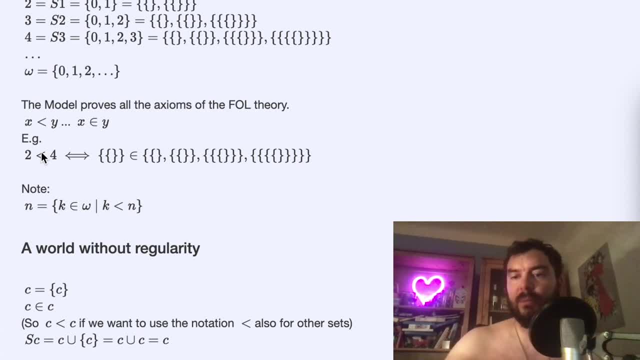 defined it for natural numbers or for ordinals. but if we also use this notation for c, then we see that, for example, c is smaller than itself, right? this just says that c, you know, by definition. this just says that c is a member of itself, right? so formally c is smaller than c. this 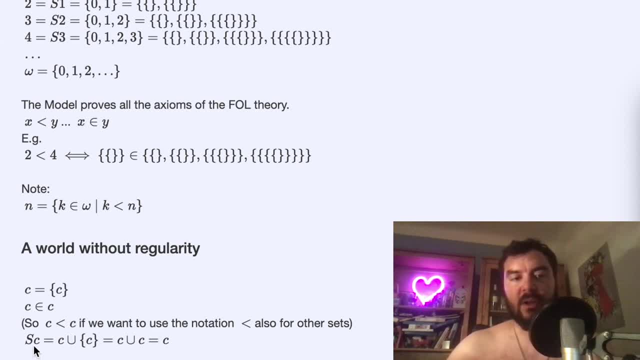 said this, then you can make this construction and also: uh, the successor of of c is uh, c itself, right, because if you just apply the definition of the successor, and the singleton is just c and the union of a set with itself is just the set itself, so you have this sort of this phenomenon. 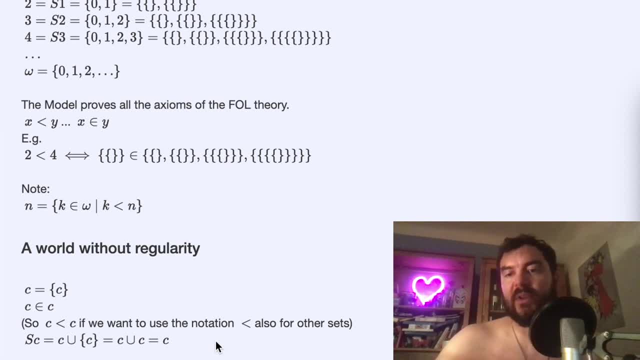 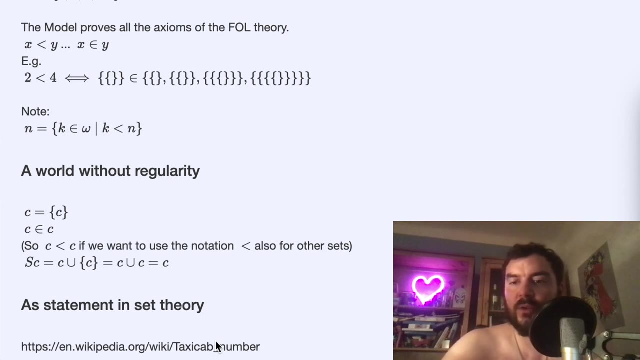 right, um, i'll emphasize it well, because something i like will also appear with some models in the with the robinson arithmetic, okay, um so um, i want to talk to, uh talk, about the least number principle in arithmetic. this is something which is basically equivalent to the induction axiom right. induction is the strong axiom schema. 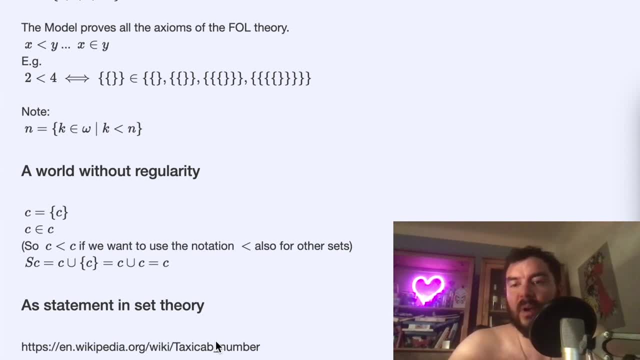 in piano arithmetic and i will show you the families in a second. but what it says is the following: it says that if in the natural numbers and any property that you choose, if there's some number which has that property, then there is also some smallest number which has the property. 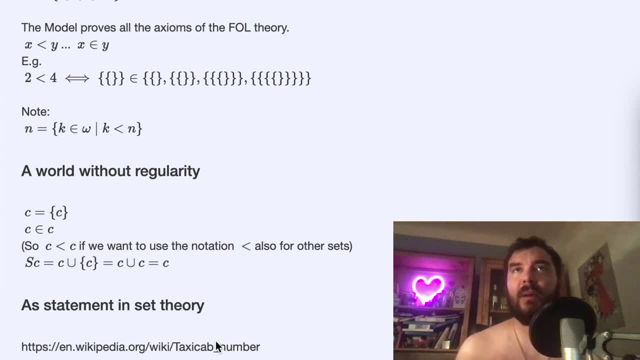 so, for example, you can talk about the numbers which are bigger than 50 and divisible by 7. right, and i can immediately tell you: a number like the number 7 000 is for sure, divisible by 7, it's bigger than 50.. and the least number principle? 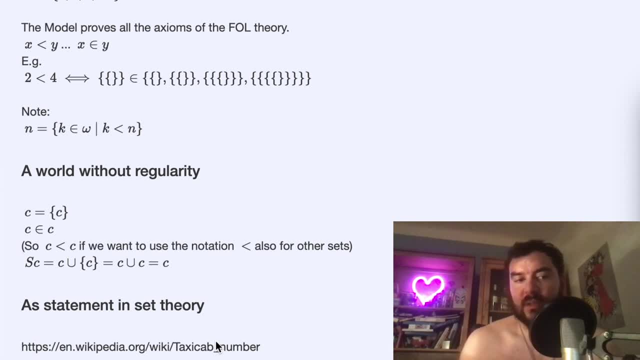 states that, okay, there exists- i i just gave you an example- there exists a number which has the property. then the least number principle says that there's also a smallest number- small with respect to the ordering in the natural numbers- which has the property. and you know, i could think. 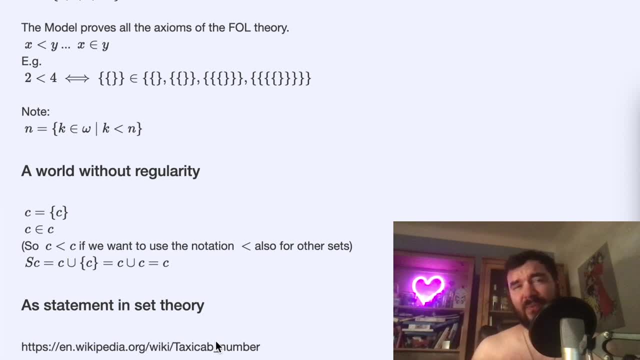 about it now, i guess it will be. is it 56? i guess it's 56 divisible 7, i think. so i think this is like good royal family territory. um, i don't want to think about this. it's effect too much now. but you see, um, this thing says, uh, that, like the other axiom, the schema says that such a thing must exist. um, the classical variant in any case, and indeed the lighthouses are uh, mouth water, and they should in case there is an adoption of the extreme capital A of relative flight of scale developed with the dictap, unscrew the protein of line of the one after the other right, so they close the gap and then the opposite of theility phase and cause theert clicc crimes. 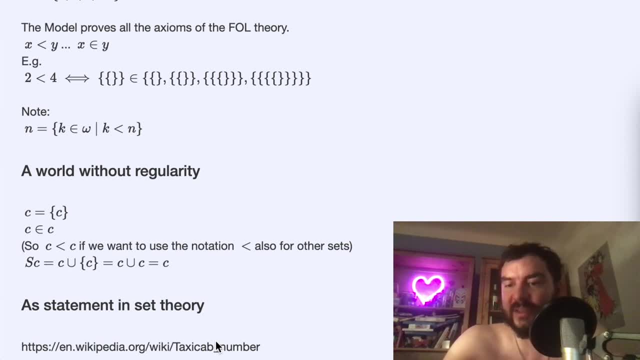 junior, classically variant in any case, and indeed Sonia likes a good behavior. you can see now aographers, city'll buy one or lessami take the reaction to the Love Noms or any VOA code, this case. i can immediately, even, you know, tell you what it is just by thinking about it, okay. 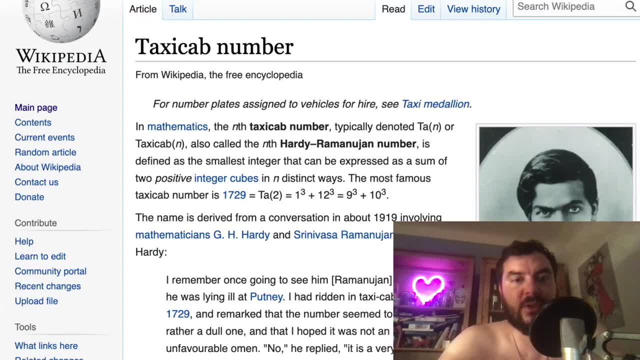 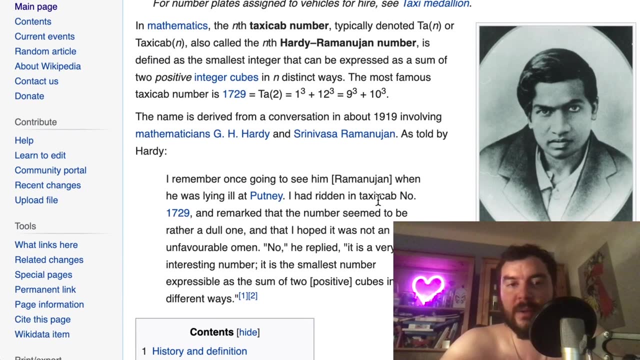 so i i had an example here for another property which is, um, you know, yes, famous, the, the taxi cab numbers. are these, these uh numbers which can be written as the sum of two cubes? there's this nice ramanujan story and this is also, you know, one of these properties. like being able to write it in. 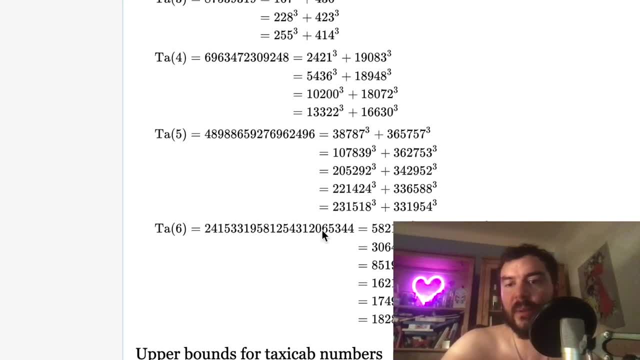 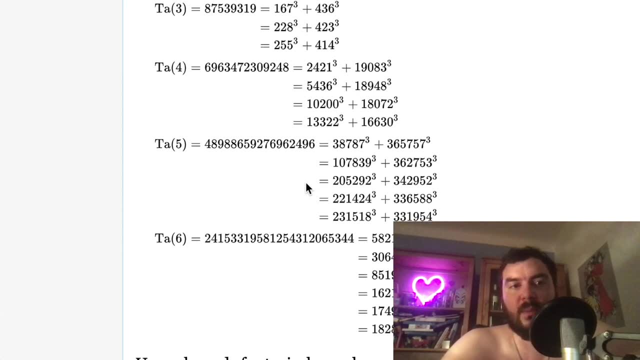 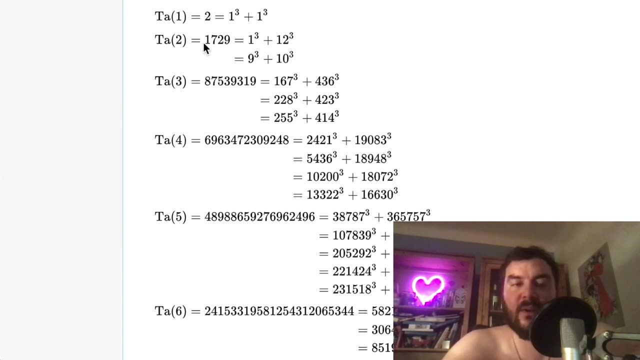 various q ways of sums of cubes. there's some big numbers which have the the property, but the least number principle will tell us there must be some smallest number right, and if you allow for the number two, then the smallest example will be number two and of course the famous 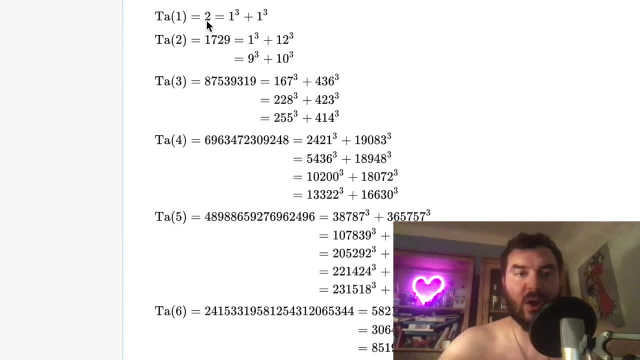 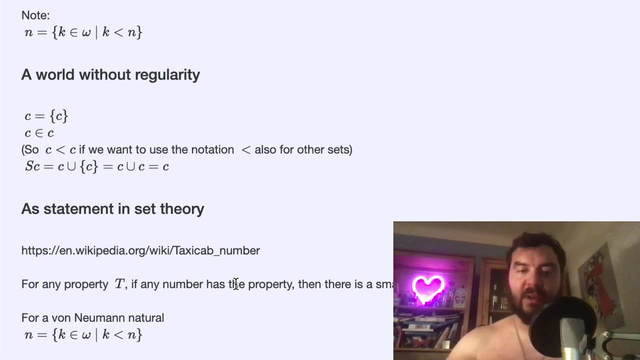 number is this 1789. you know, if you rule out- i don't know- this sort of sort of trivial case, then let's say this is the smallest example. this is just my motivating example here. okay, so this is the property. we are going to see the formal expression in um, in piano arithmetic, in. 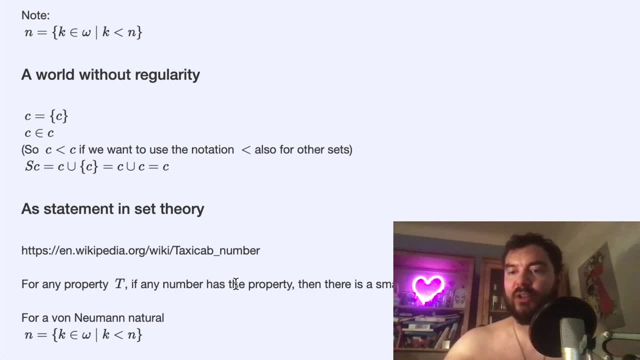 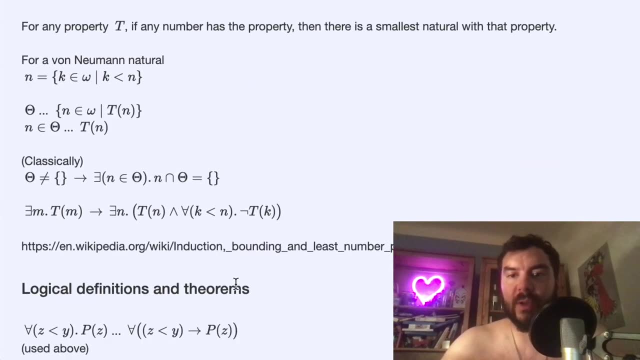 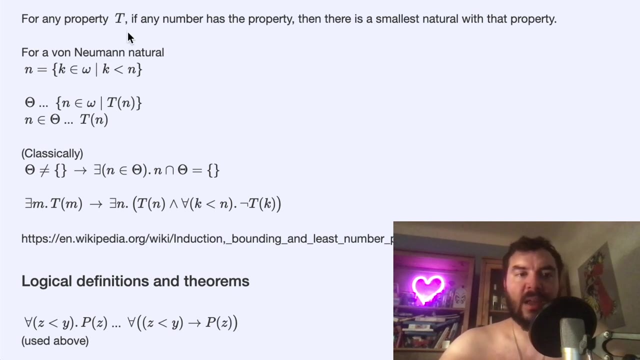 a second. but what? how do you write it actually down in terms of the model that we just discussed, right? so i call the generic property: um. okay, i will just show you the whole page, right, and don't make any secrets. so sorry, um, i call this generic property t. this is we're going to have. 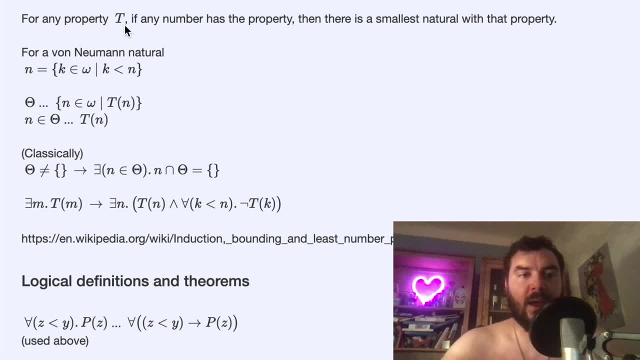 this as a schema. it works for every property and, um, um, i just said the. the normal naturals have this property. um, i can define the class. for every property, you can define the corresponding class, and if you have full separation, the separation axiom, then this is also a set. so i can just as well call it set theory, assuming you know the. 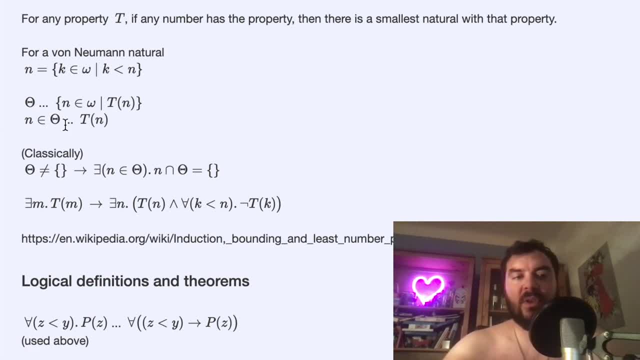 strong set theory. and um, here my dot, dot, dot means always the sort of definition or equivalence, so to say that the, the number n, is in this class, this subclass of the natural numbers or subset of the natural numbers. class notation really just means that being able to express t of 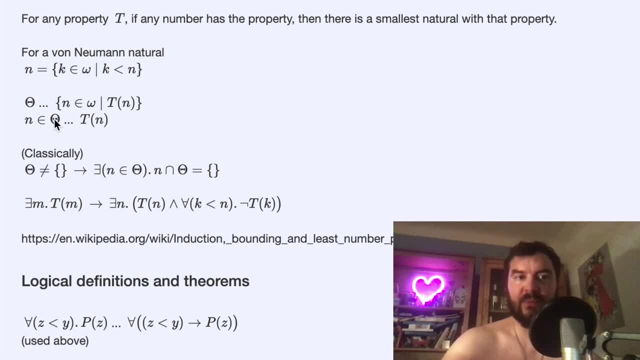 n with the element hood symbol, right you, if, if um, theta is just, uh, some class, then this is: this thing here on the left side is really just notation for the right hand side. okay, and then um, the. the statement which i just made about minimal elements is written down exactly like: so, so you. 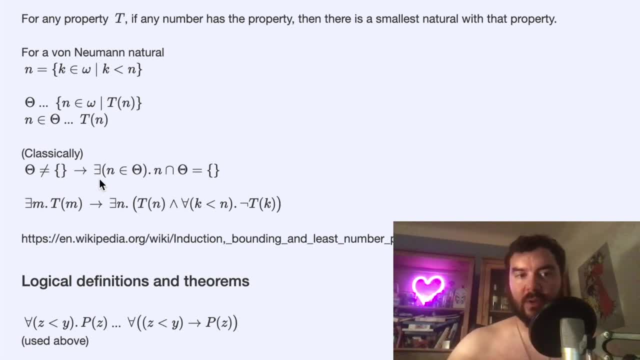 know if i, i will spell it out again and you can follow here in this set theoretical formulation: if, um, some, a number has the property which classically is the same as saying that the class is not empty, then there exists a number and this number is going to be the smallest natural number. 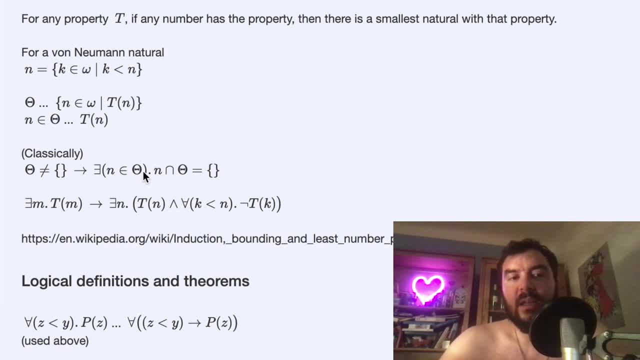 with the property and in the model, in the neumann model, um, to say that there is um, you know, to say there is the smallest number with the property, is to say that no number below that number have the property. and if i build the intersection of n in the model with this subset of natural numbers and 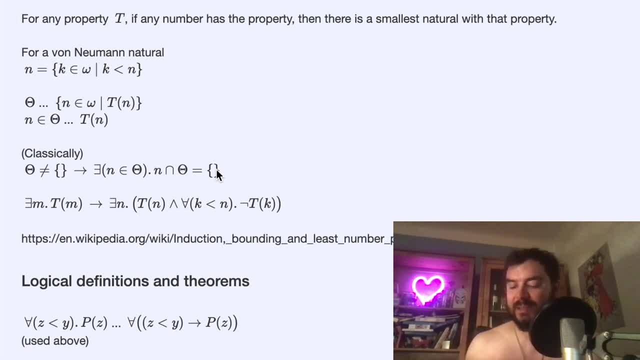 the intersection is the empty set, then this exactly means that there is no number below n which has the property t or theta. right, so to say to say that the intersection of of n, meaning all numbers below and theta, is empty, just exactly means that no number below n has. 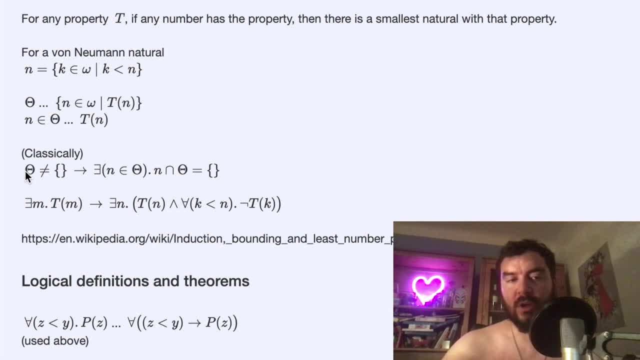 the property t, if you think about it, for a second right. so here's also the right below the statement um. for this instance, t in piano, everything, some. now i do have a stop at some places. actually the equation isn't the same because it actually its the same because of this: 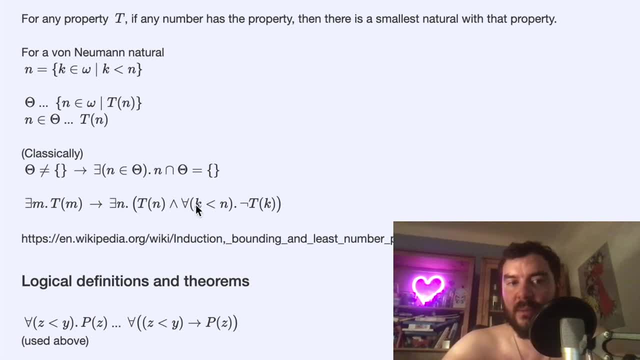 bahc. i'm not really pro in quantum, but it's clear to be clear that it's weight, and so the energy is usually already in a vertical formula. that's good. so also in different theories, here you set theory. here i have the most straightforward predicate discussion right and again coming back to my uh philosophical discussion, uh, before um, here you. 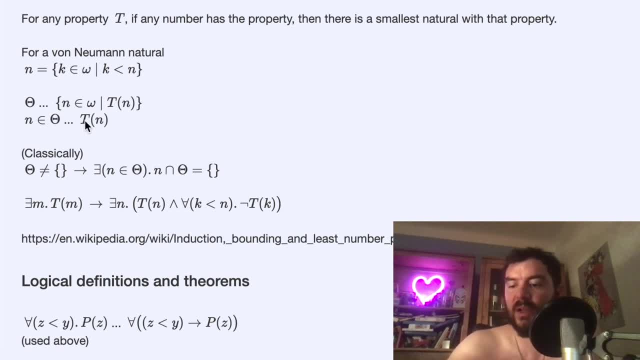 have this correspondence explicitly right: you have properties and you know you don't. if you're here in talking philosophy, you don't need to talk about natural numbers. just you can also say: you know, i don't know. nicolai is was born in vienna, and then you can talk about the property of. 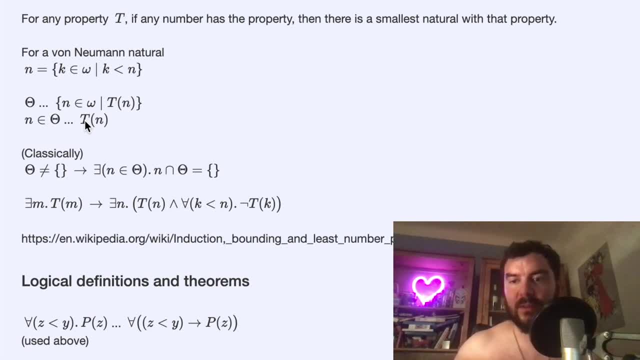 being born in vienna, and you can talk about all, uh, entities, terms, which are born in vienna, you know, or other viennese people talk about the class, and so, um, all the axioms that you might adopt for particular classes, namely the sets, um, let you express, then, statements about properties like: 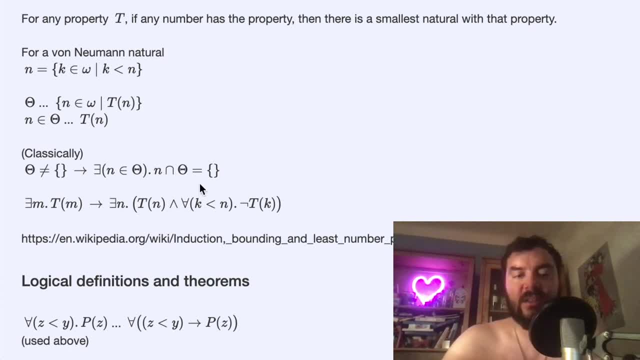 you know, being born in vienna, and so on and so forth. so here is the, the, the translation between the predicates: um, as wittgenstein had would have it, but he was also. i mean, it has been has been a decade since i read the book, but i'm i'm certain he talks about uh sets as well, ming in german. okay. 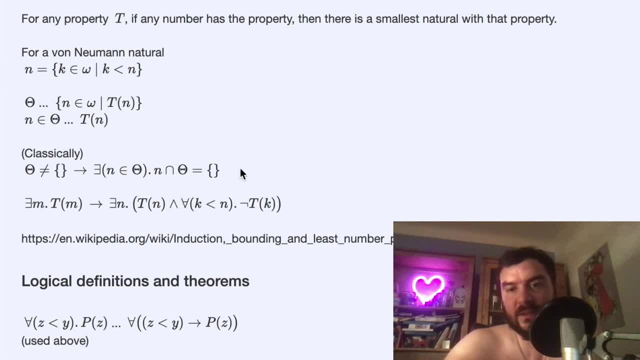 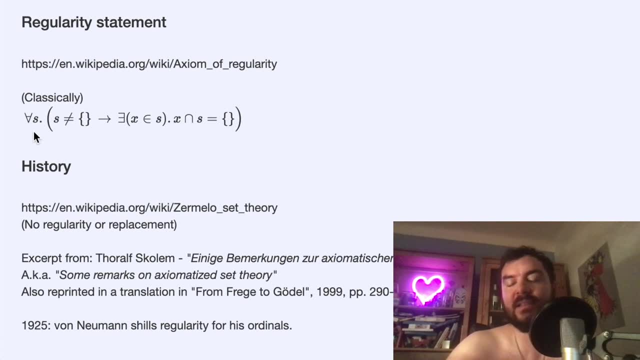 and um, yeah, clearly, you know, if you look at that statement, this is exactly um, this statement, right? so here this is uh, in, you know this, like the statement in the brackets anyway, the um, the set theoretical regularity axiom. if adopted as an axiom, then you adopt it for all sets, meaning for all classes, which. 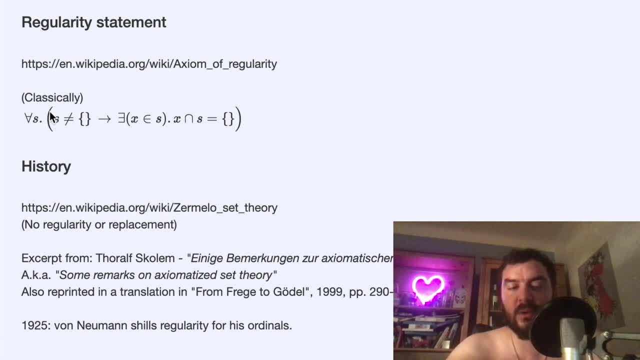 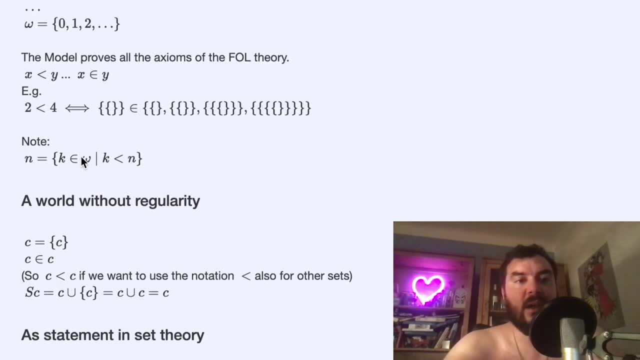 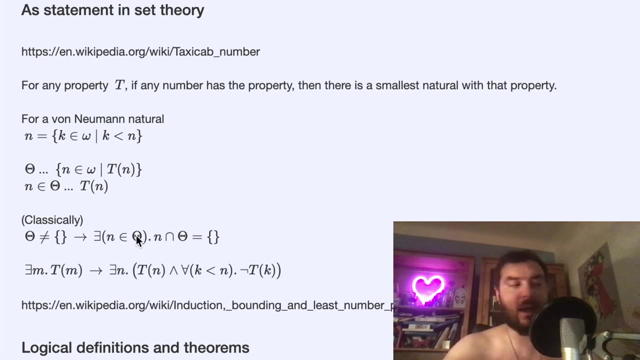 are sets, if you want. and then it says it for all sets holds. this statement. this statement here is exactly the has exactly the same shape as the one i motivated here for a particular set right, but also by induction or by the equivalent minimality principle that we are going to see the consequences. 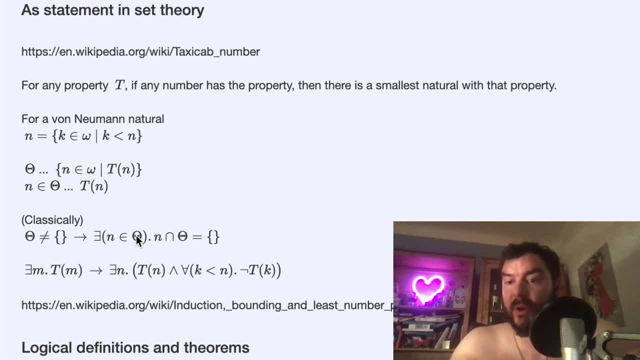 of this works for all, uh predicates, in fact. so this is, this is a weak and strong at the same time is strong in a sense that actually we are going to postulate it for all predicates, not just the ones which are made into set by some set theory. but of course, it is a weaker statement. 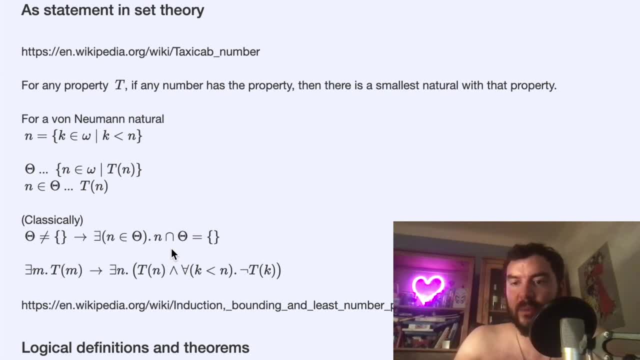 in the sense that here i'm just talking about it in in terms of the natural numbers and the natural um, much sort of smaller domain to talk about um, at least the standard model, than set theory. okay, so not to confuse you here, but i want to highlight that this is, quote, unquote, the same principle. it's 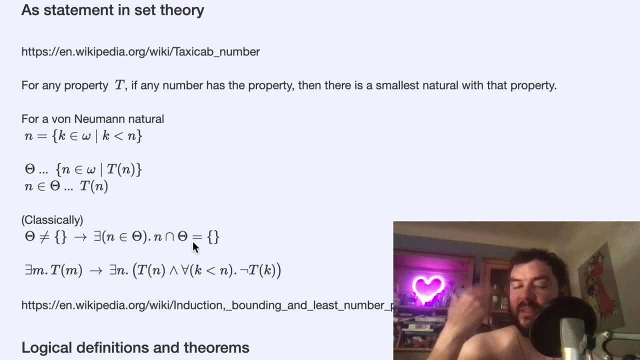 it's both a minimality statement, um, but the set theoretical one is more complicated to interpret because sets are not a priori linearly ordered objects, right as the natural numbers are. here we have the successor operation that reaches all numbers in the initial segment and this is not um available for sets in general. and 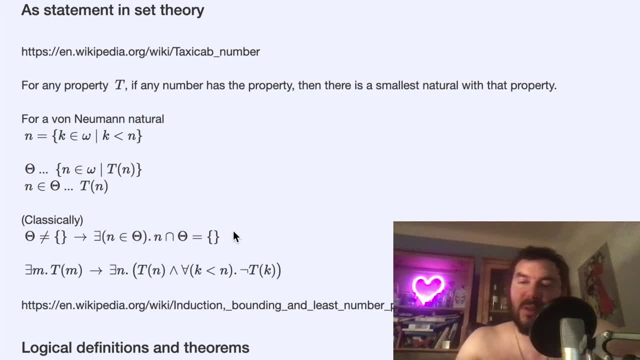 that's why the regularity axiom is a little bit more obscure, but people like to express it also as minimality statement, because then, um, firstly they, then you, just you know, need to invoke minimality, and then, um, you have a better idea of what sort of object the existence of is postulated with the axiom. 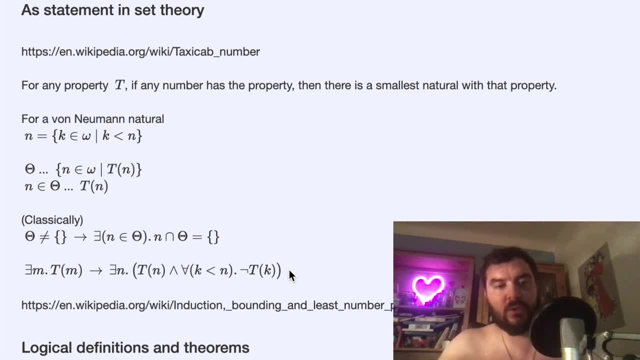 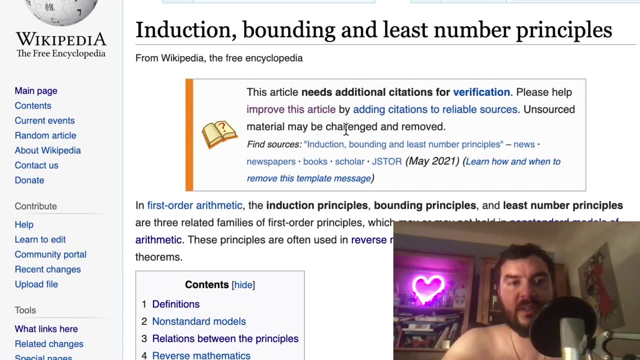 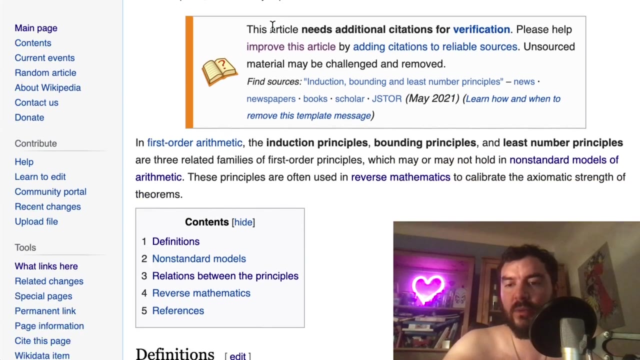 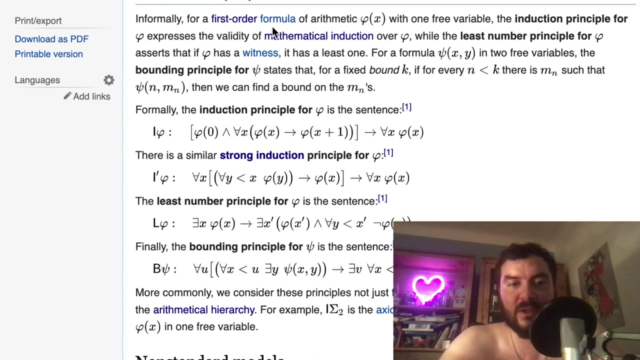 okay, so, um, i will also just show you the, the wikipedia page that i have, uh, sited here. so this is um induction, bounding and least number principles. i think this is probably written by somebody who is into reverse mathematics, because it's a super formal statement, like page compared to some other introductory arithmetic pages, uh, and you have here a bunch of 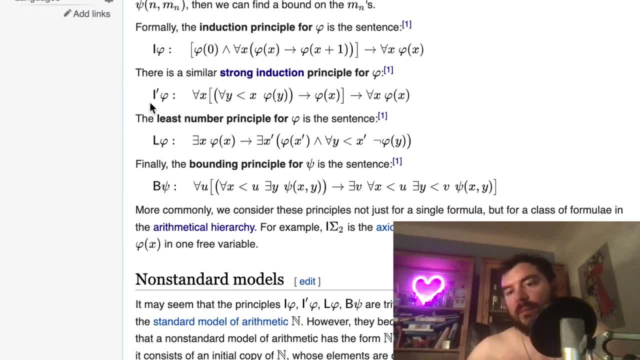 uh statements which are which, if you're in the context of piano arithmetic, should be equivalent to each other, although in the context where they're discussed here, with reverse mathematics, with second order arithmetics which are sort of weaker, they are not really the same because you also adopt them only for. 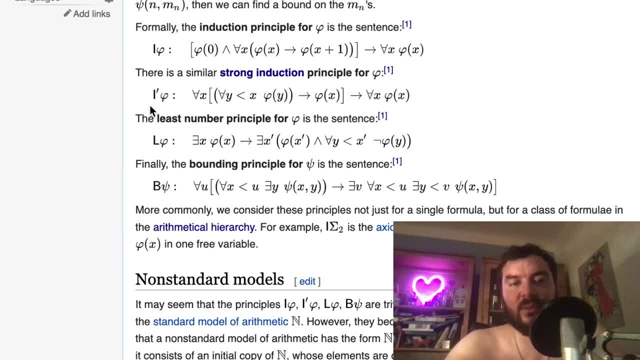 certain predicates and so on. okay, these are details on the side. i don't want to confuse it too much, but this is the one we're discussing here. this is the one which i have just written down for a particular t, the schema, and here you have the induction principles: um, if, um. 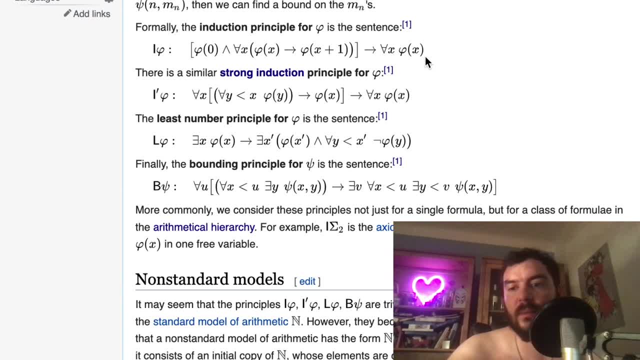 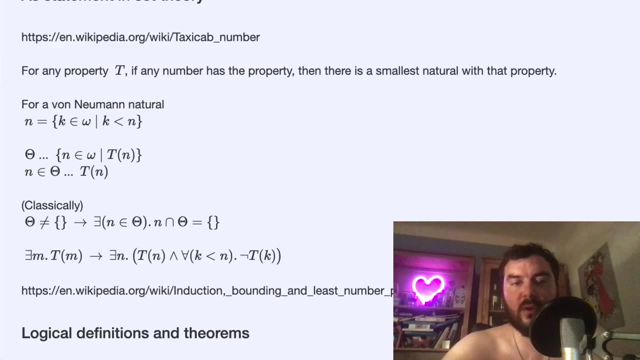 if you don't- um, you know, if you, if you don't know everything of these things by heart, you might want to look it up now because we're going to make use of those, but i will also restate them again. okay, so i've written down some of the principles that i'm going to make use of to 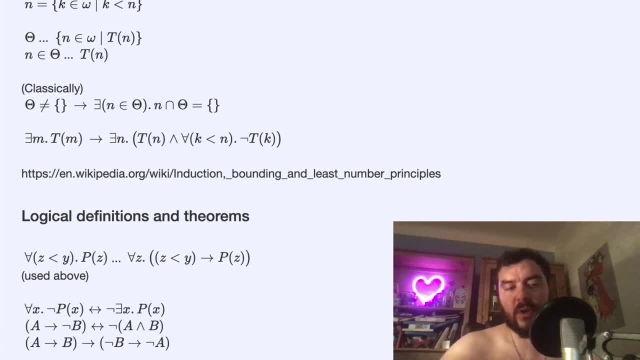 prove the things that we want to prove. um, the first is just the definition of what i really mean with this bounded quantification. right, if i say for all z smaller than y and something something, then what i really mean is this: for all z if they are smaller than something something. 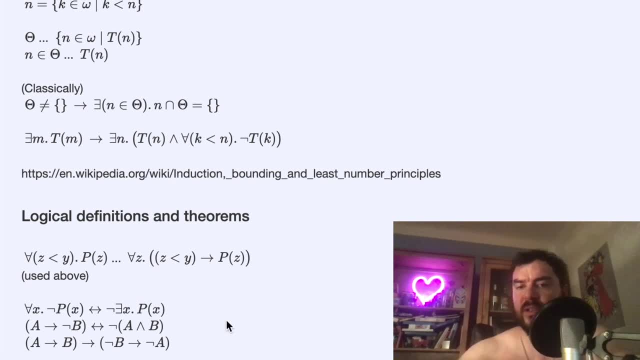 and below you see some equivalences and implications that i'm going to make use of. you know, if you talk about arithmetic, it's very easy just to stay constructive, and that's what i'm going to do. i will be explicit if i use the excluded middle. 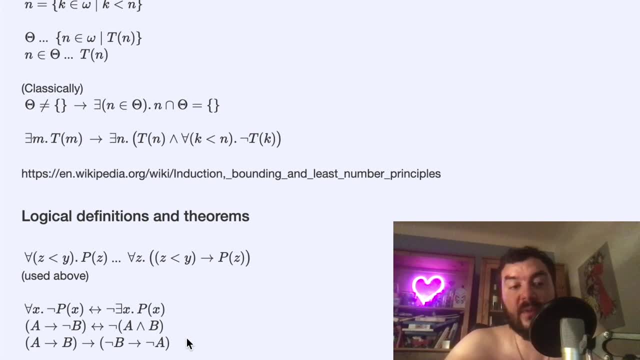 um. here we have uh, constructively valid implications and equivalences. so the first one says that if uh, for all, x, um, something does not hold, then this is equivalent to saying that there does not exist any element which validates it. um, then um. here a statement for conjunction. 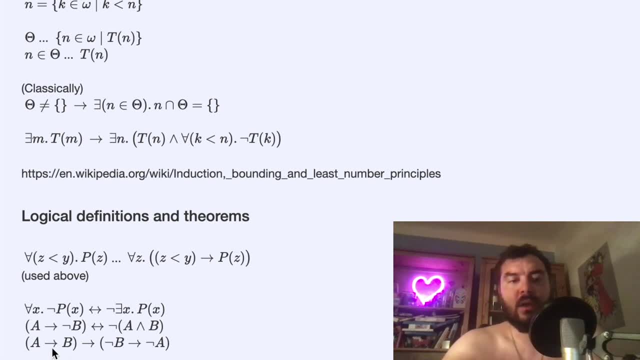 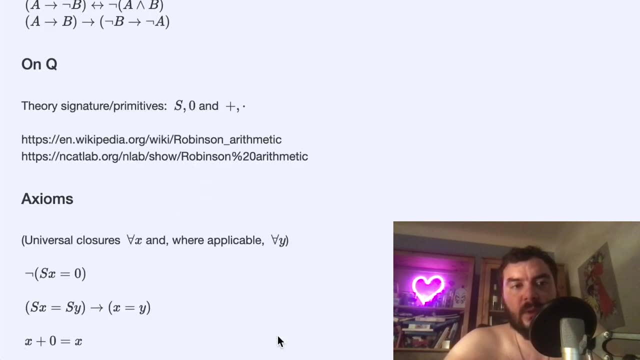 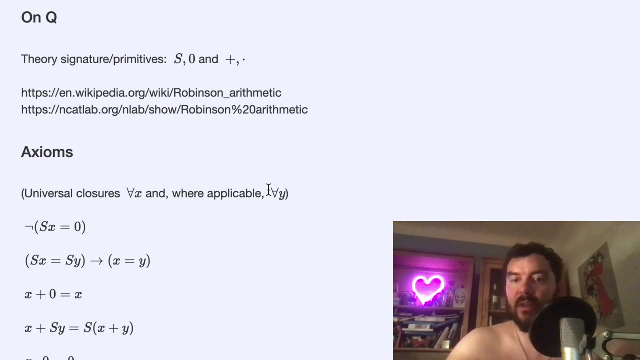 to represent it in terms of implication, and then, uh, the um contraposition, of course. okay, so um, let's get a little bit more juicy. so now we are going to introduce the theory of robinson arithmetic and, in a word, this is really just piano arithmetic, without induction and instead of 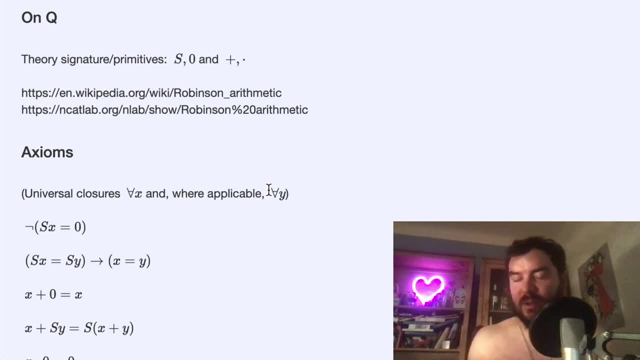 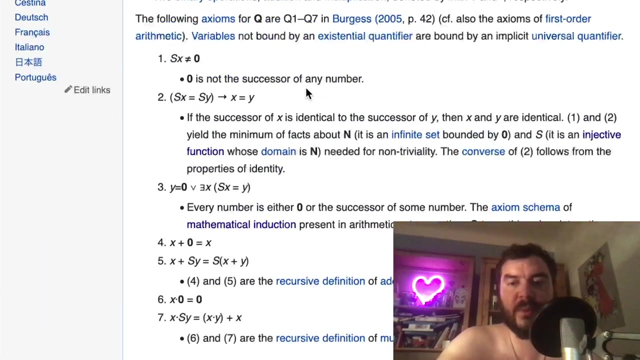 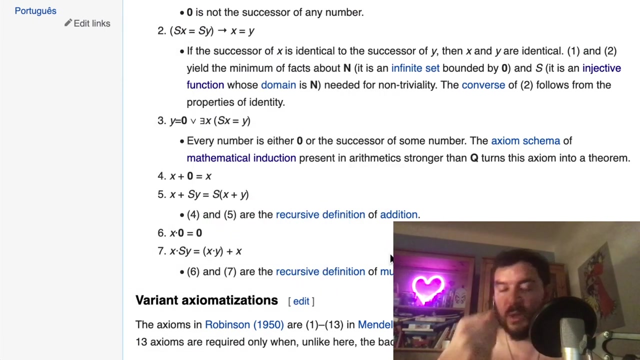 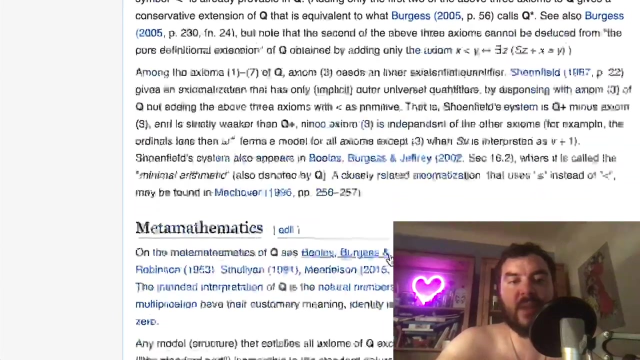 induction one stronger quotes and quotes. axiom is added, namely that every number has a predecessor. so if you are interested you can jump to the wikipedia page, for example on robinson arithmetic ob jalرة. robinson gives you more hints. so for example, for varicker you'll find various form of variations. 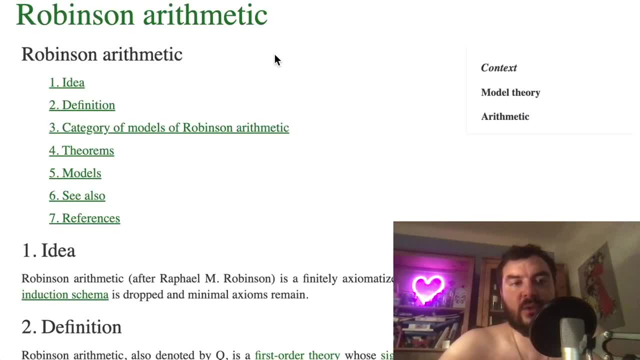 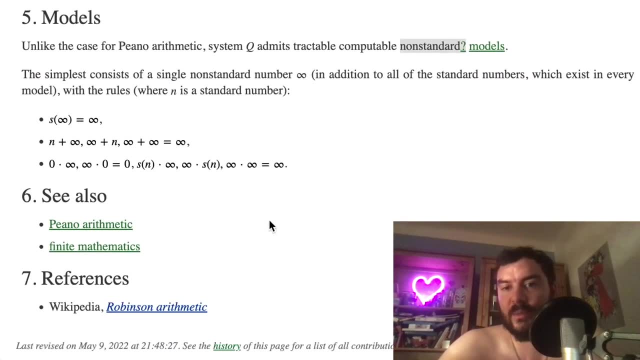 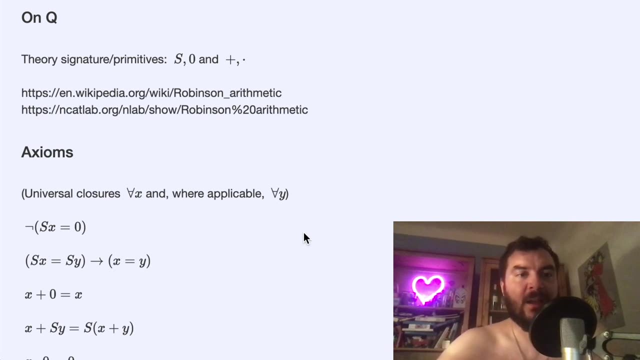 like the workkeeper of enlightenment, which is is generally a falling nine, everyone's own website that we are interested in and we're going to discuss it in a second. you don't have to press pause. so the theory, like piano arithmetic, has a signature which particular, in particular, contains the successor operation. this is a 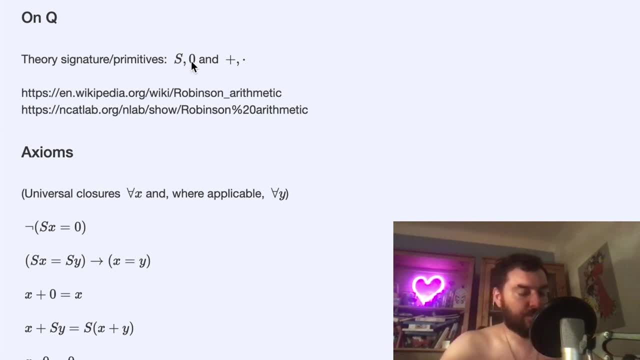 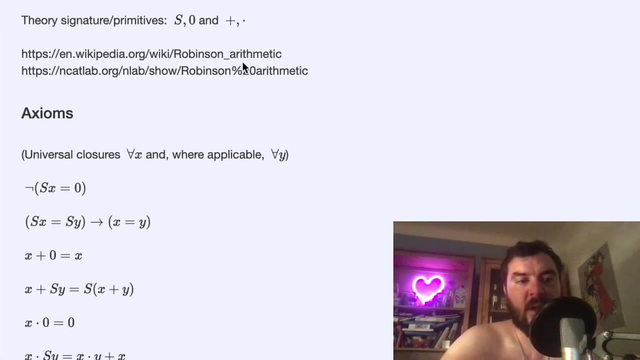 primitive in this first order theory: a constant symbol 0, and then these arithmetic operations that the axioms also talks about and clarifies the relation of this function symbols to each other. and then here are the axioms. if I have your letters X and Y, then whatever letter is in the axiom, you. 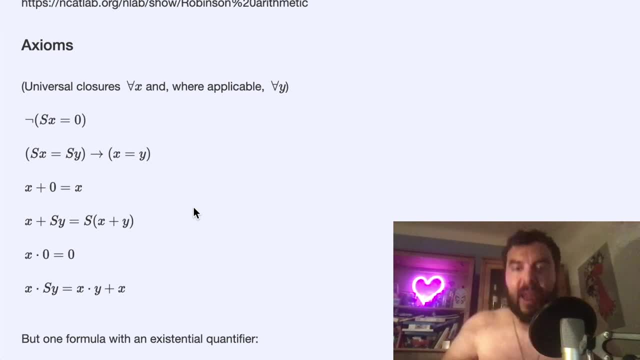 imagine a universal quantification before that, right for all X holes, so and so this is just for convenience in this case. you know, if you don't talk about universal algebra, that is really just in convenience, so I, I will just. you know, if you don't talk about universal algebra, that is really just in convenience, so I, I will just. 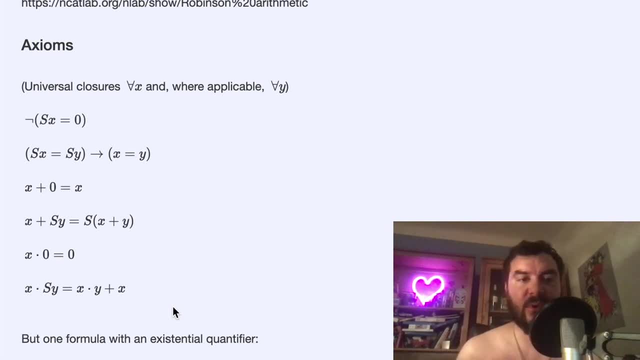 for the sake of it. go through the six axioms here. the first says that it's not the case that the success of any number is zero. sounds reasonable enough. the second axiom says that if the success of some number is the same as the success of another, then this already means that the numbers were the same. 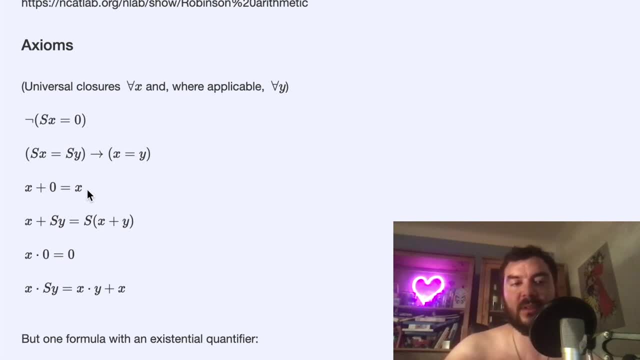 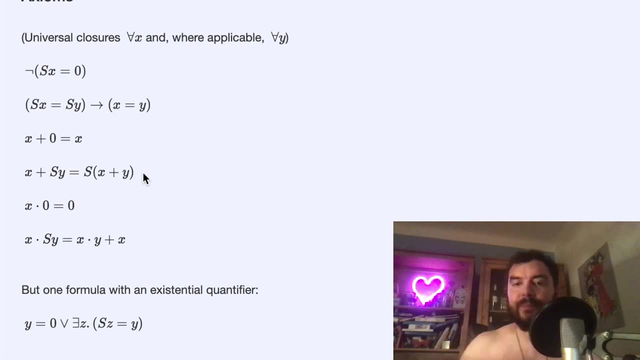 then any number plus zero is this number itself. then you know one of the characteristics of the success are right, a successor is just adding plus one. and if edition has the usual in our community properties and so on, then it doesn't really matter where you add one. you can read it like that, you can. 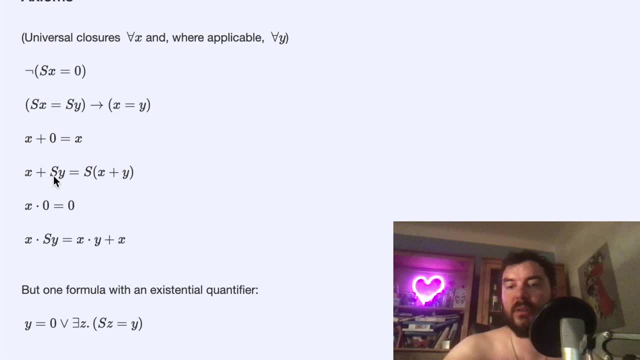 also read it as a way of computing addition and so on, sorry, okay. and then x multiplied by zero, zero, and then a relation between addition, successor and multiplication. okay, and piano axioms would have now also the induction axiom, which we are going to see in a second as well. but this theory 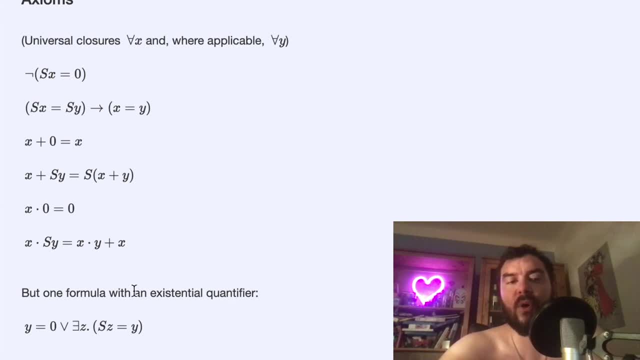 does not have induction, but instead it has one formula which is also implied by induction actually, but here we don't have reduction. we cannot prove it, so we adopt it as an axiom to get another arithmetic which is sort of like piano arithmetic. and so it says that four numbers 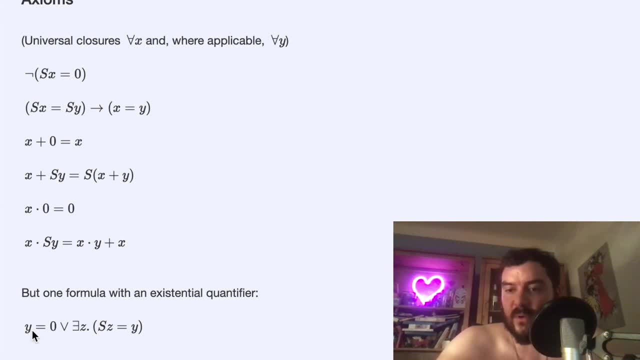 y holds: either the number is the first number zero, or there exists a number such that the successor of that number is y, right, so this says every number is either the number zero or it has a predecessor. you know, if you call the number predecessor in the usual sense, this is a statement. 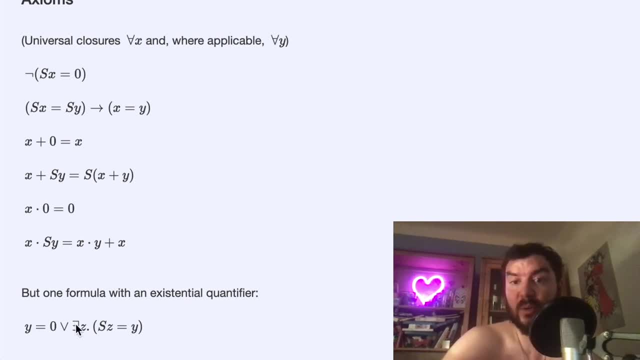 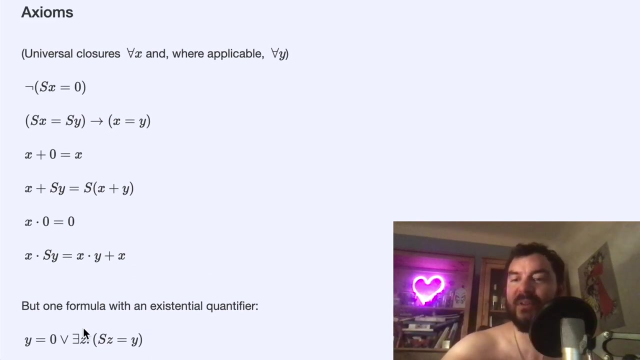 of predecessor. existence is an existence statement. you have an existential quantifier and you will notice that all the axioms so far are actually super simple. they are only only a few universal quantifiers and the symbols and the signature of the theory. this is actually. i mean, it's so like compared to other math, it's. 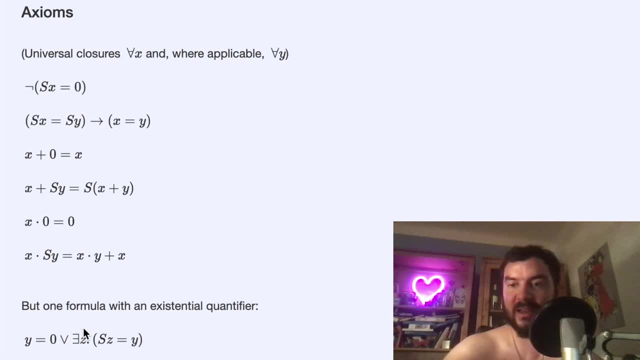 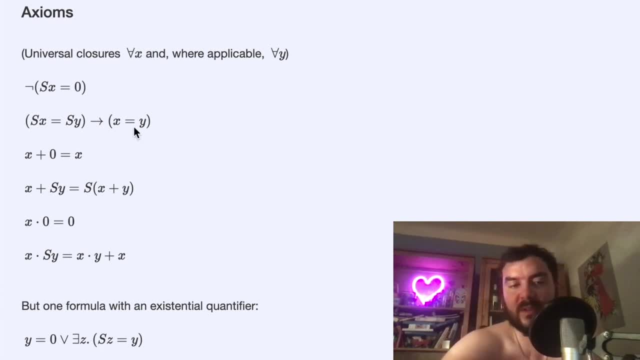 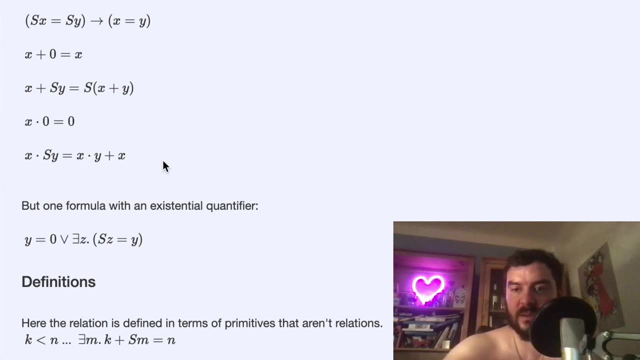 this axiom is not provable from those statements, for example: okay, so, um, this is the usual way of setting up also piano arithmetic with the standard signature, and then we can define, for example, the order relation like: so you should think about that, it makes sense because it will play a role. 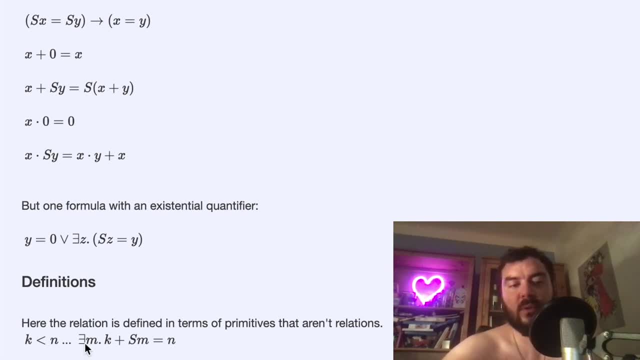 so, um, you say that a number, uh k, is smaller than number n. if there exists a number such that k plus the successor of the number is n, right, so i mean, how do? how to read that? so, firstly, the success of being here with the m is sort of a trick to excluding adding zero right like now i'm. 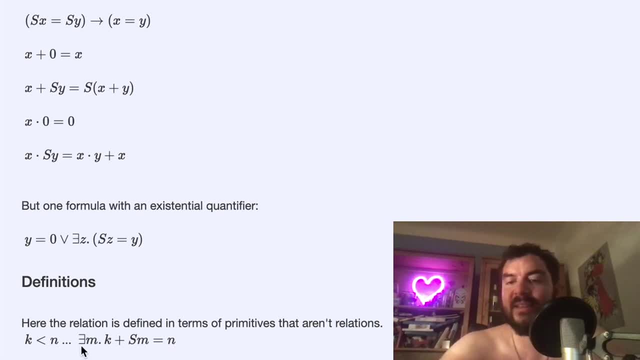 speaking a little bit more semantically, but this says there exists some number and such that k plus and then the successor of a number, This together is n. Again, semantically speaking, the smallest number, 0, would be allowed here, but then this says k plus. 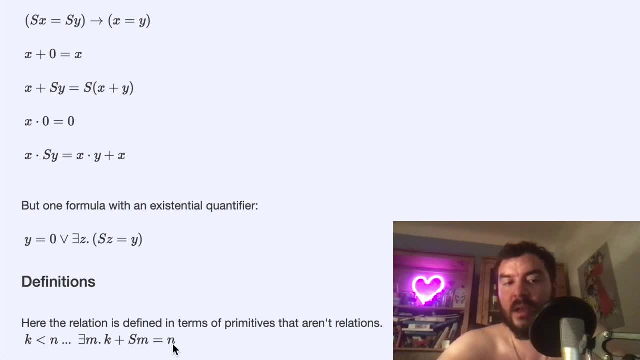 successor of 0 is n. so k plus 1 is n right. If there's any number m bigger than 0, let's say 5, then that would say k plus 6 is n right. So this characterizes that whatever m is, n is actually like in terms of the 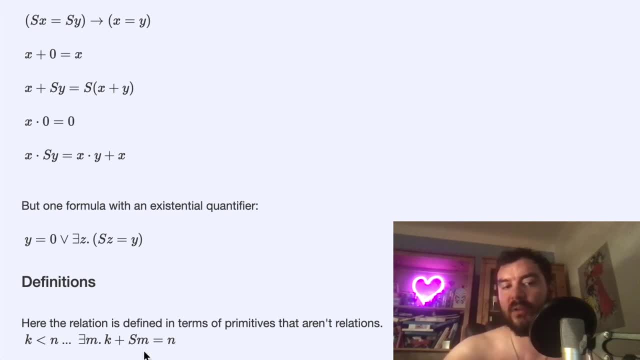 standard model, a bigger number, right? I mean, you should think about this for a second and validate in your head that it should make sense that this is a good definition of the smaller-than relationship. okay, Okay, yeah, I will do. 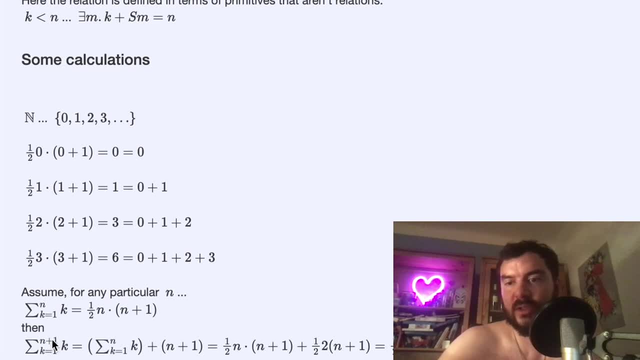 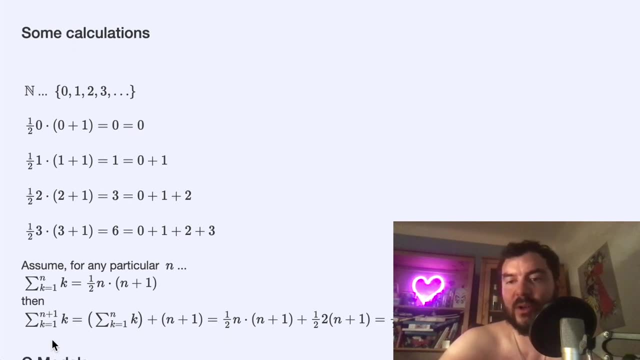 some calculations there because I will later show, when we adopt induction, what that, for example, means for what the language can prove right. I will not like say too much about that because I don't know if I get the rest of the video through in 50 minutes, but I 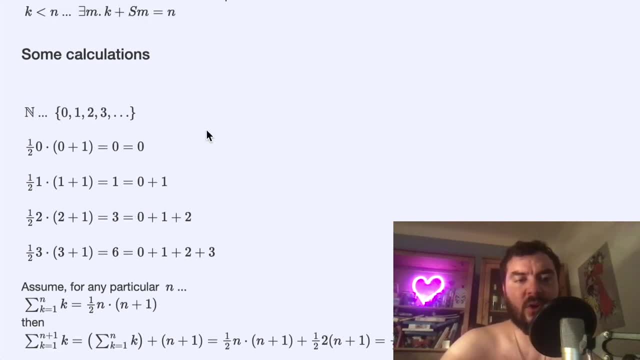 will try. So here's some calculations. right, I now denote the natural numbers as this collection. right? We're not in set theory. I don't want to talk about the set of natural numbers as an object in my theory. I want to talk about the. 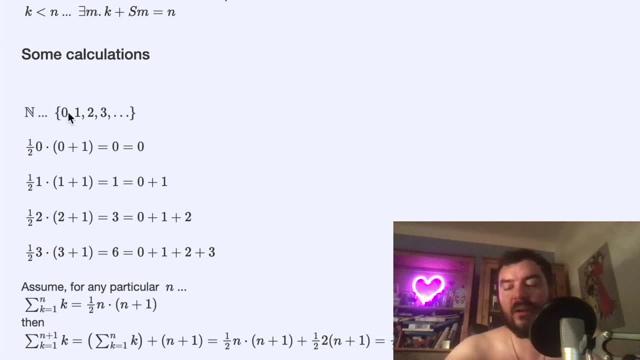 domain And for any number that you can give me here, the standard natural numbers, it turns out that this peculiar relationship holds right. So if let's say, division without rest, if you multiply the 0 with 0 plus 1, and then divide by 2,, you get 0, and this is just. 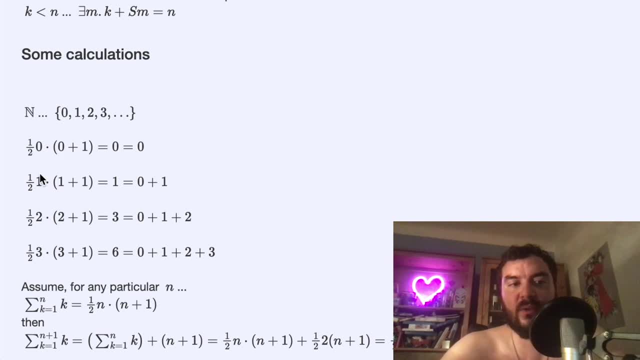 0. If you do the same thing, but instead of 0 here you use 1, then you get 1 times 2 divided by 2, with the rest is 1, and this happens to be 0 plus 1.. And if you go, 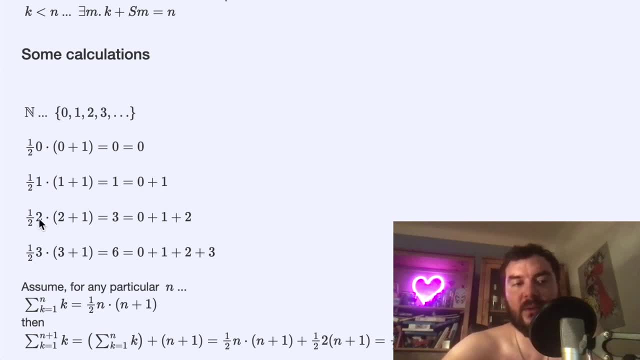 on and plug in something different, then you get: 2 times 3 is 6, divided by 2, it happens to be 3, and this is this. So you get this peculiar pattern right. And so for any number in the Robinson Arithmetic, if you give me any number, for example, 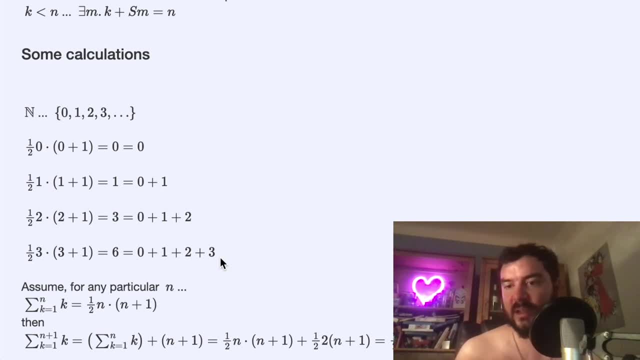 9000, and I have the time I can write down this and validate this and we'll like Meta- aiii. Mathematically, you know, I make the texture that will actually work, will like actually turn out to work, And then more We can speak about some. 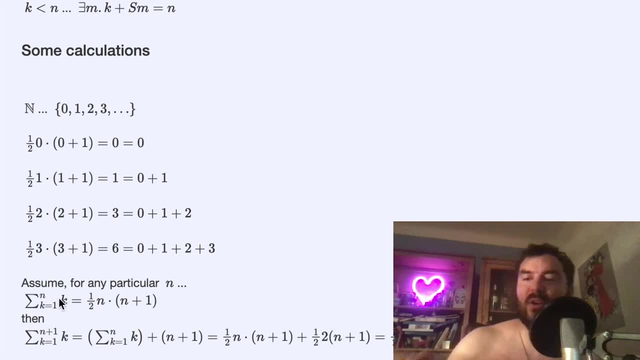 implications, right, For example, of course you know you would have to define recursive functions- blah, blah, blah in these languages- and it's possible to define this finite sum. And so let's make the following observation: Given any particular n and sum over the numbers k, this is: 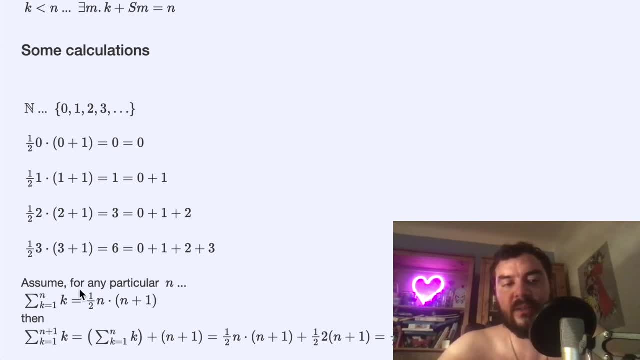 basically the right hand side here. assuming that this turns out to be this expression, this multiplication which corresponds to this, then what actually does happen if I don't go to n, but n plus 1? well, I write this down here: this is just to n, but then one step further. this is this thing, and then I can use. 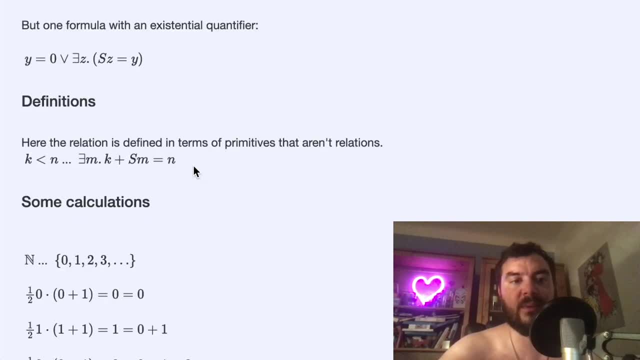 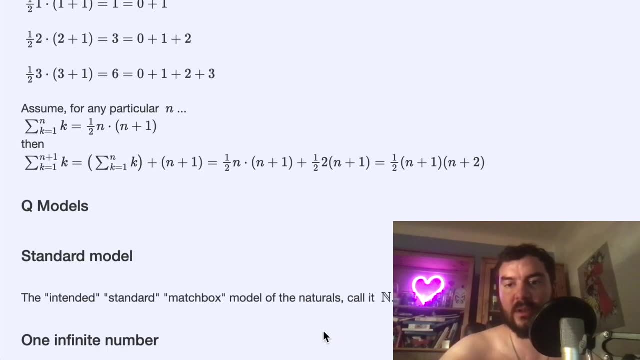 their, you know, normal arithmetic, which is also implied by but the axioms here, and on some rewriting it turns then out the upsala. it doesn't out that this is actually of this shape and this is again then of the shape. so this is an some observation that can make. I can you know for any particular number. I can, can do. 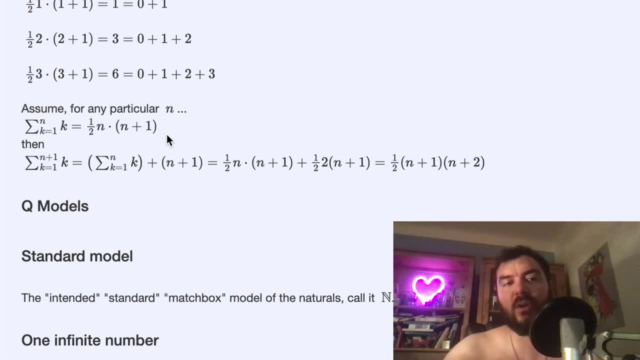 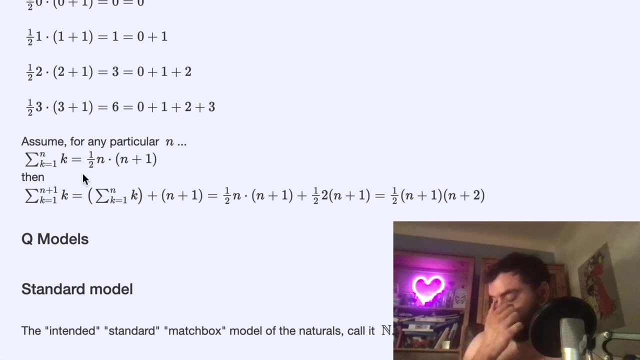 this thing. okay, so now you know, I know that for the first few numbers this worked, and I know this, I mean, you recognize it. this is sort of the induction step, but sin, since my theory does not have an induction axiom. it's not the case that now I cannot conclude that this relation 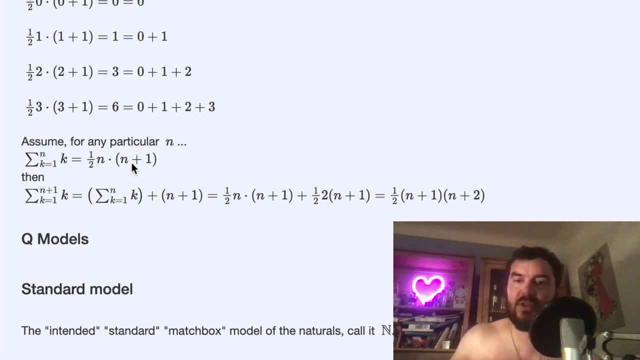 always holds right. this is exactly what the axiom of induction in enables me to do. it enables me to make a statement with a universal quantifier upfront. I can maybe evaluate this, this stuff, for every number, but I cannot make a claim inside of the language that this holds for all numbers, right? this is the power. 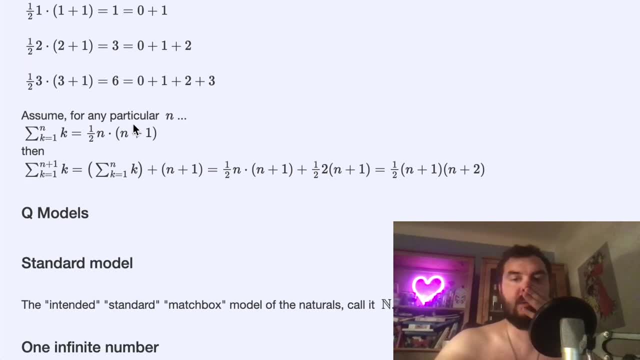 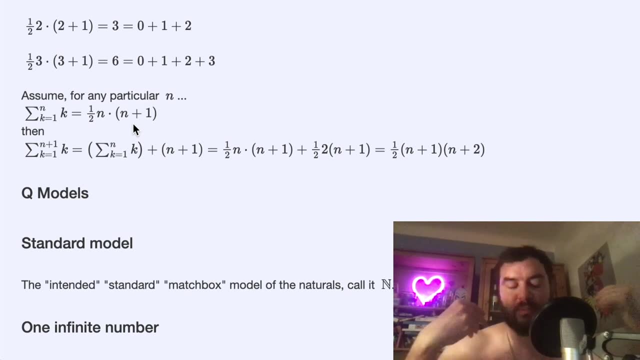 sort of the induction axiom. okay, so we're going to get to induction later, but here now some of the cool parts which might now explain some of the explain the ways in which the regularity axiom or here in this case, then this number principle, which is the corresponding principle, rules out in the 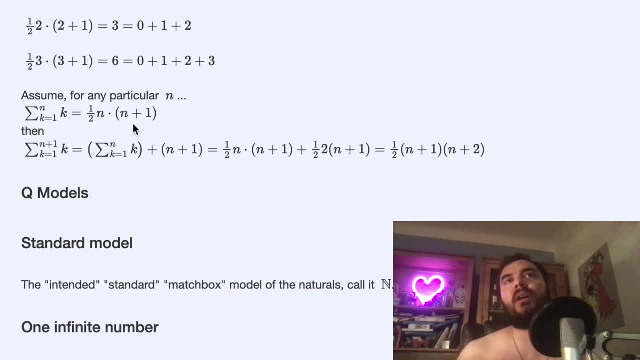 set theory case, self membership and in the you know predicate, speak, speak case- predicates having themselves as property right. this is sort of what was ruled out when Norman threw it out. so can he can do his ordinal stuff. he wants induction and have a simple set theory. but this is basically what is ruled out by adopting 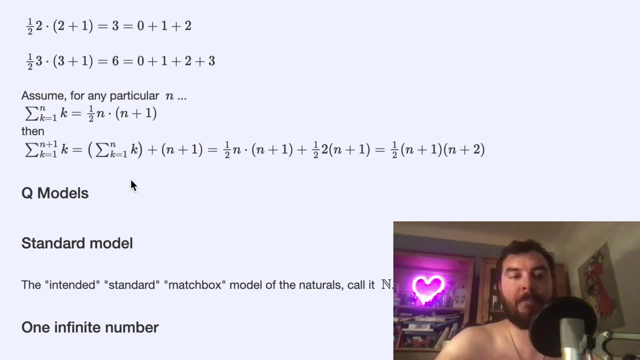 this, this sort of regularity or minimality claims. so we're going to discuss a non-solid model of Q. I will mention a few and this will be fun, and then, at the end, I will also mention non-solid models of piano arithmetic, which might be maybe more surprising. 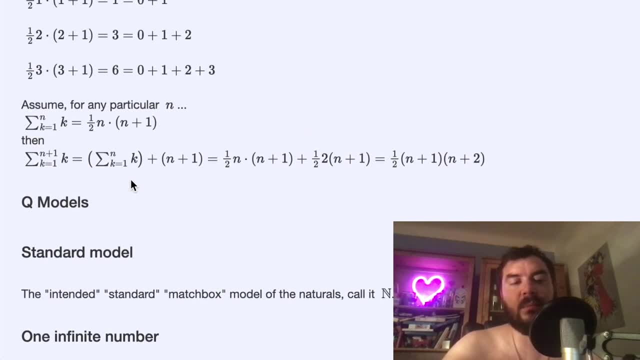 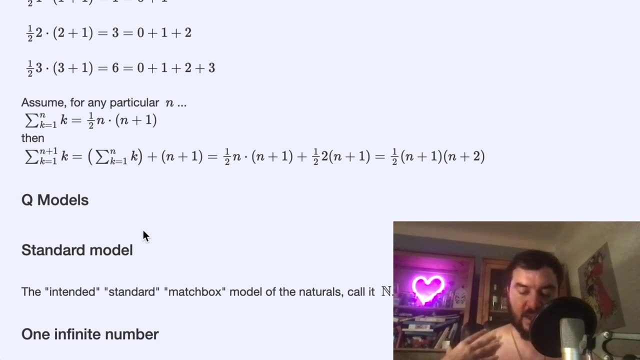 okay, so models of Q. well, the first model, that is clear, is the standard model of initial numbers and I call it here sort of matchbox num model. this is like when you say, when numbers let's instead of matchbox, let's say backs of stones, right, you have a bag of stones with before a bag for stones in. 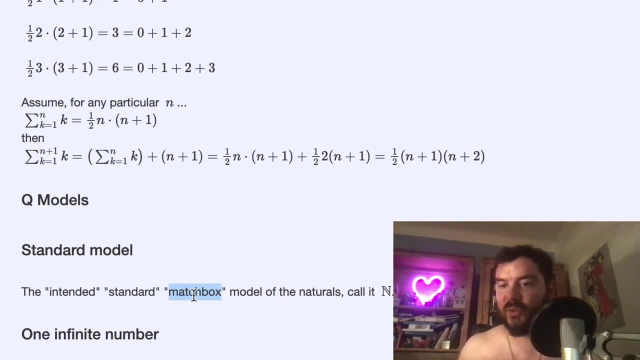 it and a bag with seven stones in it, and then you can each define an operation of addition by making a new bag and putting the stones from both of the bags in it, and then you get what did I say: 4 and 7- and you get a bag with 11 stones. 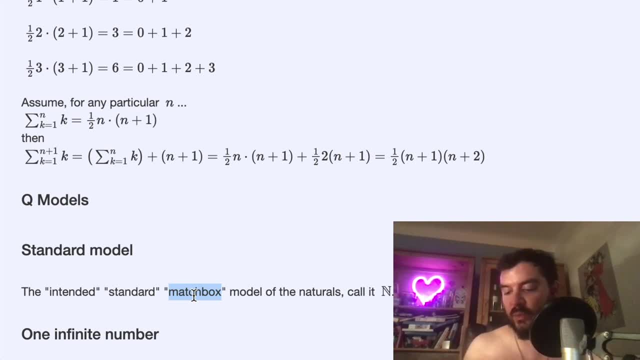 in it and thereby moved from two numbers to a third number. you added them and, more to the point, the standard model can be then represented, for example, with the Neumann model in a set theory, as we did. or you think about recursive rewriting with strokes on paper that capture. 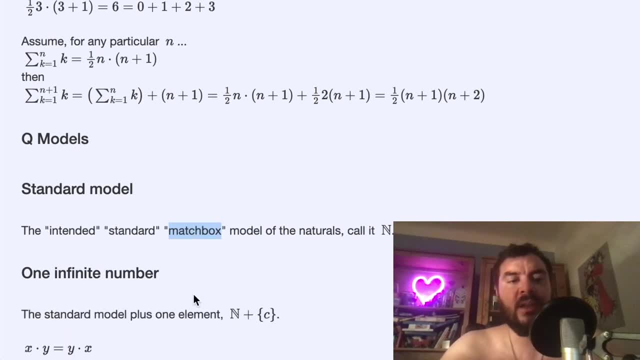 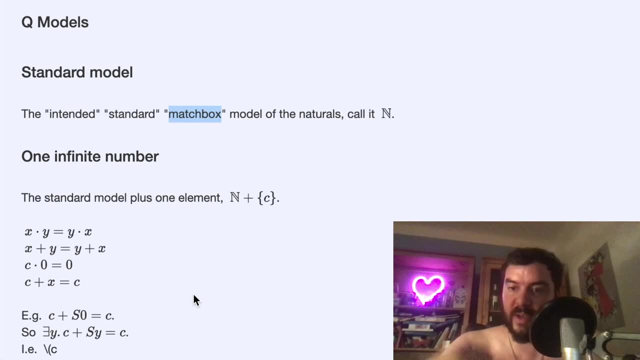 sort of this standard model right. But what we can do now- in Robinson arithmetic as opposed to piano arithmetic the situation will change in a certain way, as we will discuss later- is what you can do is now, since you don't have the induction axiom, it's actually compatible. 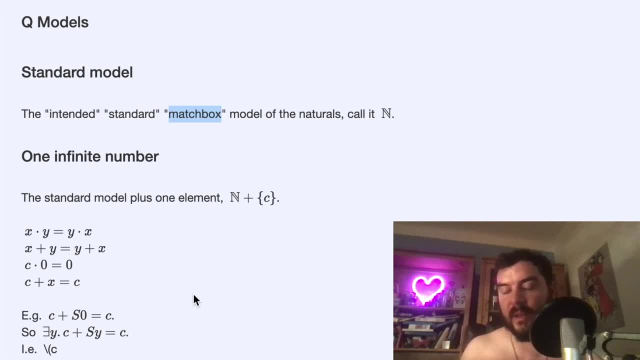 to a standard model right, So you can do this in a standard model right, So you can add one more element. we call it infinite element. if you want, I call it also C, similar to what I did already before when I discussed sets and this. you add this and you impose. 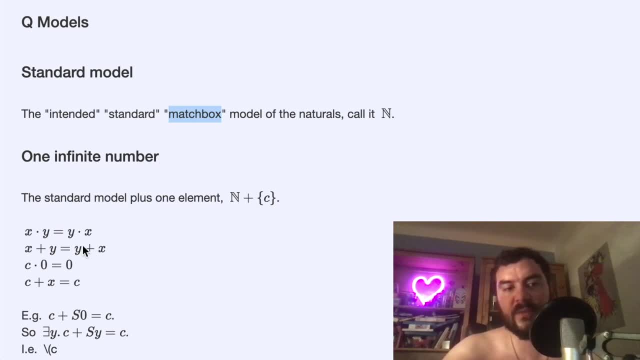 some arithmetic rules, right? So okay, the first things are just commutativity of the numbers, as we already had them, and then you say that C plus 0, C times 0 is 0, I mean, this is demanded by. 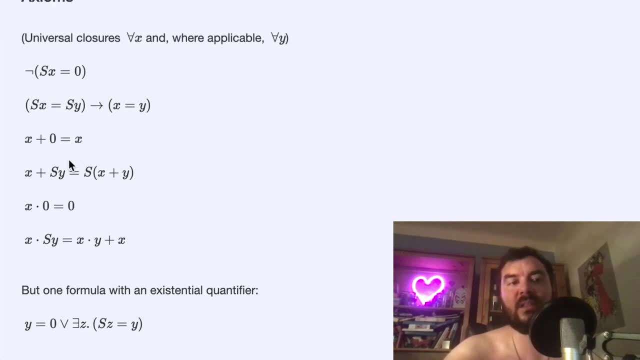 the axioms here as well. right, this note: these are the axioms for the arithmetic you must hold for all numbers. and by all numbers we don't just mean, we don't mean a particular model, right, we don't mean the standard natural numbers. the theory, the syntactic theory, does not know about the standard. 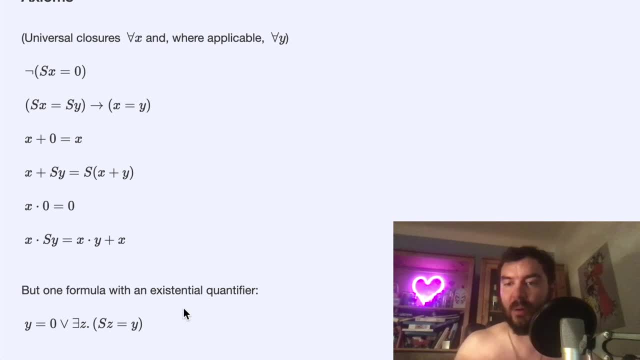 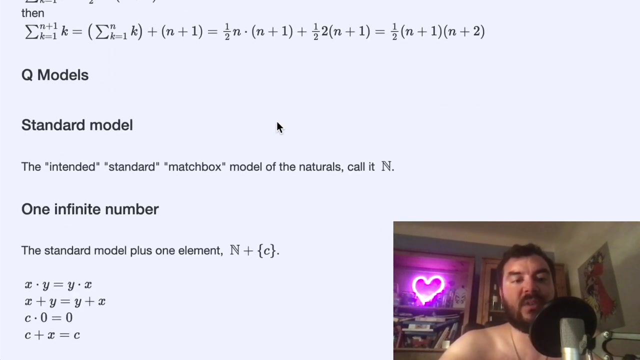 natural numbers. the theory is a syntactic construct that you can interpret and you can read something into it, but the theory itself does not know you know how many numbers it has, or or if it has numbers which are sort of special, as we have in this model now. so you have this number. 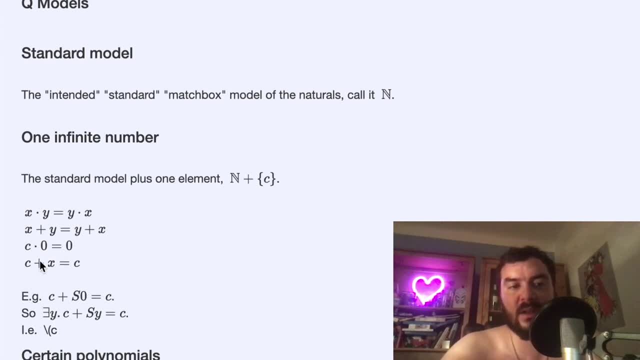 to be a model of the theory we need that the c multiplied by zero is zero, and so we impose this. and we also say that c plus x is c again right for any x right. so c plus 9001 is c again, or c plus c is c again right. in this sense we can call it infinite number, because it behaves like 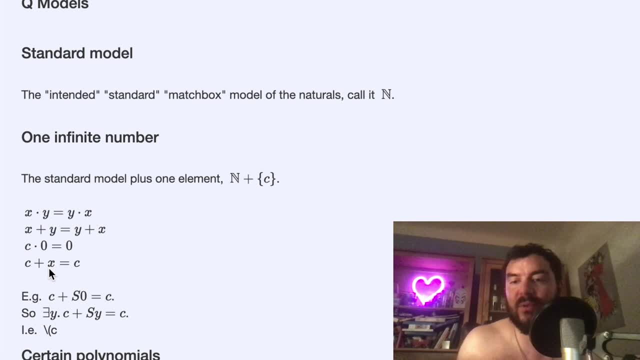 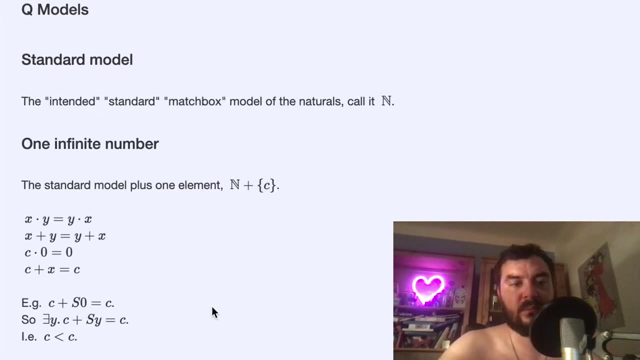 like an infinite number number, as you might expect from an infinite number. if you do um- and here my latte is broken, okay, um, yeah, so, um, some consequences. um, as i said, c plus, for example, one is c. so this also means that there exists a y, such that c plus s of y is c. right, you mean y equals zero and you know any like any y like. 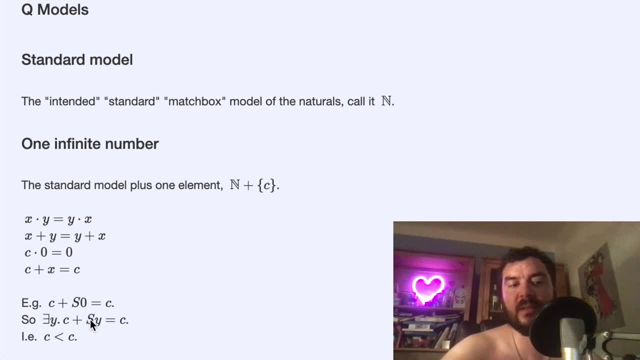 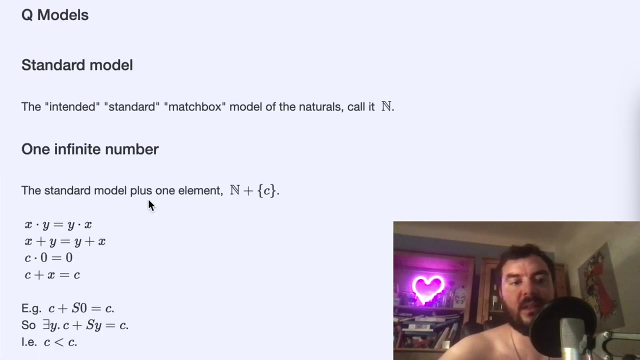 y being seven also would work like c plus. the success of seven is c plus eight would also be c um. so by definition of our smaller than relationship in the arithmetic theory, right, by definition here, this means that c is actually smaller than c, right? this is just a formal statement of this right. it's of course you. 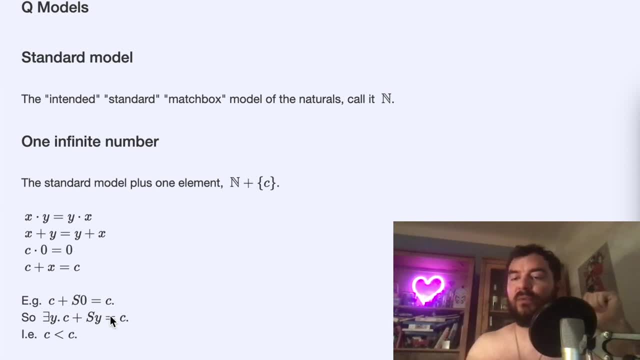 know, when we write down the smaller symbol, we don't have that in mind, but the theory does not rule out that this, this is possible. i mean it. it would rule out, as we will see with induction, but this weaker theory does not rule it out. so this theory actually does not rule out this model. 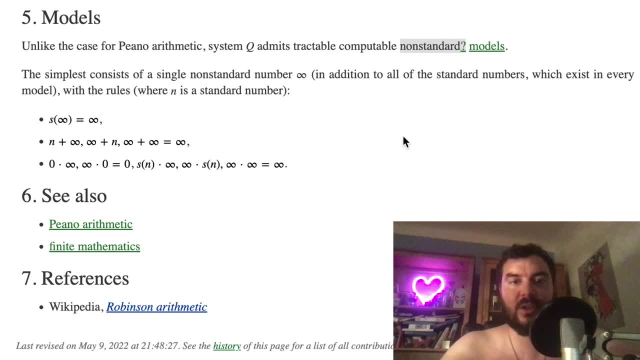 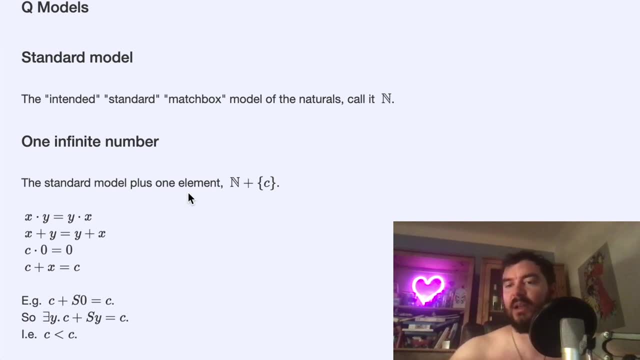 and um. so, by the way, this is also here shortly mentioned, explained in in on this page. so you see how, uh, removing axioms allows you to have different, more models than you had before. i mean, in a way, it makes sense, right? if you add constraints, then 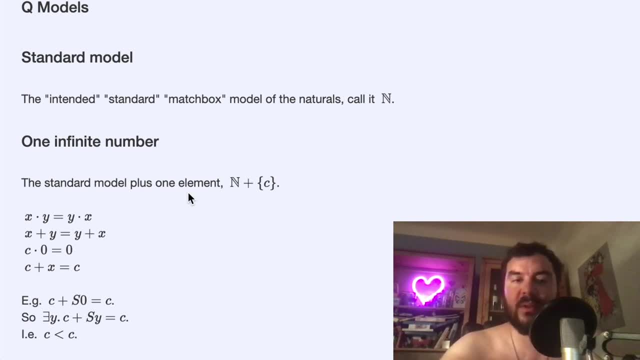 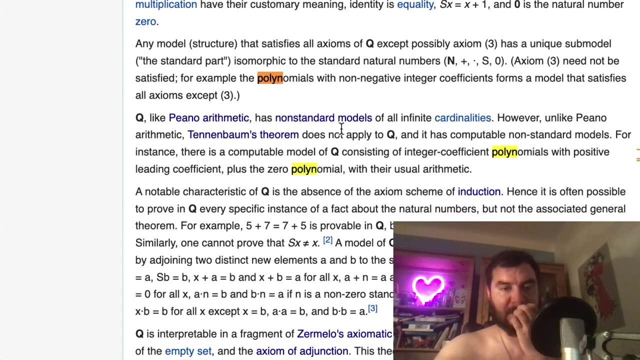 it might cut away models in the other direction. if you remove constraints, you get more models. yeah and uh. as mentioned in wikipedia, this is not the only funky model. uh, they mentioned that polynomials with non-negative integer coefficients uh form a model. so if you take polynomials with, 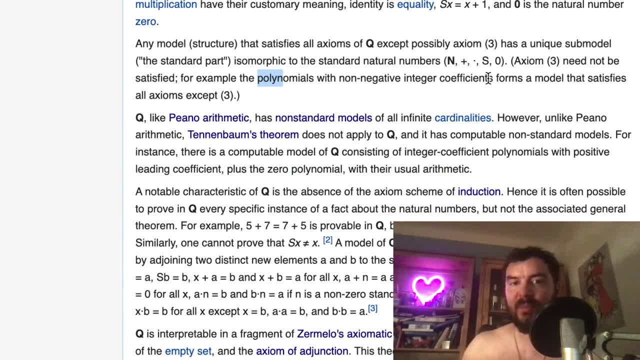 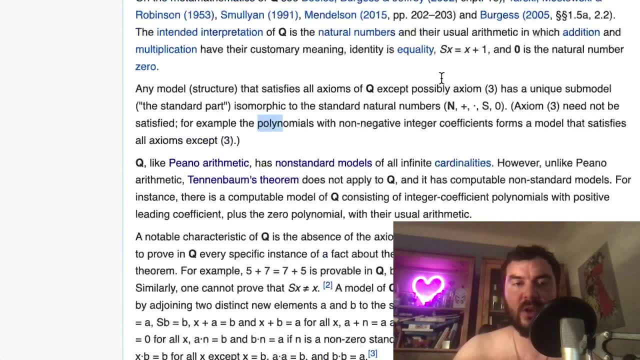 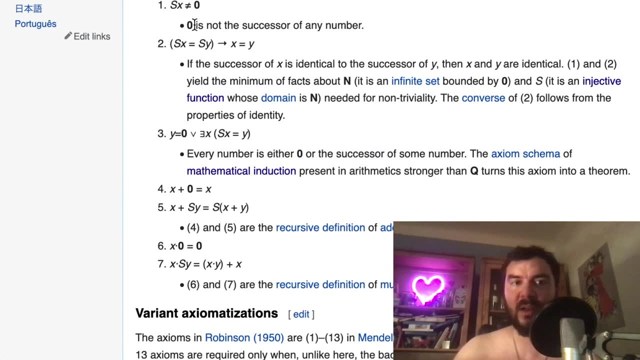 non-negative inter um integer coefficients, and, but also the zero, and this is basically the polynomial ring, or a subset of the polynomial ring, with uh integer coefficients. then all these, these axioms of the theory, these axioms, here, they are not broken. right, you can take a polynomial and and add. 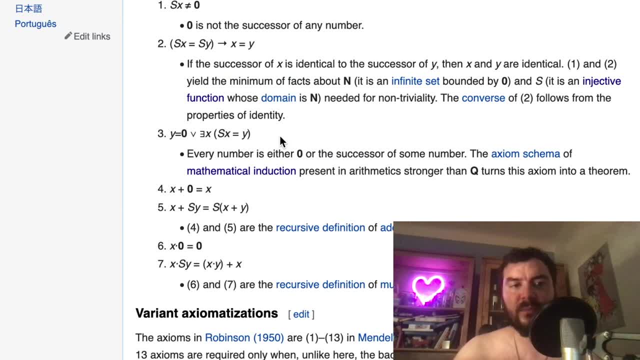 plus one and you get another polynomial and um, and all these rules, right? if you multiply a polynomial, it has the zero polynomial. look at a polynomial. what about the rest of the numbers? um, that's it. uh, we could add um in a way that, eventually, um, your end will don'tמש. 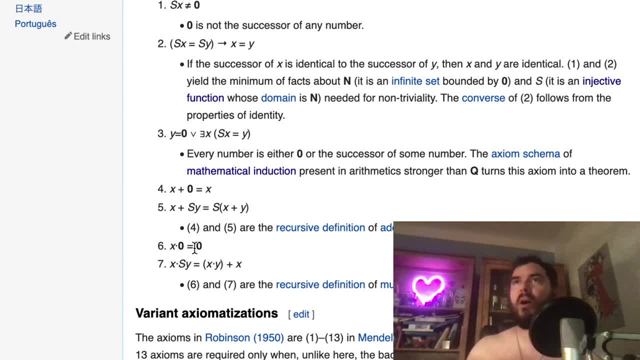 Hochschule Langmadant sporting for McClellan and Denver and our center aiser, there have one way of expressing things- then the existence of competing models, which might be very different. uh, might, uh, it can be interpreted and or can be argued for and might be argued for. 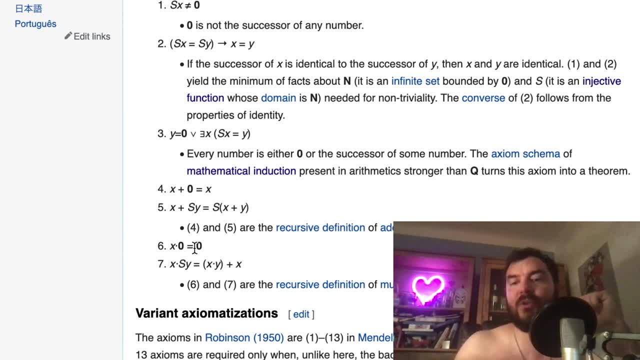 by some people to to imply that there are things we cannot capture as well, right, so just having the the formal mind um might suggest at least um that there is something that we cannot pin down, because it is then also the case that in piano arithmetic that there are non-standard models. 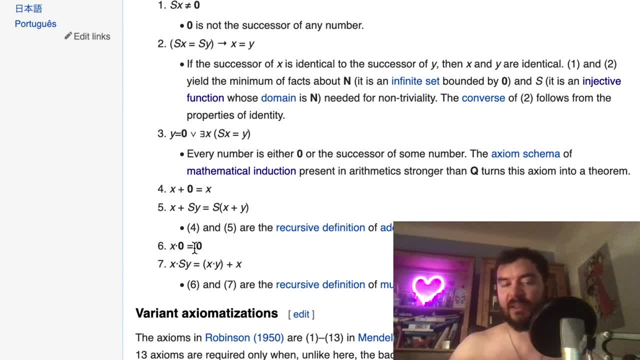 and indeed, um, you cannot fix the theory um in like you know, um in uh, this is the more complicated mathematical proofs. right, this is the, the, the formal logic and meta logic which happened a few years later. but in the end, uh, it goes as far and says: if you want to stick, 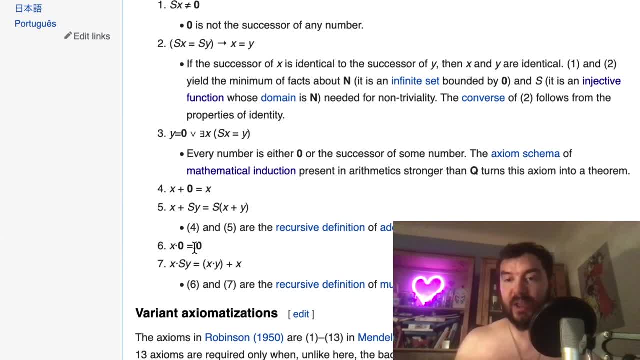 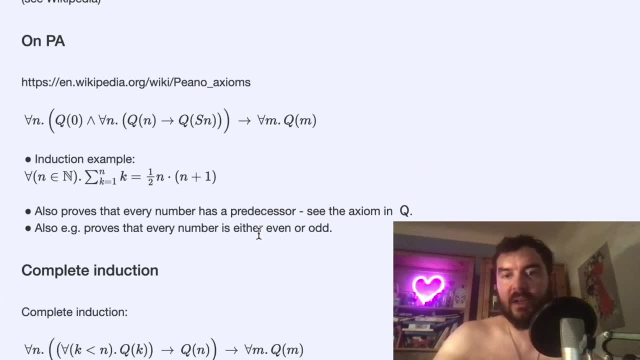 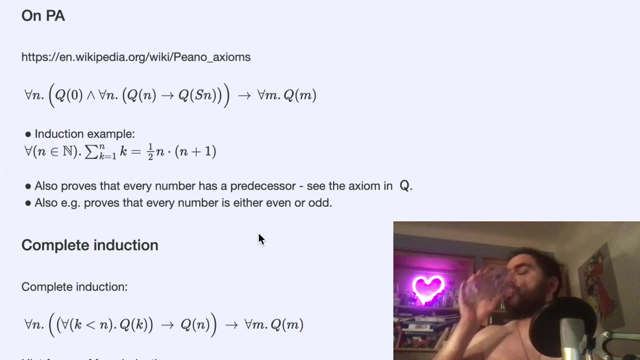 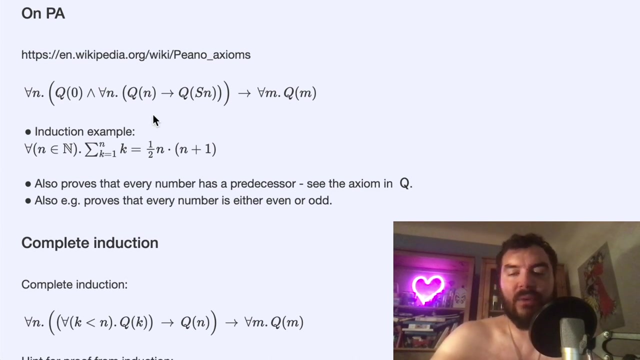 to the first order logic, then there is a lot of things which you cannot fix right, famously, okay, um, so okay then, uh, then let's finally. uh didn't write right, uh did it in under an hour, but uh, it might be worth to uh still like complete this here. so piano arithmetic aids an axiom. 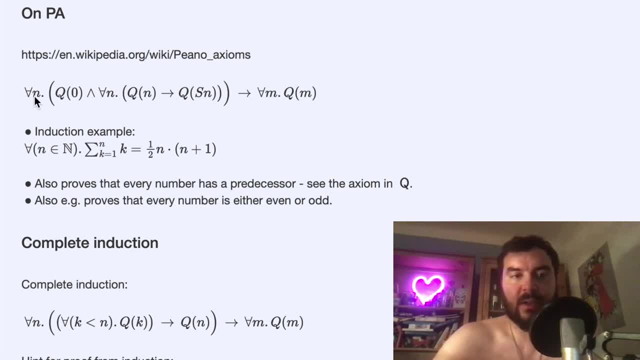 that for is, or an extreme schema that says: for every predictor, um. it tells you, if you do it this way, you can't ask an rentala as well, or an ant 작업, you get this q and if you tell them so in their executing and saying earlier q on x cross. 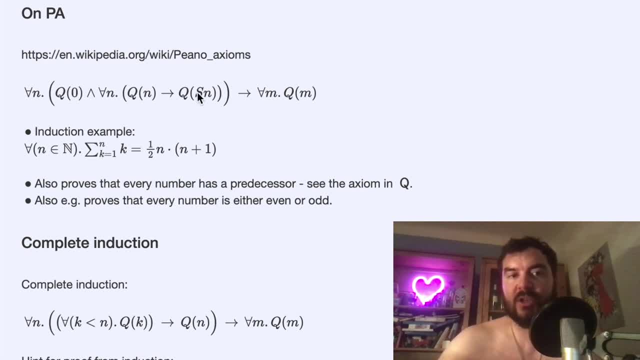 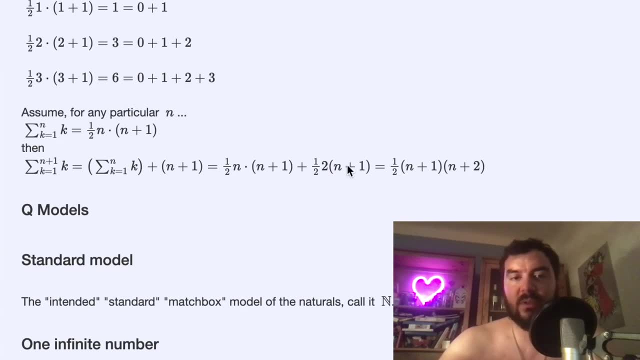 how many times do they get um q? you get this induction right. and so now, for example, going back to the induction example, we have validated force, a bunch of numbers- and we also have validated this implication right if it holds. so again, if it holds for this thing, then we have demonstrated with doing summer arithmetic. with some arithmetic that holds for the success. and then this axiom exactly says: okay, well, that done, well, because that worked. so it is true, it actually happens. and that Choose is true for all characters. it happens, even in the weavers. it works, but it would not route any terms matching化. um, however, the square, Paula, what we consider as Generally rules of algebra, which are small, are the видите for al finina''. 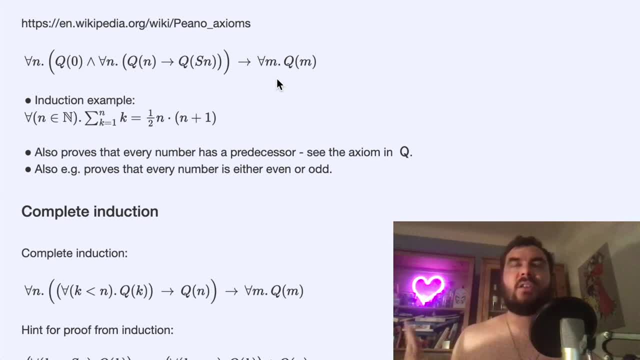 works for all numbers, right. and now the funny thing is, however, that piano arithmetic also has non-standard models. so, while we naturally think of the, the natural numbers, as this in terms of this standard model, you know, uh, matchbox and bags of stones, sort of objects- right, they are just these. 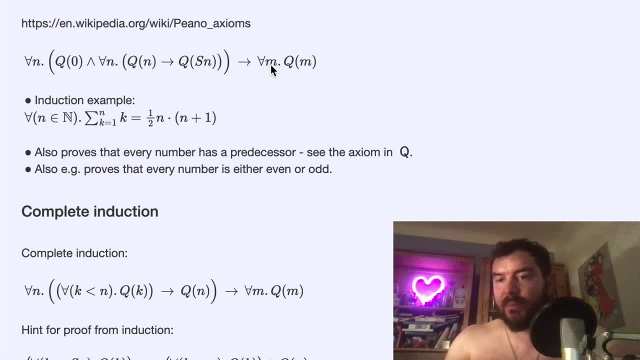 it turns out that they are. also, it's permissible in piano arithmetic to add infinite numbers which, um sort of, come beyond the initial segments, and we are going to see some pictures later. um, yeah, okay, so, um, you can prove then, for example, that this axiom that i manually added to robinson 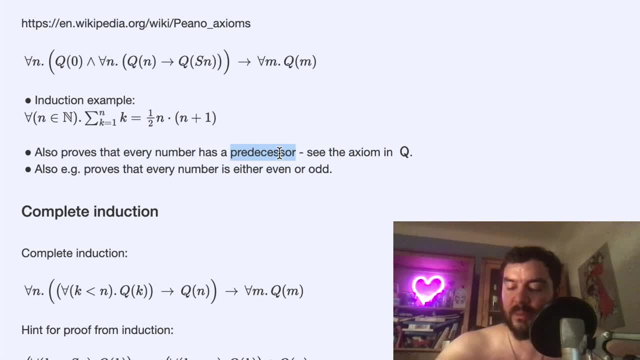 arithmetic that was manually part of robinson arithmetic, namely the statement that every number is either zero or has a predecessor, actually follows from uh in the induction axiom. for the sake of simplicity i will not prove that, but i will prove some other thing which are is also interesting with induction and um, necessary then to understand the non-standard model. 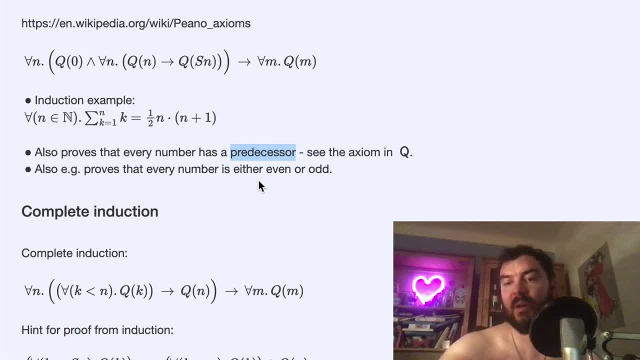 um, i want to point out it also proves that every number is either even or odd. right, you can- i mean you can- think about how will will the proof go right? you validate it for for zero and then you make the induction step. it cannot be that hard to prove that every number is even or odd, like every. 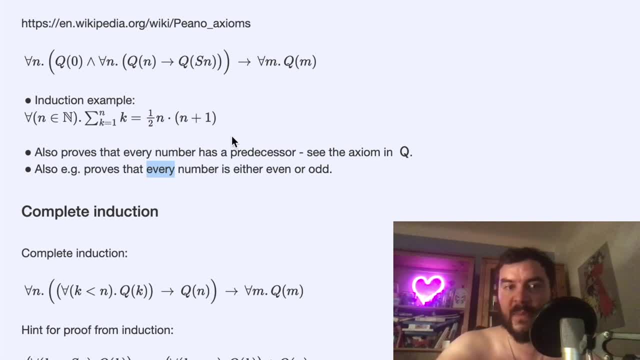 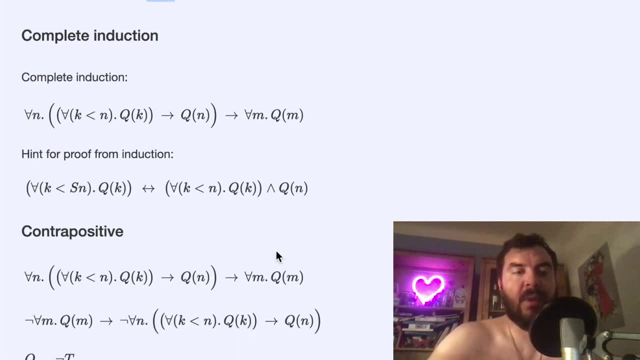 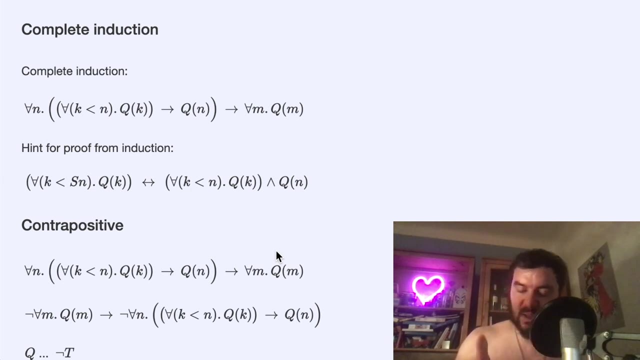 every. this is this area- is of course this, you know, the quantifier, and that is. this is then the former statement which the induction axiom gives you. okay, um, so uh, to understand the relationship between minimal element and induction in piano arithmetic as well, this proof is exactly the same than for set theory in transfer. 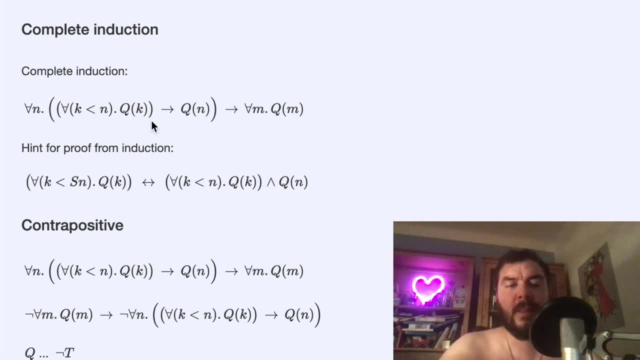 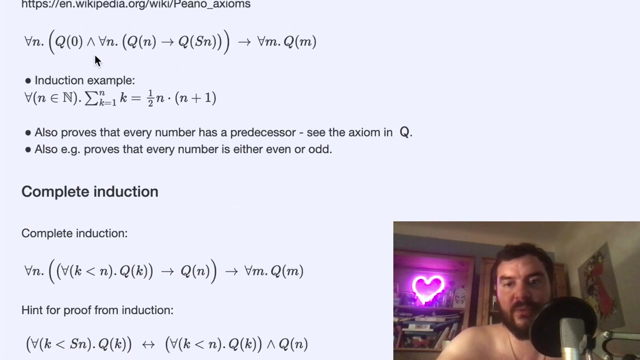 finite induction and regularity. um we sorry, you know, when i talk for an hour then my, my nose is like tickling. um so, uh, there's another form of induction, called the complete induction, which on the nose has a like a harder requirement. you know, it looks exactly like induction before, but uh, 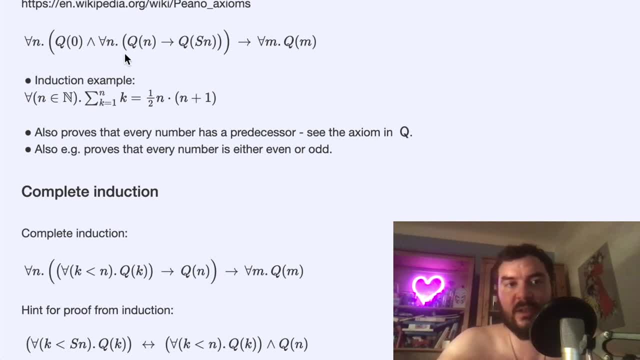 similar, except the zero is not explicit and the successor operation does not appear, but instead the. in our definitions, the derived relationship of uh smaller than appears here. so again, this zero and and and success operation. these were the primitives in the way that i pulled up uh, the arithmetic theory, and i defined the smaller than relationship in terms of them. 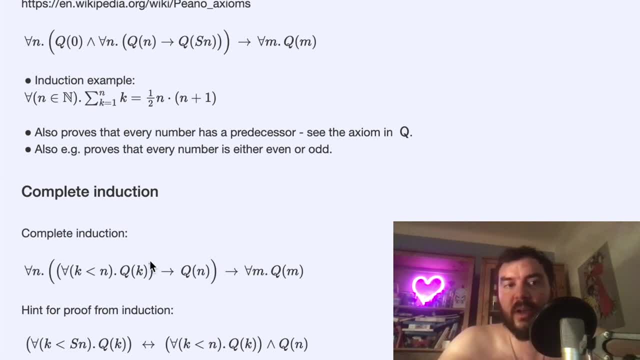 and then there is now an induction statement which we can prove from the original standard induction statement, which does not use this symbols, but instead uses that symbol right, the relationship symbol. and this is also then, theory is not in like in defined in terms of some constants and some some operations, but in terms of 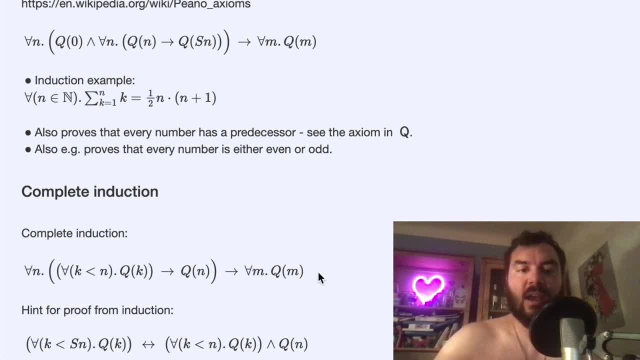 a relationship, namely the membership relationship. this is also, then, the axiom that is then relevant for set theory, the transfinance induction, or set induction actually, which proves transfinance induction, and, in fact, the set theory? analog is basically exactly the same statement, except the relation is not smaller than, but membership. okay, um, i will not prove it, but this is equivalent. 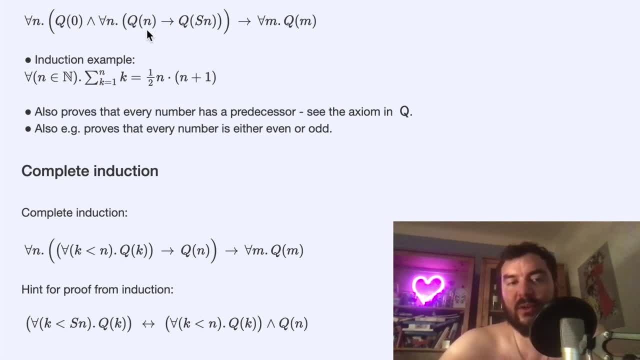 to this induction, even if that uh looks, you know, easier to, um, i mean, depending on how you see it, uh easier to work with. you know, here you just do a one step. here you might have to prove, um, i mean you might, you can assume more. i mean there's pros and cons and you can go. 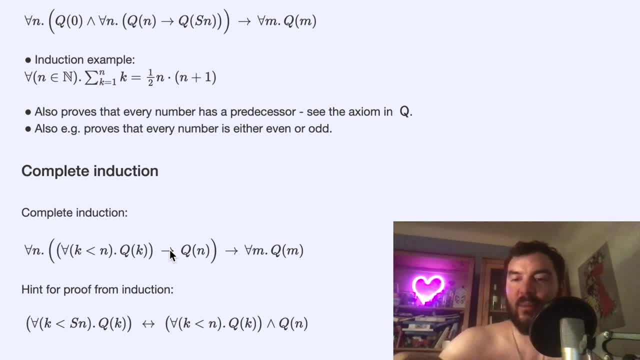 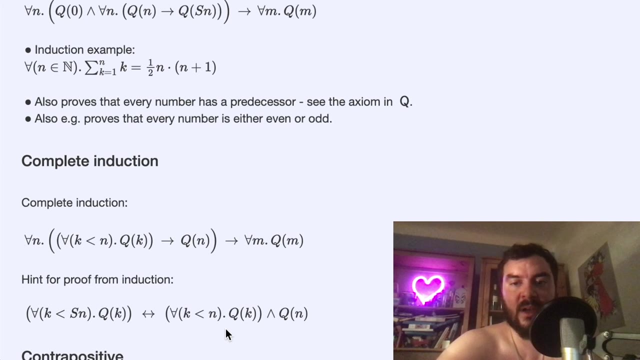 to wikipedia. you can go to wikipedia. you can go to wikipedia. you see different scenarios where this and that form of induction is easier to use. But these are actually derived from each other in some small steps and without going through everything. here's a small hint: If you look at the bottom formula and you see that, if 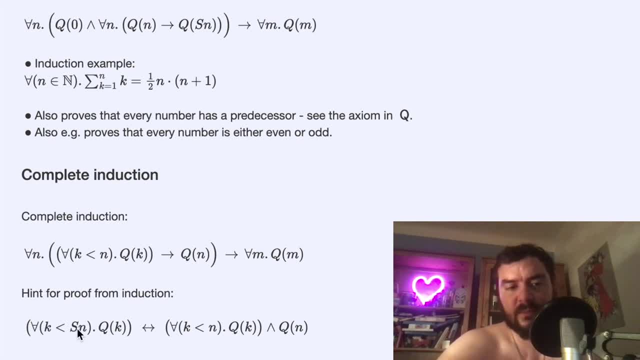 this formula, which has a successor in it in the universal quantifier. you can actually see, then, that if this holds, then obviously q is true for all numbers smaller than n, but also for n itself. The universal quantifier becomes a universal quantifier without the s, but with an exact. 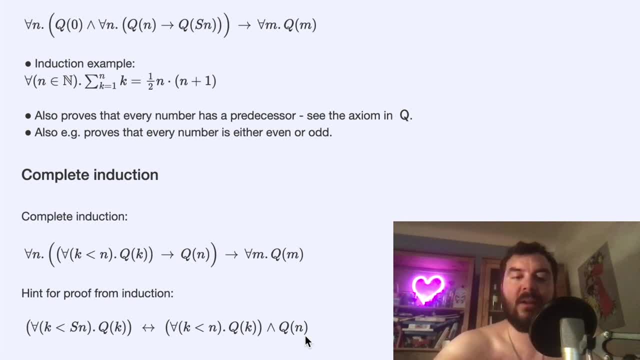 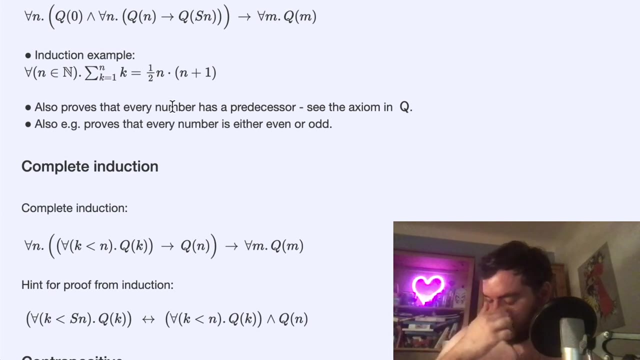 conjunction. You can quickly think about why that makes sense and then you can use this and prove this form of induction from this form of induction. You can do that as a homework exercise. So I'm just highlighting that there are the same quotes and quotes derived from each other, and this is the form which is relevant. 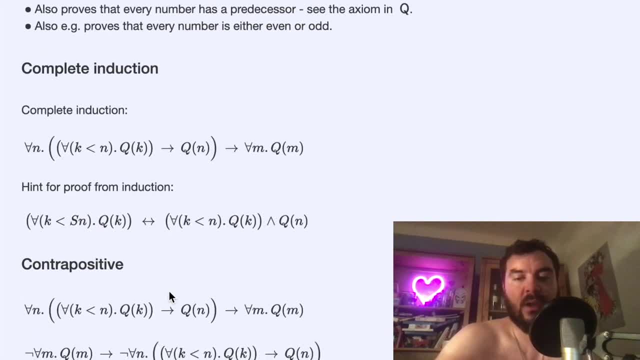 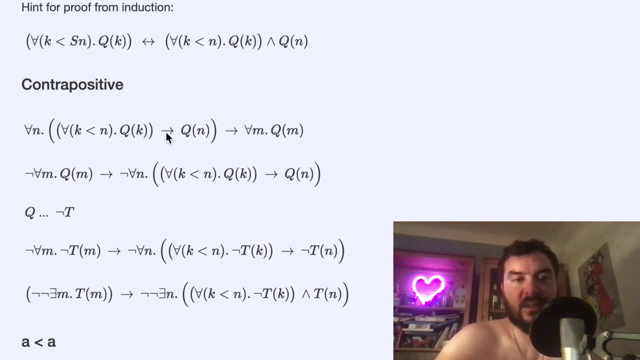 for set theory and also for the minimal statement that we are going to discuss in the final section here. So sorry, okay, this is again the induction statement. I'm going to take the contrapositive right. I've written down the formulas that I'm going to use. this is this, here and now what? 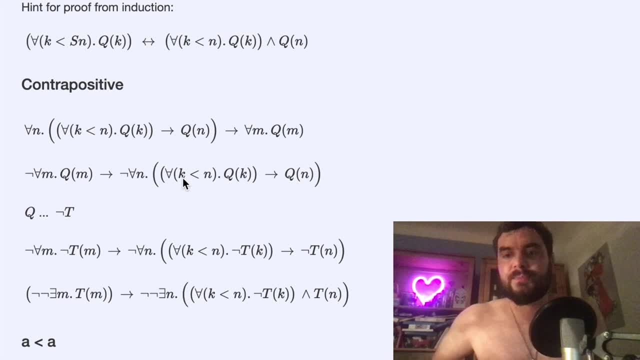 it means If I'm in the proof of the equivalence- classical equivalence at least- is I'm going to look at particular cues which are of negated form- If I'm in a classical context, then negating twice brings me back, and so nothing is lost there In any case. 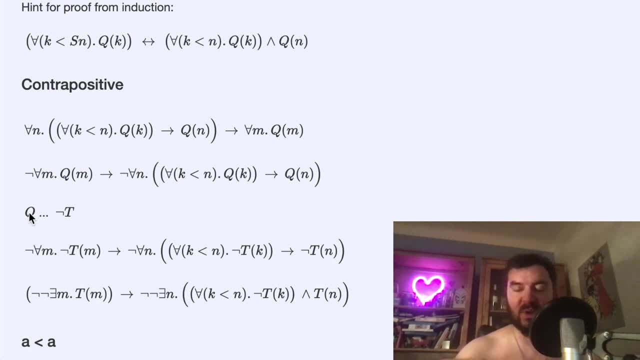 here I'm looking at particular predicates, namely the form of a negated form. So what I mean is, classically, you know, I can say I'm born in Vienna and it's the same. classically, I'm not knowing what the following case is. a thing: I'm not not born in Vienna and so there's nothing lost in considering. 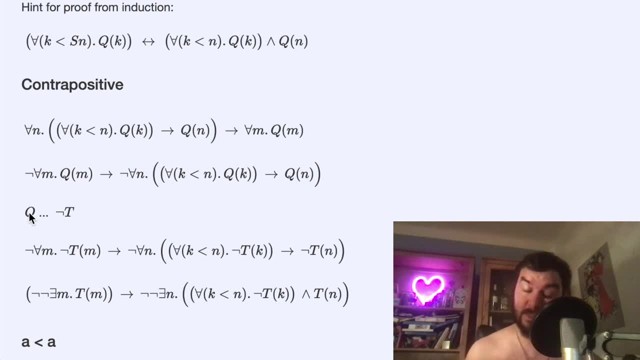 only predicates which are of negated form classically speaking, and so I in any case again- you know I'm trying to hurry, to not go over time too much, but here we're going to consider this negative predicates, and then the same statement just reads like: so we can use then again the relation between 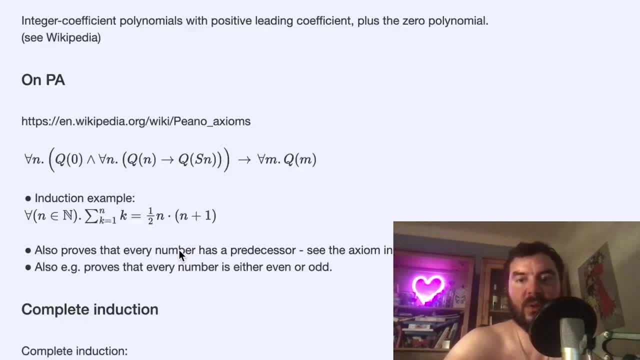 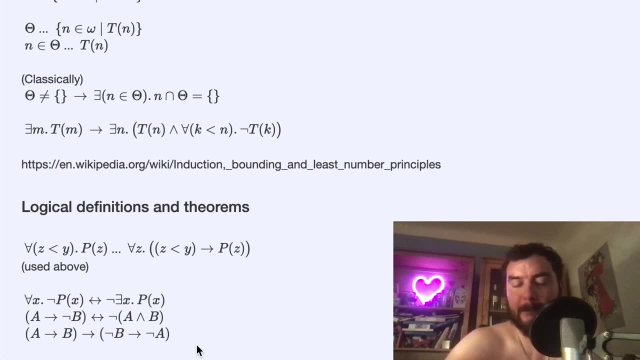 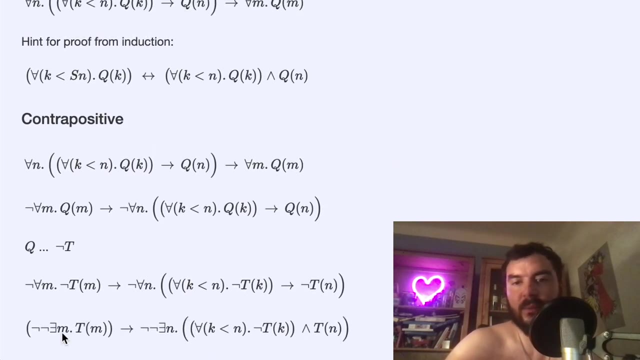 implication and conjunction. this you know. I show it quickly to you the rules that I'm applying, which are constructively valid here, these are rules right to rewrite the thing as such, and and then, finally, what we get is this sort of statement: and this is exactly the least number principle, bar the. 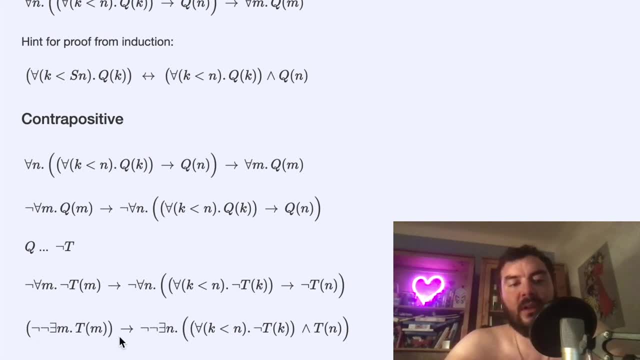 double negation here in in the assumption. it's actually good that you're constructively speaking. it's good that here there are double negations, because to assume existence is a strong assumption, right? so this, this thing, is a weaker assumption than just then actually assuming existence. so if then an M exists which has T, then this: 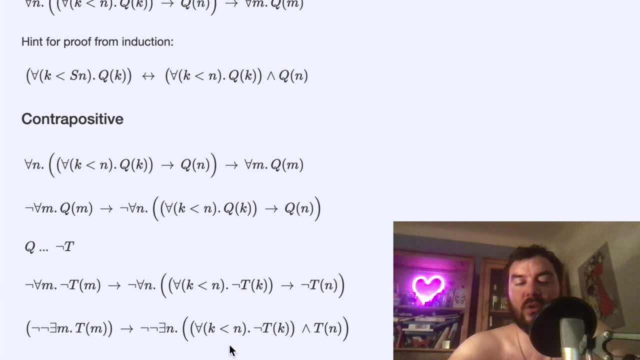 certainly is true, but the implication also holds if there just does not not exist and an M, and the implication is also double negated. again, if classically you can remove the double negations constructively, sorry- if T is decidable, then- and you know a number exists and you can also. 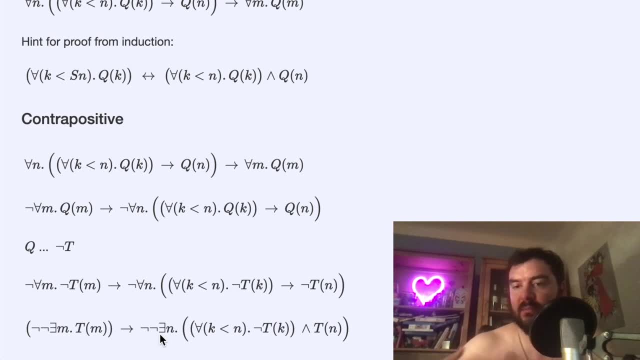 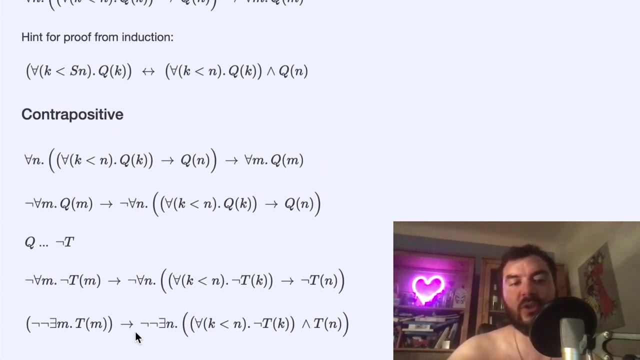 look at for all numbers beneath M and you can check if there is a minimal element. also, you can either adopt Markov's principle which says that double negation elimination holds for decidable statements. just comment for the type theories among you also. okay, so we have established this from the complete induction and which is the 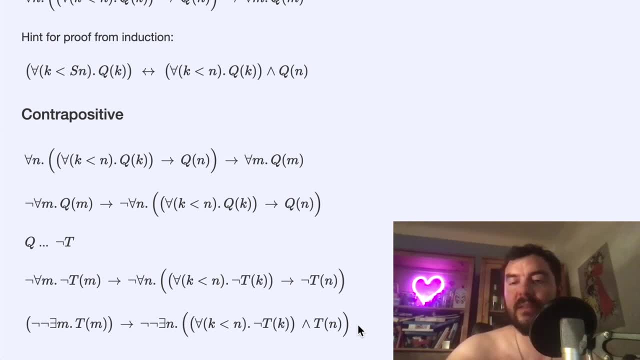 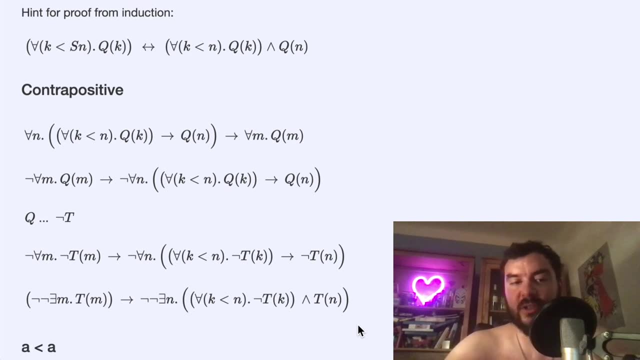 minimal, the least number principle, or minimal number principle, and now the least number principle, and now the minimum number principle, and now now the least number principle, and now the least number principle, and now the. now i'm going to look at the implications for this sort of relation. right, what we are going? 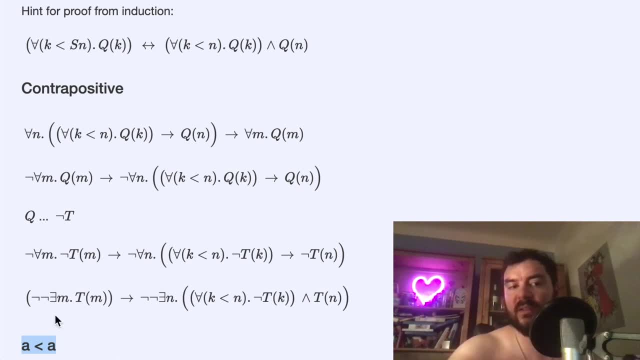 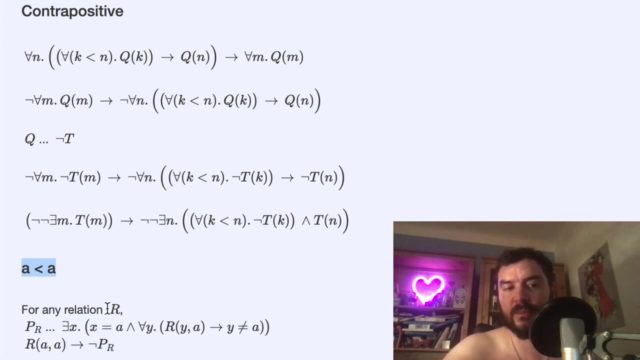 to see in a second is that this um, the statement here, which stems from reduction, so which holds in piano arithmetic or hiding arithmetic, actually rules out that there are numbers with this property. and this goes as follows: so um, let's say of any relation, and define pr is another. 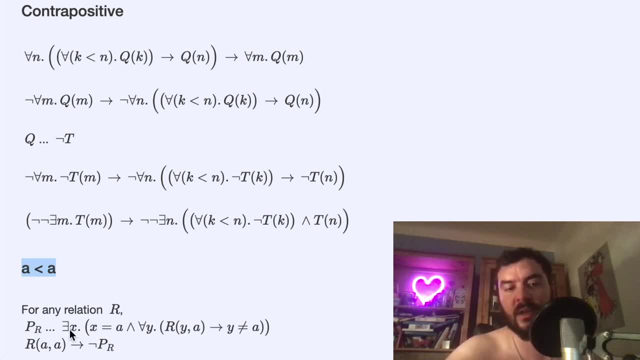 property as such. if the statement says there exists an x, exists x, which actually is a um, and that for all y. if r is a relation, uh, if y is in relation to a, then y is not a. this is basically. i'm mirroring, i'm just abstracting from from the expression here. then this thing, um. 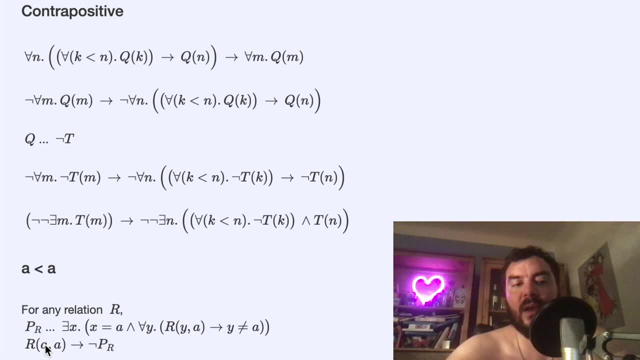 has the following implication: if if a is in relation with itself, then it means that this thing does not hold. when you can play this through, let's say a um is in relation with itself and there exists some number which has this property. well, this number is then a um. and if for all y? 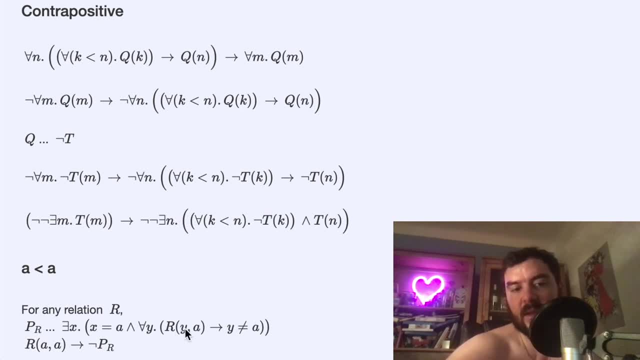 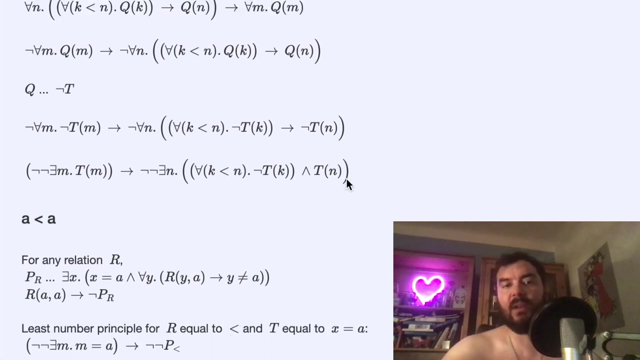 uh, this expression holds, then it also holds for y equals a, and then you have a is not a right, so contradiction: um. so that means um. if that thing holds, then if r is in relation to itself, this is contradictory right. and so um, if the least number principle holds. 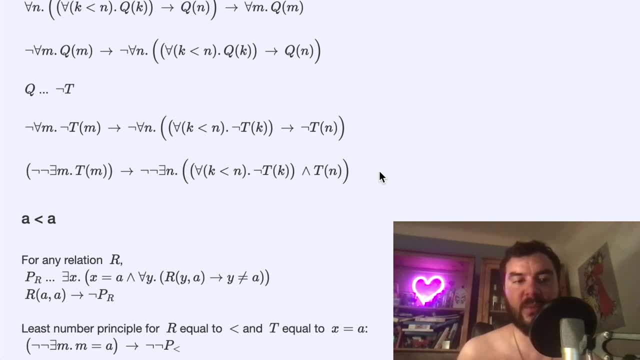 which, which holds by assumption of induction. um, then the existence of an a, or we called it c, a, c, which is smaller than itself, is actually contradictory, right? so, um, if, uh, again, let's play it through, let's say a, c, we assume that a c exists, which. 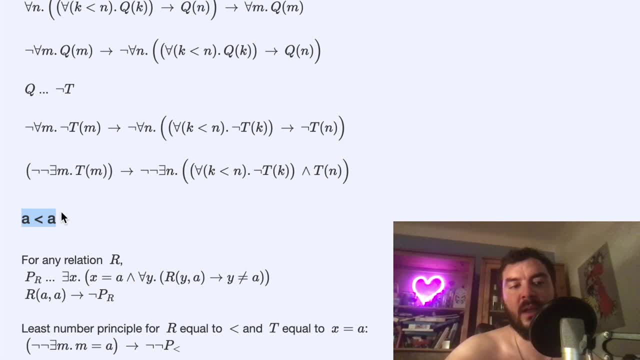 is smaller than itself. okay, then, um. use the um for t. we are going to use um. x equals to c, right? so the, the property that we are going to look at is that x equals c. then, uh, the assumption of um, the least number principle, holds right. because there, there. 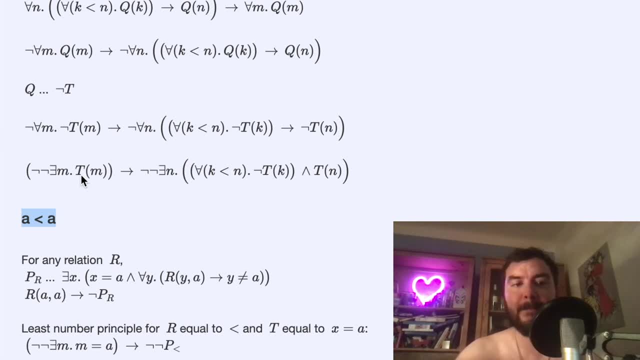 exists an, a number which is equal to c, um and also um. we we know that this thing, like by this argument, is Listening. well, its a plus or minus. maybe i'm just out of my mind that x is equal to one, so which? that is usually right to say literally. 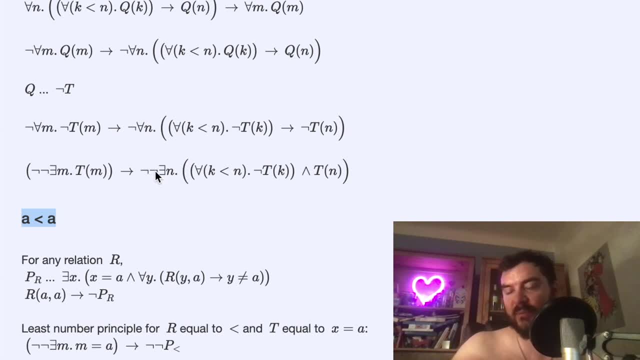 yes, because. and then if if c follows Block C, all the values of N ó equals b, if c follows Block C, all the values of Nrese Multi, and then, as always, it's uh, almost as though um that you can also say another це. you can say like this: criticizing, comparatively right. so 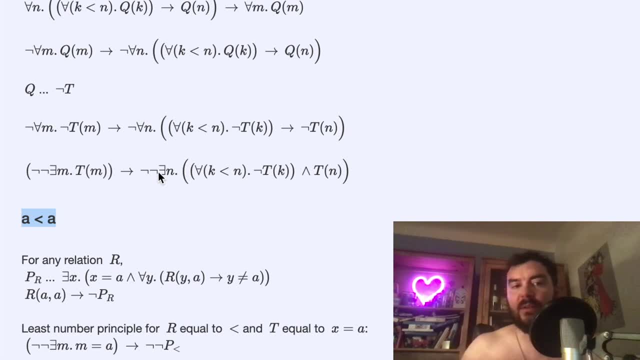 If you are more interested in it, then just play it through yourself, right? Make the assignment like. write down a list of assumptions. Like we exist, we assume that this least number principle holds. We assume that there is a, C which has a property that is smaller than itself. 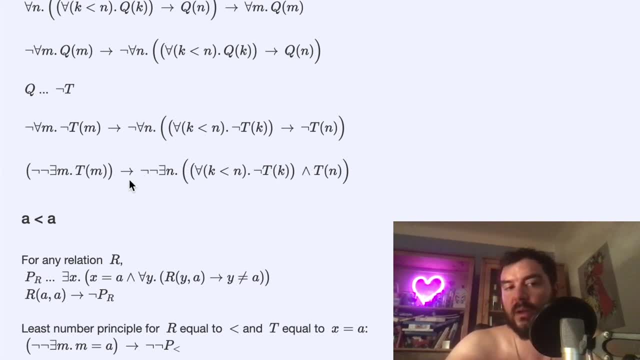 And what does it mean? if you look at this implication and you, if you take everything apart and you take into account that the number C is smaller than itself, so that both T holds and not T holds where T is this equality relation, then there's just too many things that are true and you get a contradiction. 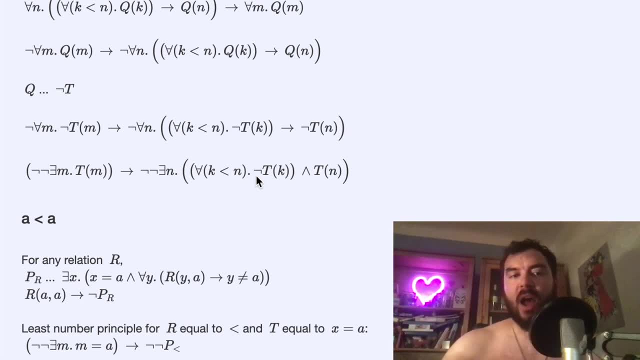 Okay, I hope that makes sense. So this: this shows how induction um in the form of the least number principle actually rules out that the number is smaller than itself. right? So in, in. in piano arithmetic no number is smaller than itself and the 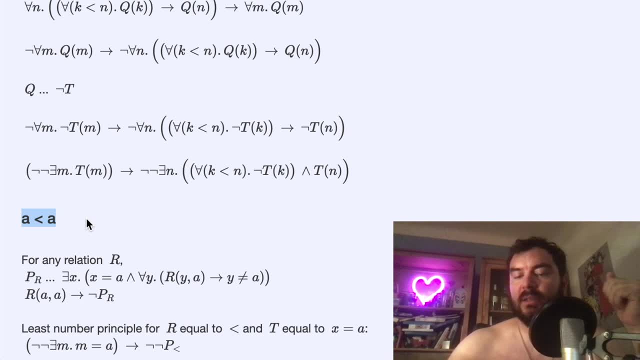 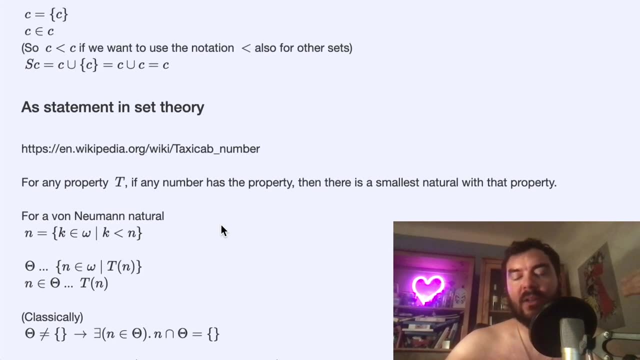 C element. um is not a legal model And um I like, if you look at the set theoretical analogy where um you imposed the set induction, which you know, it's like transfer induction, or if you directly impose regularity which corresponds to the least number. 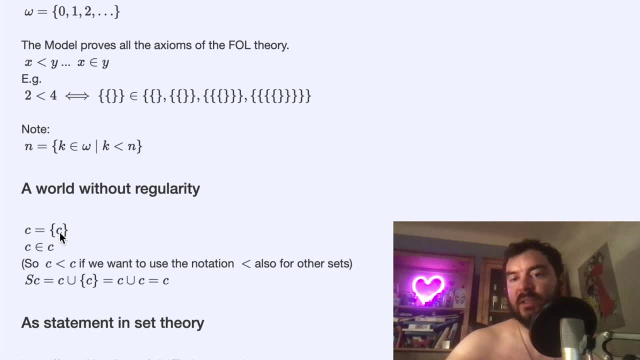 principle, then it rules out this: uh, objects which contain themselves exactly with the same proof, Like you? Okay, So you can play everything through the. you have this general relation. in this case it's not smaller than the natural numbers, but this membership, and then 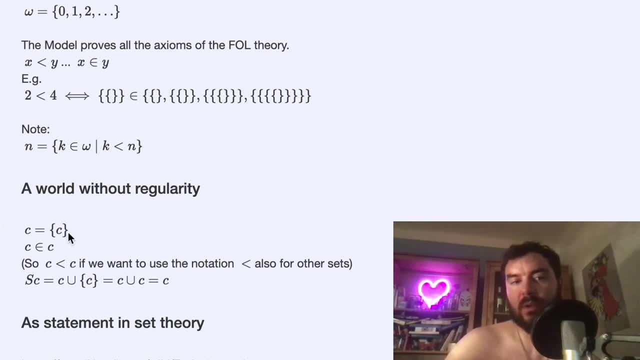 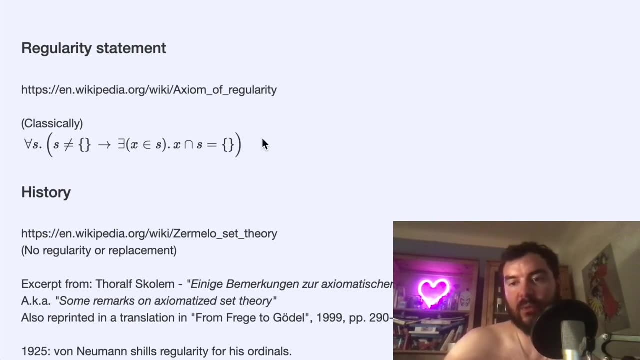 by adopting these axioms, you rule out this possibility as a model and indeed you know, I mean you can go on the Wikipedia page and prove that the singleton which contains itself is ruled out by the axiom of regularity, like in a two liner right. 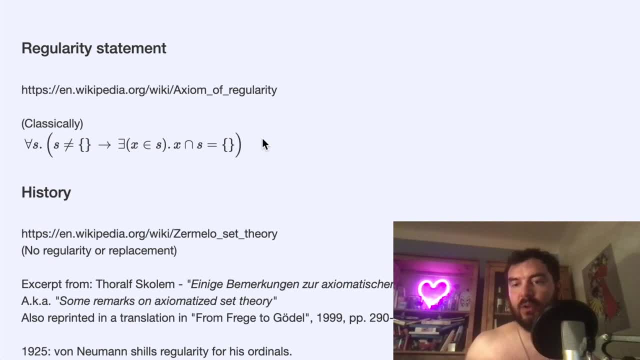 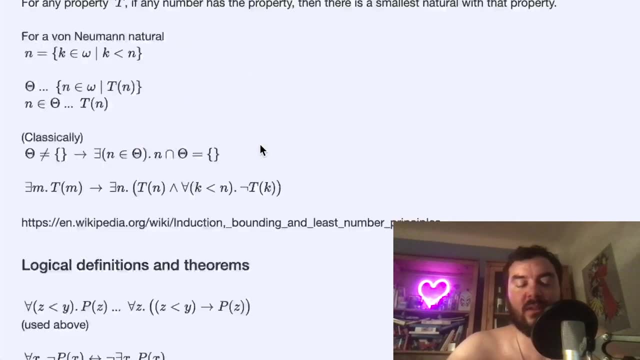 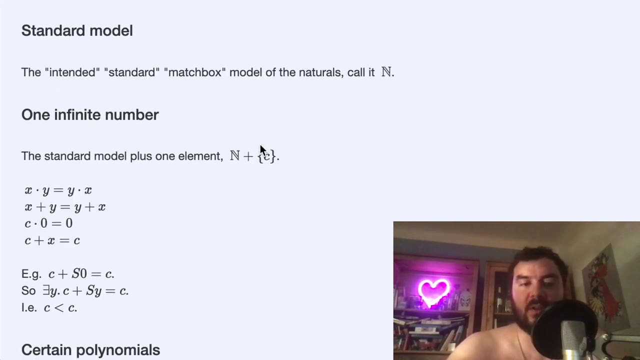 I have, I like, um cooked up a much more broader um context for this sort of um proofs of non-existence of um self-relation. but this is how, how things happen, right, How? how? um models of theory are ruled out by adopting this induction axiom, by 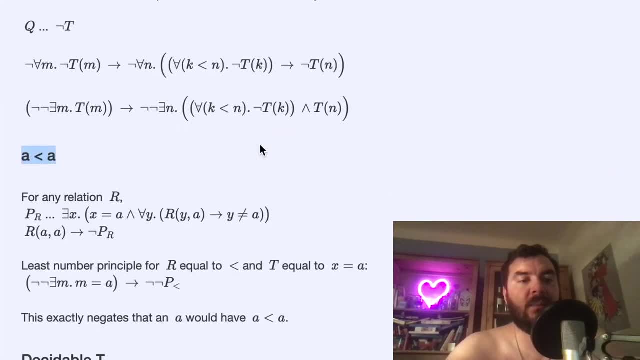 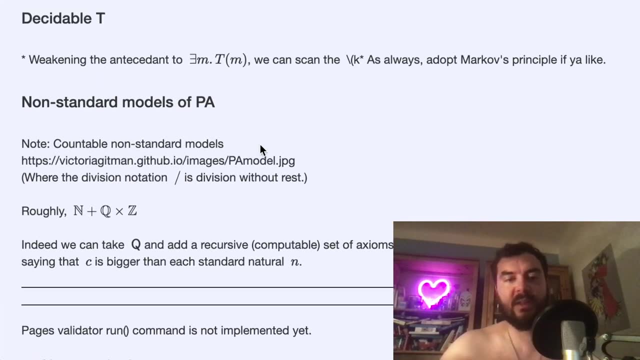 certain structures are ruled out. Okay, Um and Okay. I've already noted that, And and so, finally, in the last minutes, I want to uh emphasize that also. if you're in in, adopt induction, uh, it's still the case that. 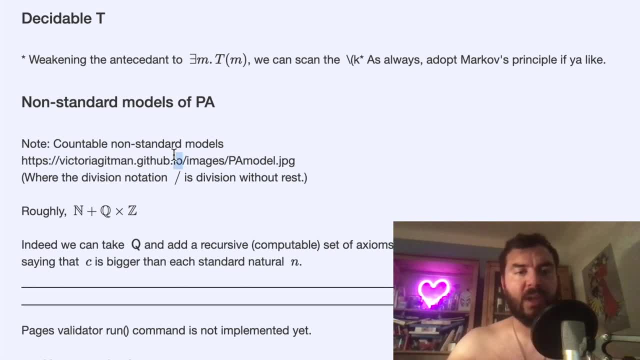 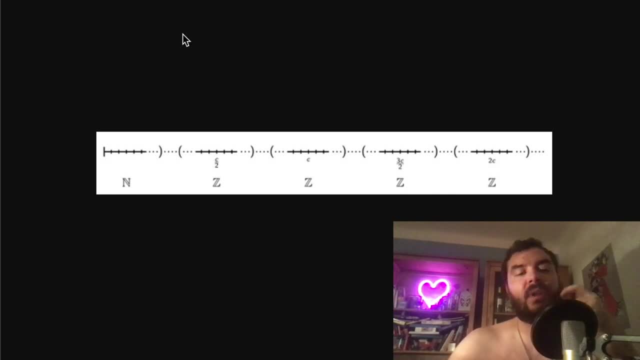 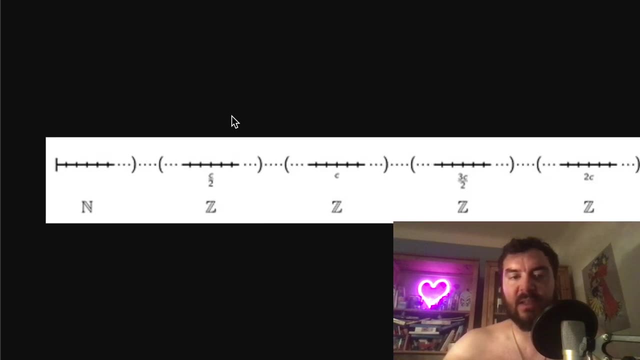 The theory will have non-standard models, And what happens is I have this here. So this is from a blog of, I think, a student of um set theorist Hamkins. Um, and yes, this picture, this is what? uh, one of the countable non-standard. 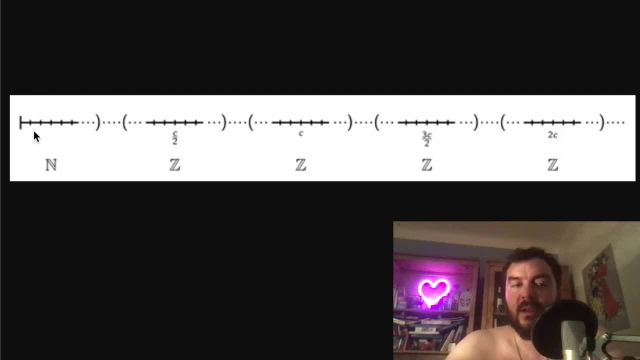 models of piano arithmetic still look like. So, um, you have to fear of paranoia. arithmetic: It has the induction axiom. It's like this: first order, It has the induction axiom, but um, it's still uh possible to find a model. 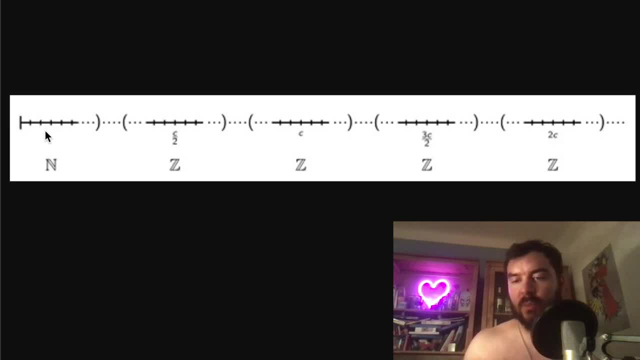 and you can encode it, for example, in set theory, which has more elements, Then just the natural numbers, for example, you might have encoded them as phenomenal numbers, this normal behaving numbers, right? So what happens here is this: you say I um, I assumed existence of an, um, element C. 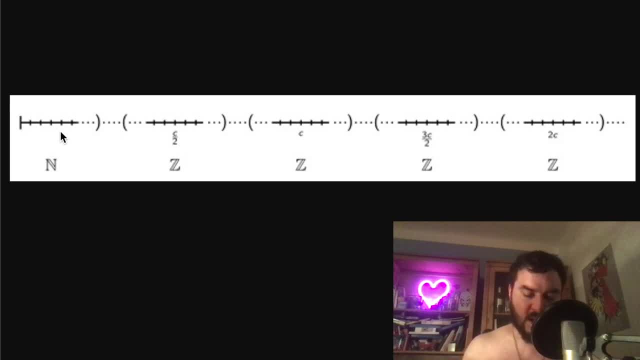 which is bigger than all the standard natural numbers. right, The first order theory can actually not talk um, um, like it cannot really distinguish with quantifiers, um, between the standard natural numbers and the numbers which come after, after the initial segment. but what you can do in the 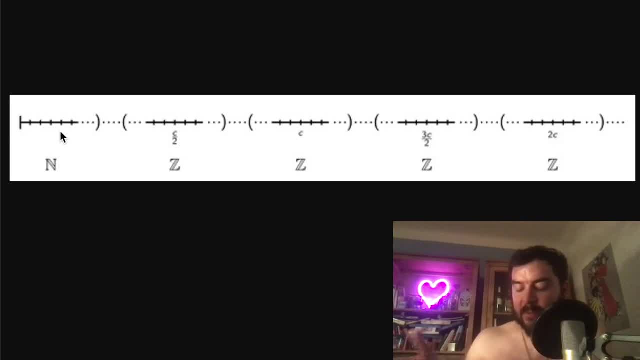 theory, like we do did already with the induction schema, is: you add an uh, infinite amount, contemplate infinite amount of similar looking recursive axioms, and these axioms have the shape that you say: for every uh number: zero, the success of zero, the success of success of zero. 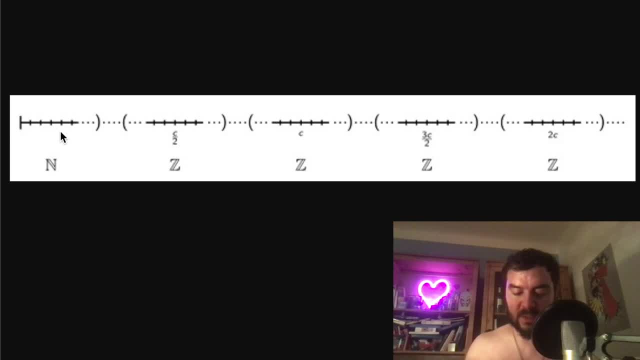 And so on. you add the axioms, that all the statements, the individual statements, that these are all smaller than C, and what you get then is that there's the natural numbers, um, with all numbers that you are familiar with, so to speak. 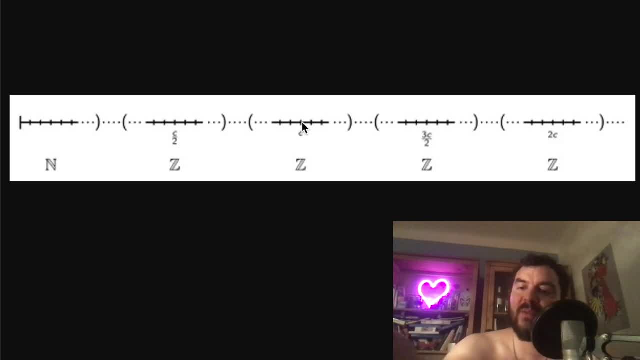 And then there's a C, and but we, you know, we, we prove by induction that no number is smaller than itself. So This C does not have the property that is smaller than itself. However, um, it is legal that it is there. 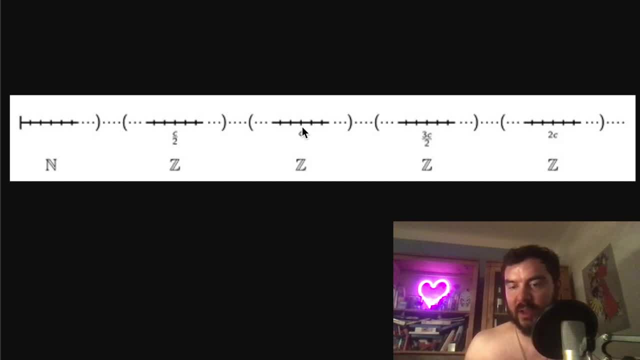 And the, the induction axiom and the other rules, the other axioms of our theory now imply that there are even more elements. So for example, for um uh, for taking C, we can form the successor and the success of that and the success of that, and these numbers must all be different. 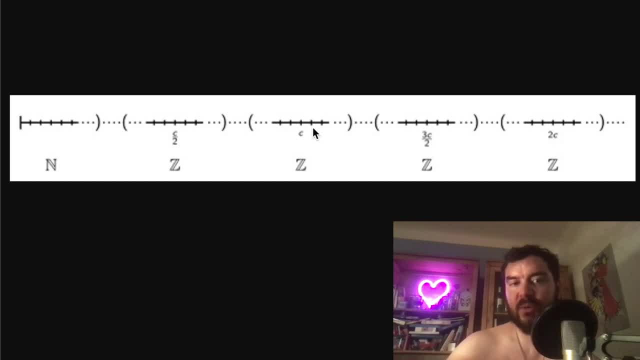 So, starting from C, There is a structure which looks exactly again like the natural numbers, but it doesn't start at zero, but it starts at C right. Zero is a special number in the natural numbers by the axioms right. 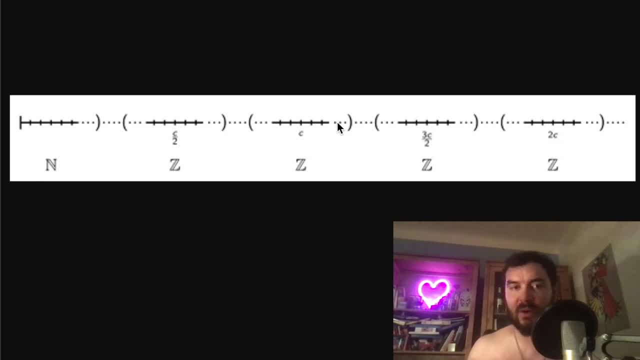 Everything times zero is it's again zero, and so on and so forth. So zero is still here, but C is here and there starts another um sequence of numbers which again are sort of like like the natural numbers in the sense. 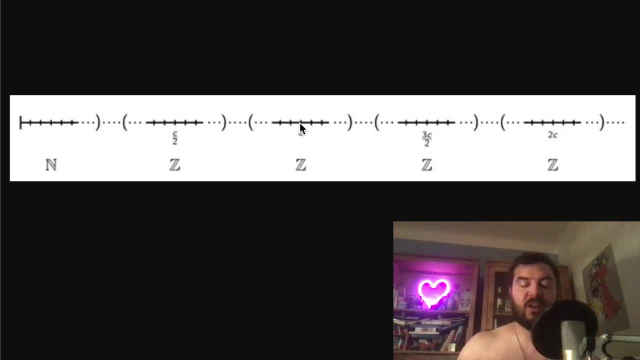 that they start somewhere and go where. but we've also proven- Or we have not actually proven in this video, but it's also provable from induction- that every number has a predecessor or or zero right. Okay, The stereo is here. 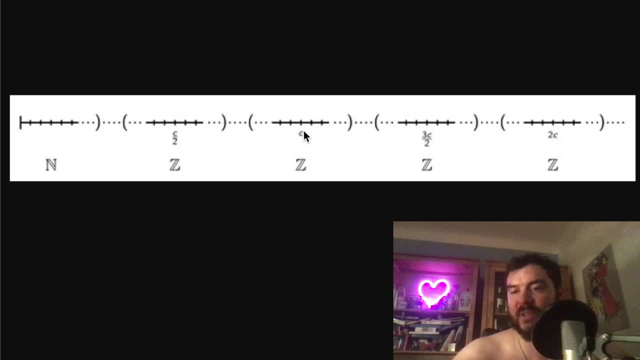 It doesn't have a presence predecessor. but here C is different from zero. So that must mean by the statement that every non-zero number as a predecessor, there's a presence predecessor, And that's why the numbers go backwards from here, right. 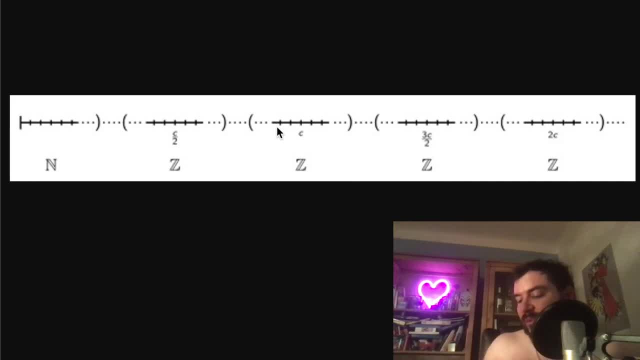 It says: Oh, you know, there must be one number which is free before C, And so this number three before C exists as well. And this is it's still not contradictory. You just say there is more numbers And um, then what also happens is: um, you can do division. 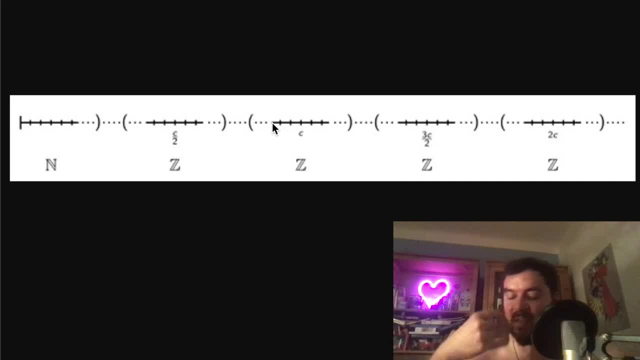 without rest uh in in the naturals right. So an even number you can divide by two, and an uneven number divided by two like minus one divided by two. And so what sadly, so to speak, happens is you get a bunch of uh like fractions. 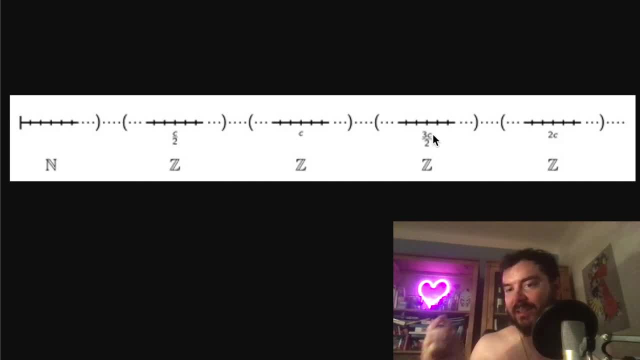 times C and these behave again like like This: two sided natural numbers, right? So this whole thing is basically the natural numbers plus and then for every rational number, like for example three over two, another block which looks like the integers because it goes back and forward from this number, right? 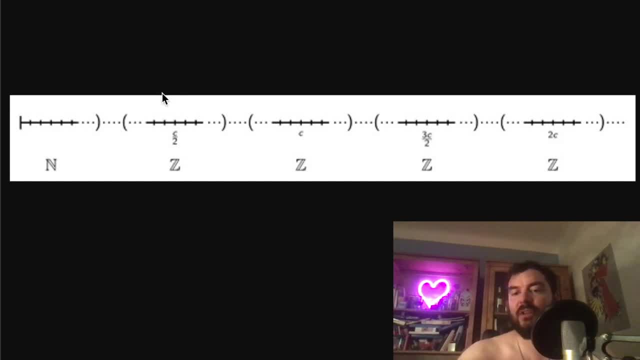 And it's funny, but this sort of construction, um, still fulfills all the axioms of arithmetic, right? You might believe that it fulfills the simple, Okay, Okay, You might believe that it fulfills the simple axioms that are also. 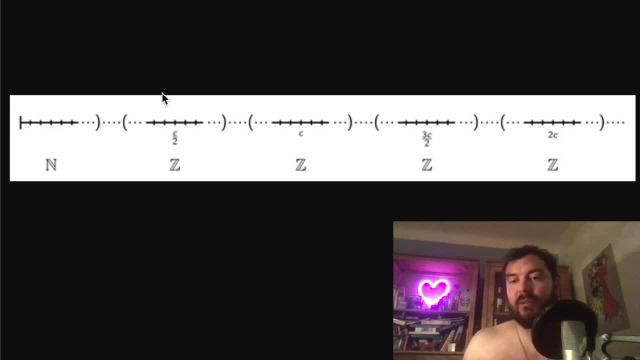 part of Robinson arithmetic. but it also- and this is like difficult, more difficult to discuss, um, because it goes in the questions of consistency- It also fulfills the induction axiom and says: basically, the induction axiom now says that if something is true for zero, and it's if it's true for any. 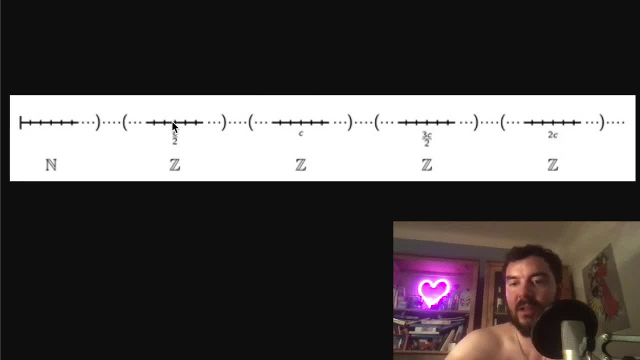 number. it's also true for the successor number, right for for this, this, for this or this. then the property actually holds for all numbers. So it's fascinating to think about how Arithmetic it does not really know what it's talking about, right. 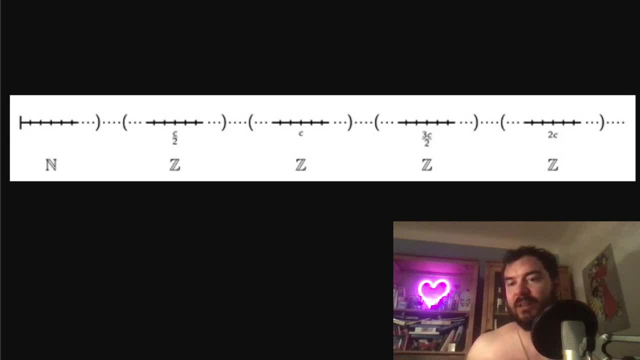 Of course we have the standard model in mind, but there are other models, And if you write down for all numbers, then piano arithmetic does not know that. there's no, no sense in which there's just the initial segment of natural numbers that you're used to. 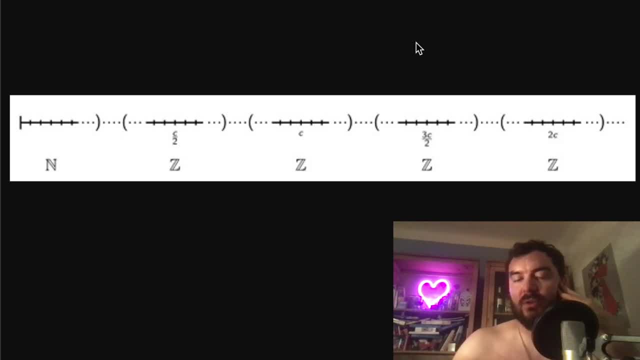 If you have the first order theory of arithmetic, then you could also as well be talking about this sort of numbers, with infinite jumps, so to speak. um, if a theory has, uh, just one model, we call it categorical, and more is to be said about that.